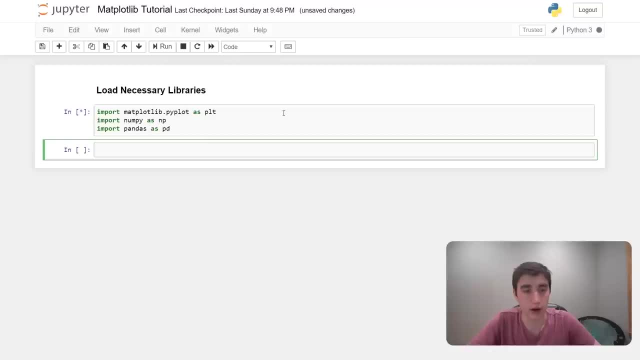 examples: import pandas as pd and run that, and so if you have all these uh like already installed, you won't get any errors. if you do get these get an error when you're trying to run them on the these, you probably need to install it. so you can either do a pip install, matplotlib, pip install. 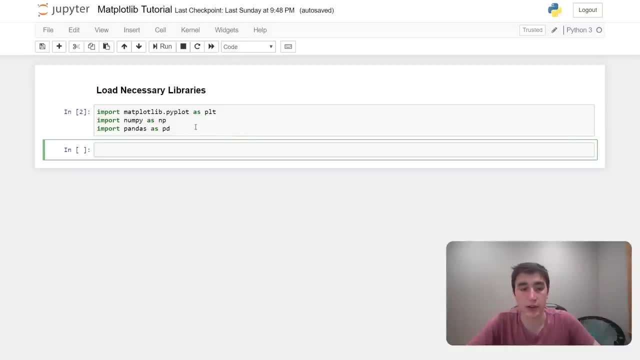 numpy pip, install pandas, or you can install a python distribution that already has these packages, such as anaconda. i'll link to how to do this in the description. okay, so now we have our libraries loaded. let's now build our basic graph. so i always think it's kind of the hardest. 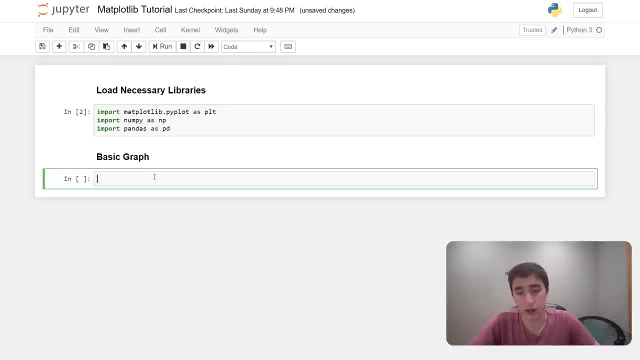 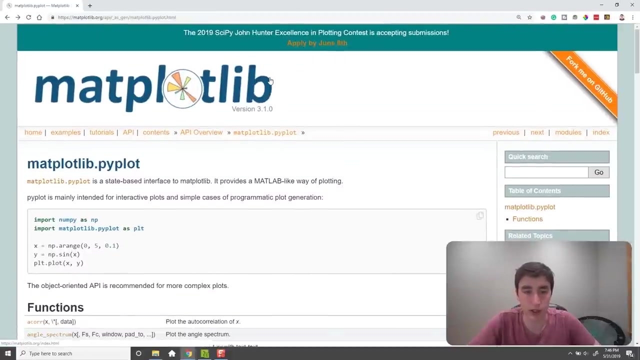 part about anything with python in general is starting with that blank, blank space. so what i recommend for matplotlib is always start at the documentation. so i have a link for this in the description, but here is the home page of the matplotlibpiplot documentation and what i 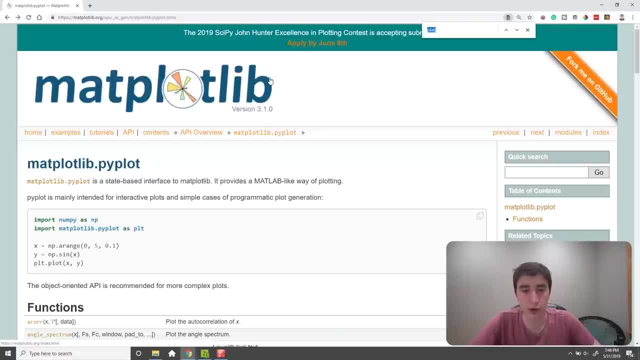 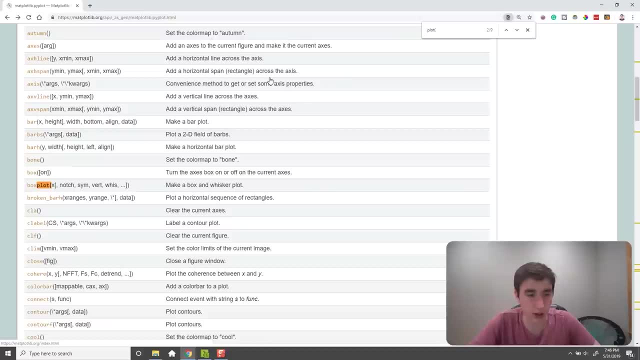 recommend is like whenever we're trying to do something new, just do a control f and like: look for it. so if we look for plot here, that's like we're just trying to get a line graph on the on the screen. uh, box plots not we want, we don't want it. then plot: okay, this looks good. 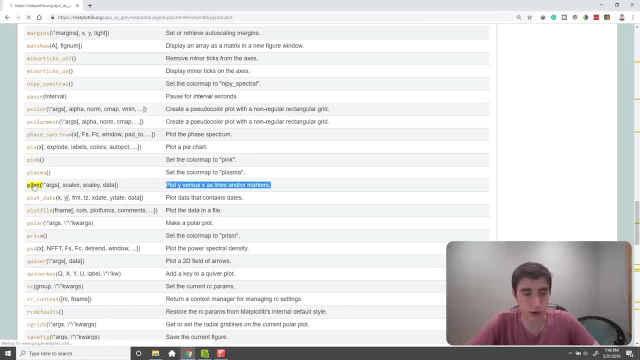 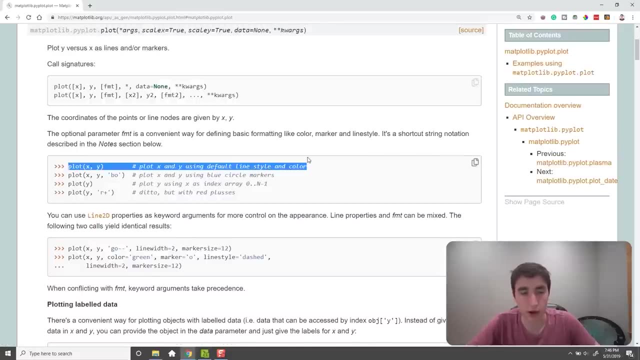 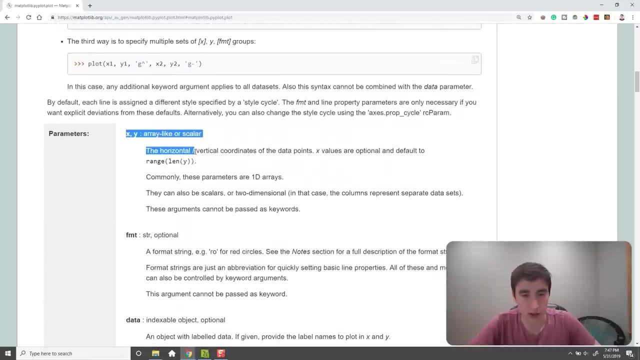 plot y versus x as lines or markers. so this is what we'll start off by doing. as you can see right here in the examples it gives: gives plot x, comma y. so that's the command we'll have to run to make this work and just to know what x and y are. if we go down to parameters, they tell us that 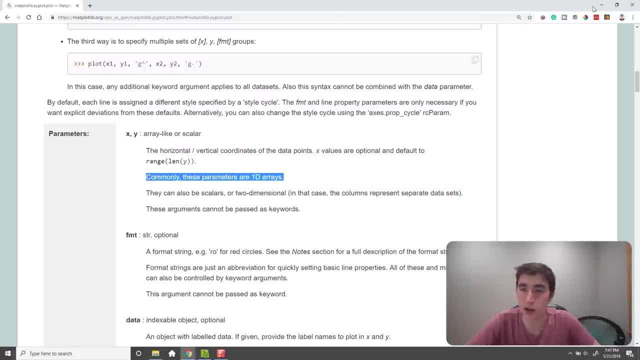 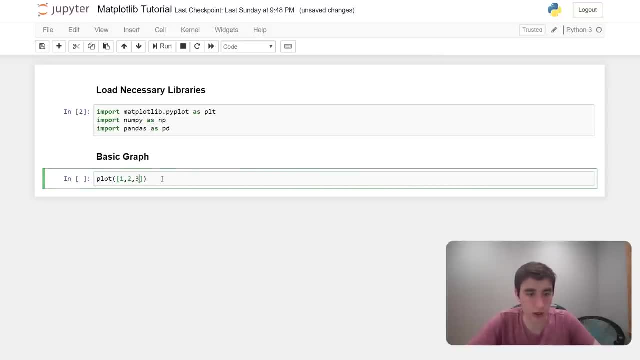 commonly these parameters are 1d arrays, so we know we need to pass in 1d array to the plot function. so if we do plot one, two, three, that's going to be our x, and uh, two, four, six will be our y. i can't. 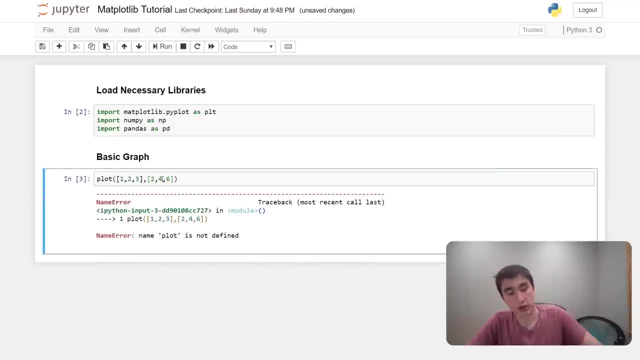 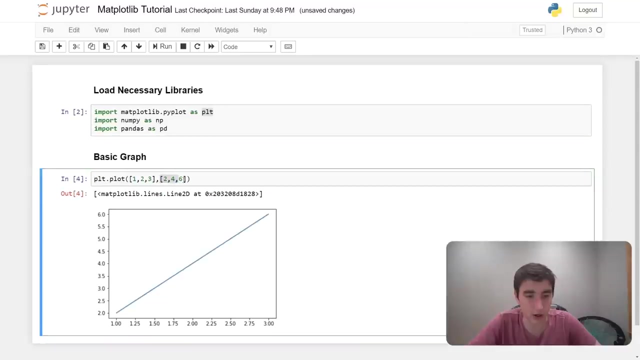 type and run that ah plot is not defined, so we imported pi plot as plot. so when we run this function we actually have to do plt, dot plot, and then this is our x and the second array is our y. so let's see what happens there. yay, we get a graph, and to clean this up a little bit, i recommend: 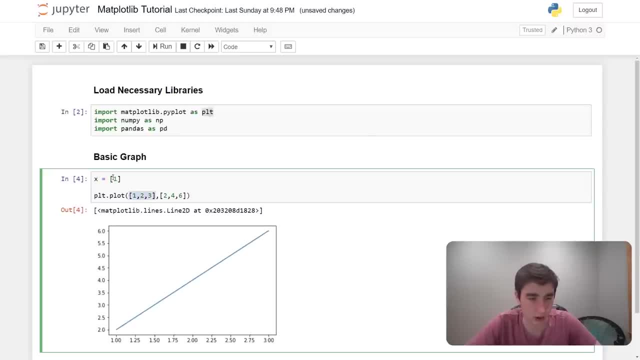 moving our variables into or moving our arrays into variables. so x is 1, 2, 3 and y is 2, 4, 6, and we can change now this to x, y. and one thing that's annoying with the mplotlib if you're doing: 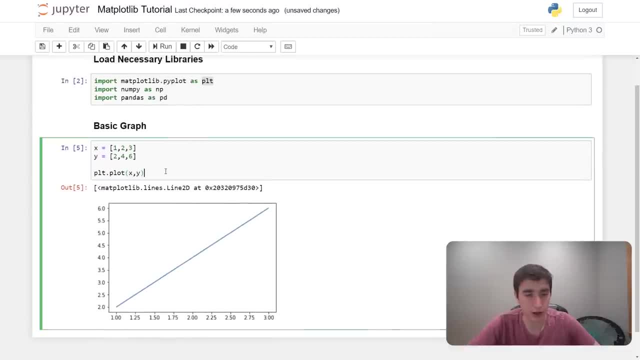 this in jupyter notebook by default is: you have this annoying little line here, so you want to get rid of that. you can just read it on your own. so if you want to do that, you can just type in the formula text and then you just type in the formula text and then you can get a graph and you can. 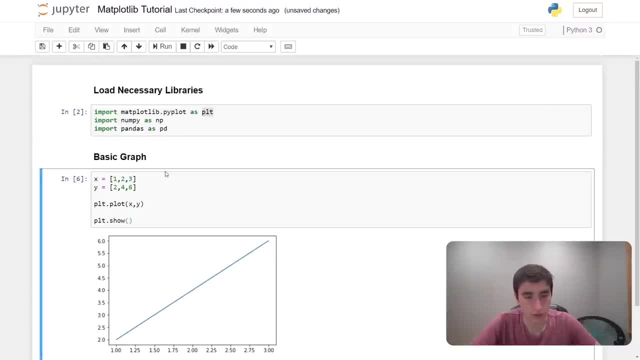 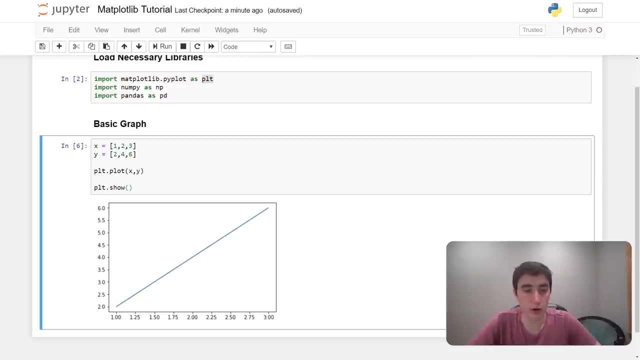 get a graph and you can get a graph and then you can come up with the function. you're going to get a actually call plot dot show, and that's the correct way to actually show this graph. okay, now that we have just a line on the screen, let's start adding a. 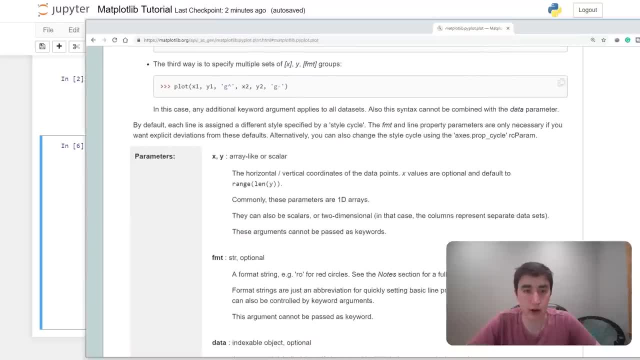 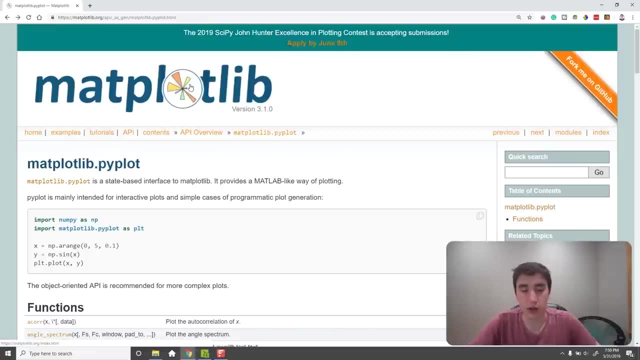 little bit more to our graph. so to do this, let's go back to our documentation and go back to just the pie plot. so I think this is a good spot to start, because you always can kind of just ctrl F and find something you're looking for. 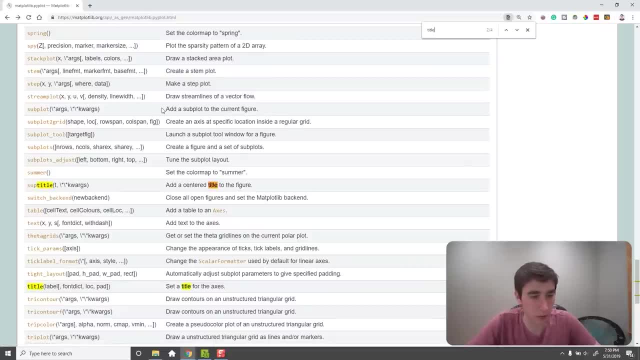 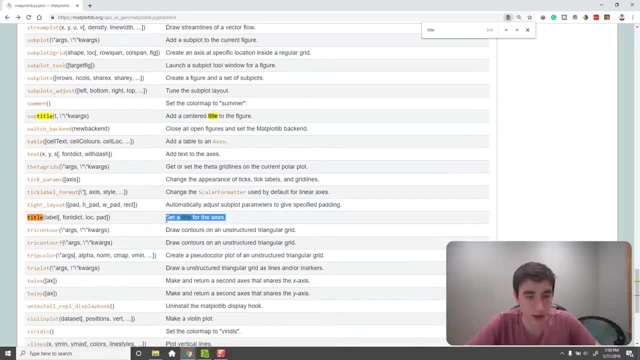 if I type in title, it points me right to a couple different places that I probably want to look at, and right here is what we're looking for. so set a title for the axes, click that, and this tells me all sorts of stuff about how I call. 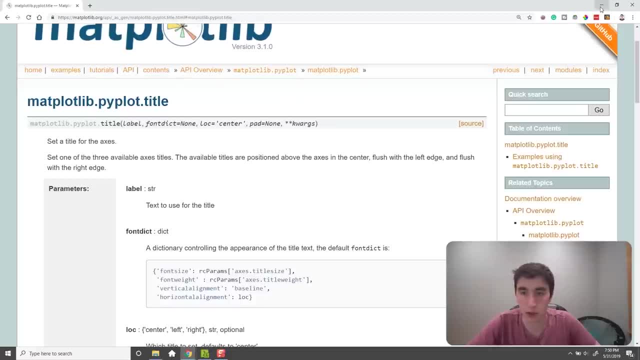 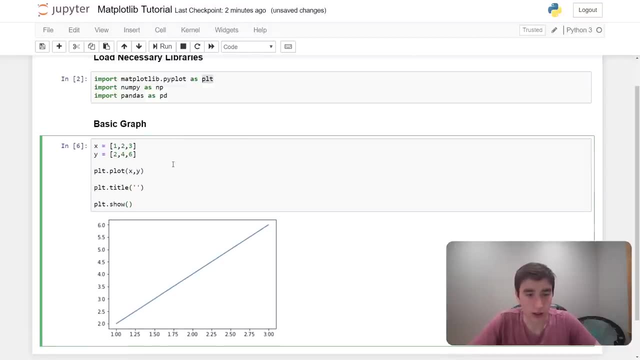 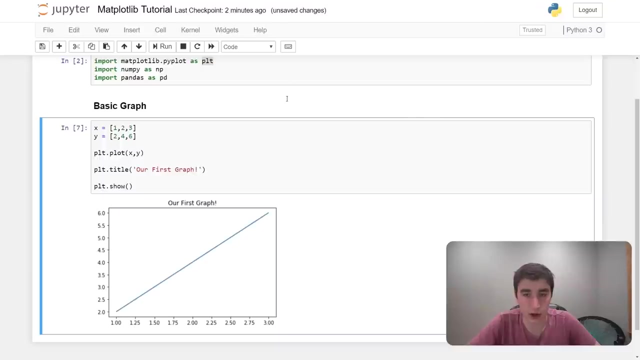 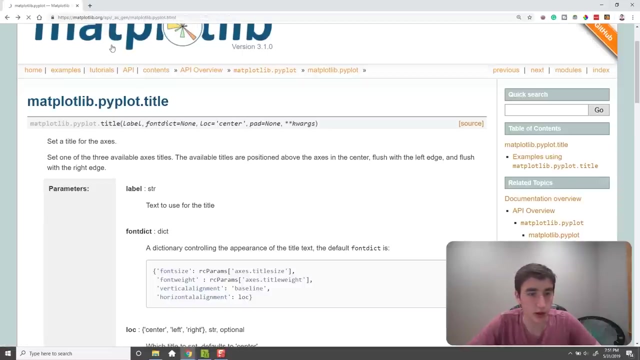 this. so it looks like I need to do pie plot title. so I can do plot title and let's just do our first graph and run that. as you can see, our title is now there, and same thing for a lot of the different parameters. so, going back to the documentation, if I want an X, 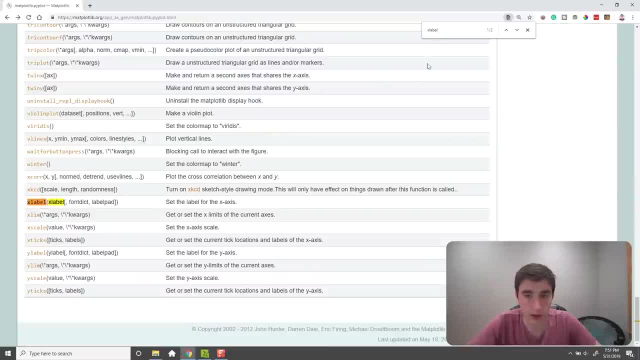 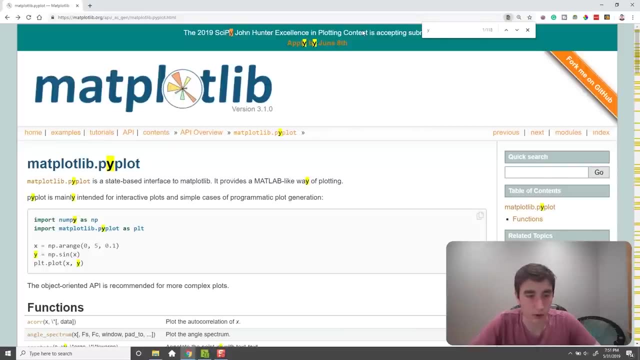 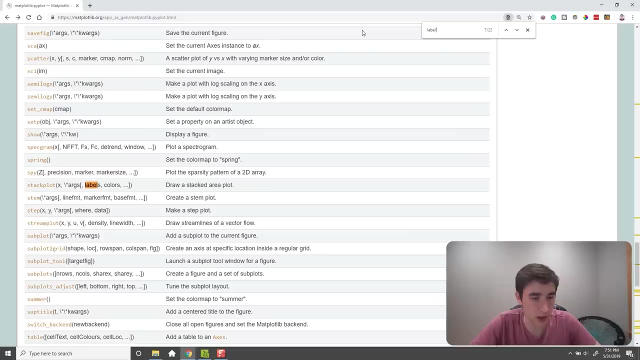 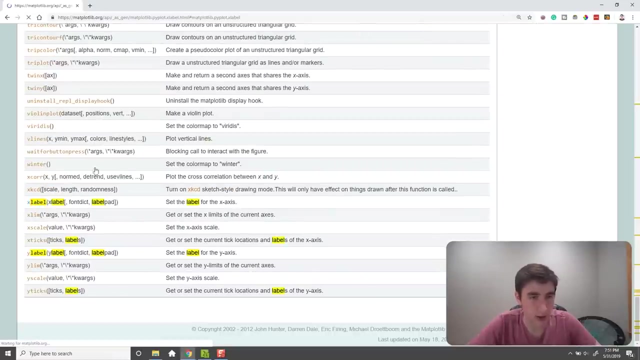 label on a Y label. I just type in: alright, I guess I knew that, but let's just say Y label, nothing comes up Y. or just even label C label label a contour plot. that's not us. the fig label is no, I know title no: X label, Y label. that's how we get there, so you can keep. 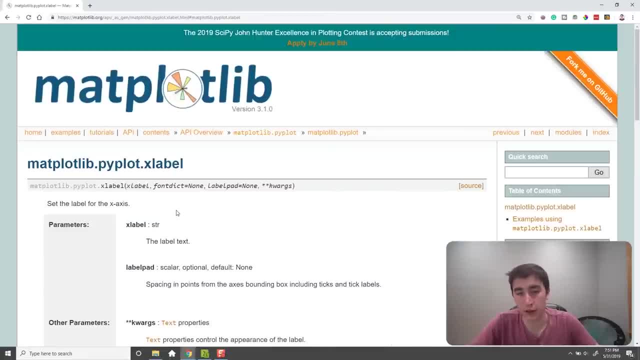 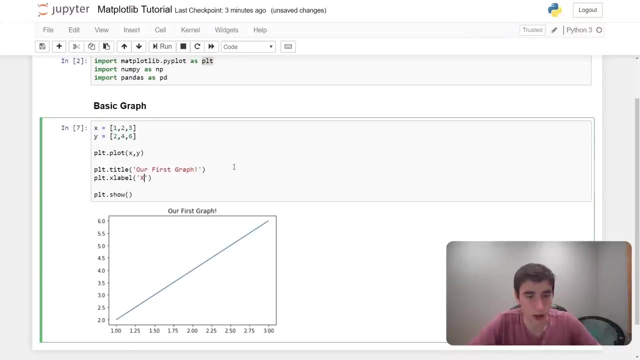 doing this and really easily find what you're looking for. I think it's a good place to go, if you kind of, just if you forget things, because I always forget things from that plot web. okay, so adding a label to X and Y- y-plotxlabel- x-axes. 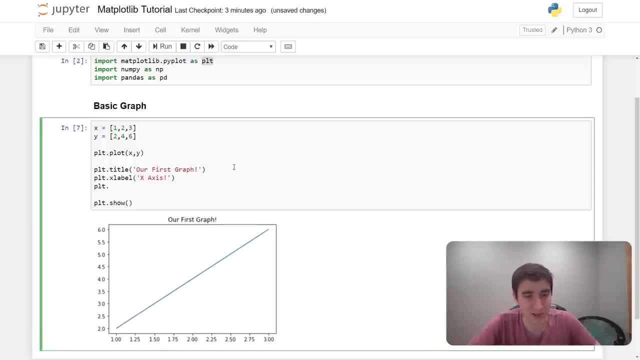 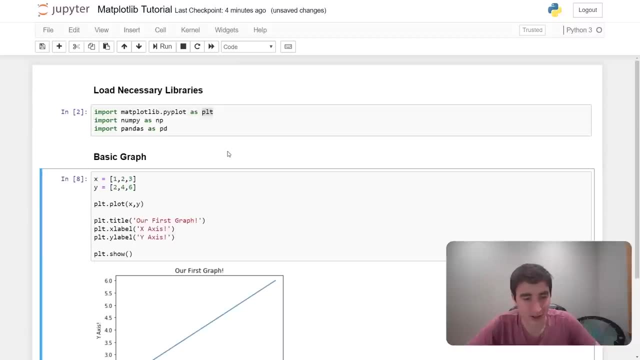 And I guess I'm getting really enthusiastic because I keep adding exclamation points to all my stuff: y-axes, Yay, Let's see what happens. Yeah, and I'm going to just get rid of these exclamations. I don't need them. 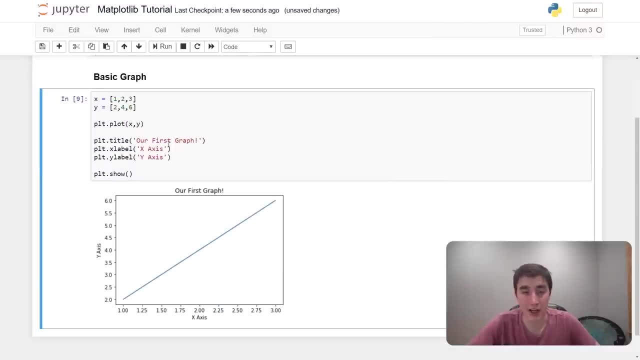 Okay, so now we have a graph and we have a title and we have y-axis, x-axis. In a real graph we would label these properly, but for the sake of this example- we're just kind of getting a feel for how we add these- 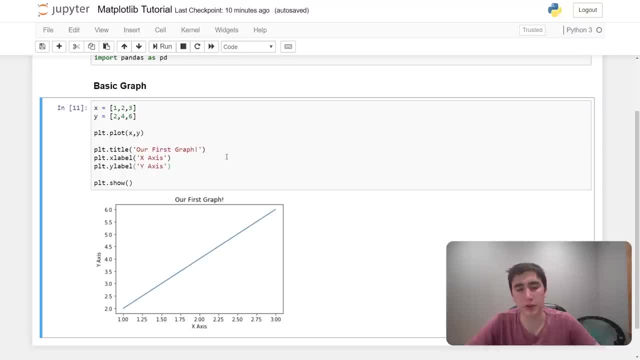 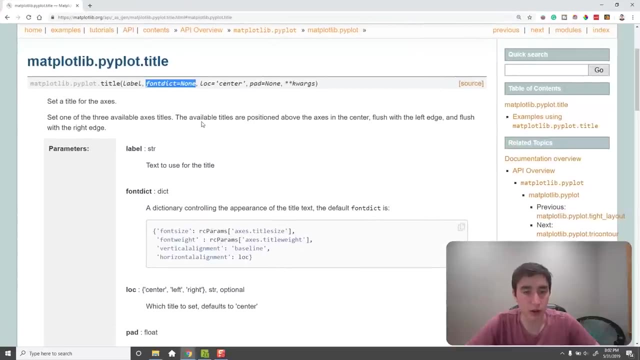 All right. so now that we have our title and labels, one thing we might want to do to them is resize them. So if we look at the documentation for title, one thing you'll notice is that you can use, you can pass in this font dictionary. 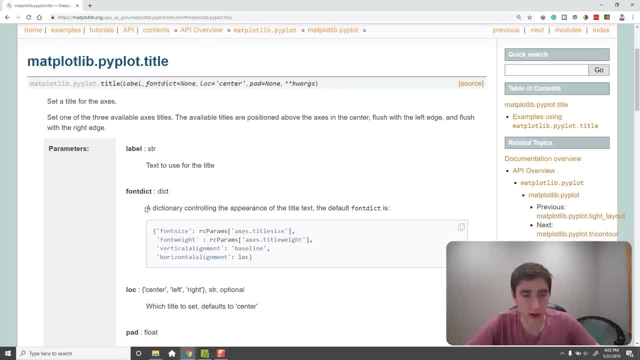 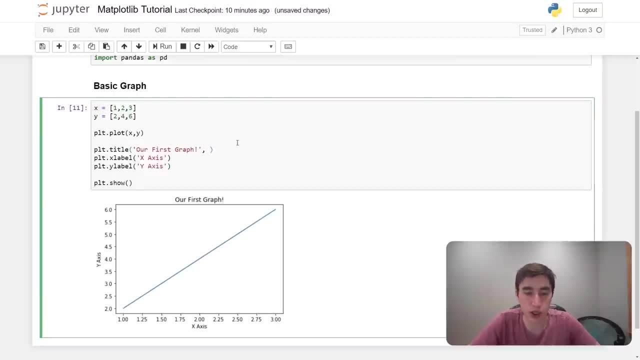 and it gives you a little bit of details about the font dictionary here. But basically there's all sorts of options that we can do and play around with our font. So let's say I wanted to change the font of our title. I can do font-dict equals. 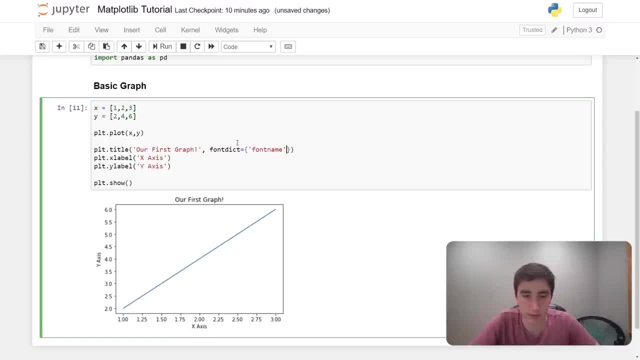 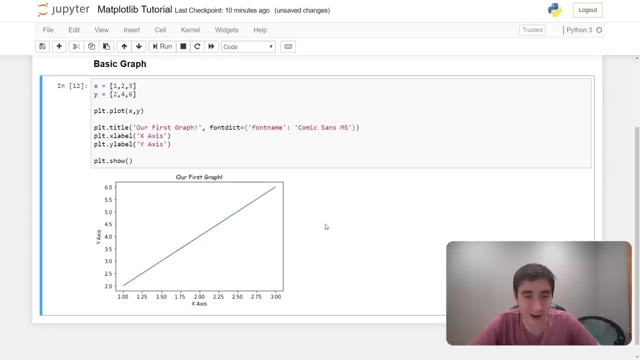 and I can pass in font name And let's say, my good old, trusty, reliable Comic Sans MS will be our new font And if you look at that, we got a nice new font on our graph. And if you can't see it, 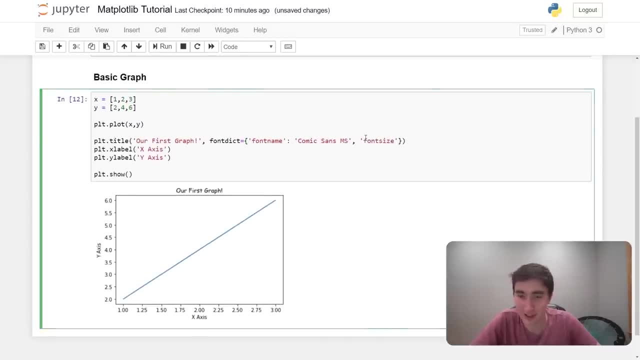 well then, in that case I'll change the font size to be something like 20.. Now you should definitely be able to tell that I've changed the font type, And in the description I put a link to all the known Matplotlib fonts that you can use. 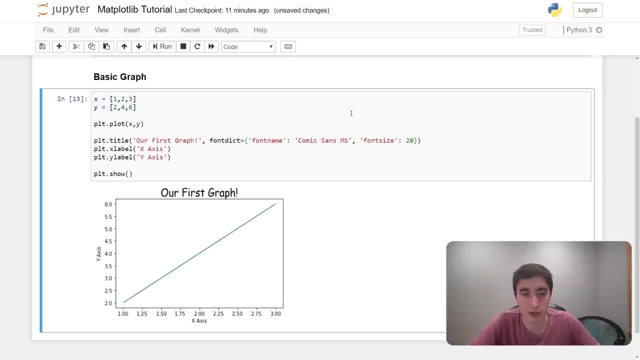 And if you look through the documentation you kind of find some different options. you can do with this, And you can also do the same thing with the labels. I could do like font-dict. Let's say I wanted to make this font REL. 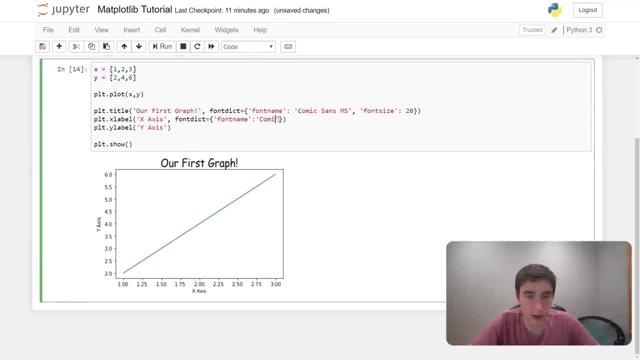 And that, honestly, might be the default, But if I did it, like Comic Sans as well, you can tell that the X-axis now has changed, But I'm going to just leave that at this B for now. Okay, So we did labels. 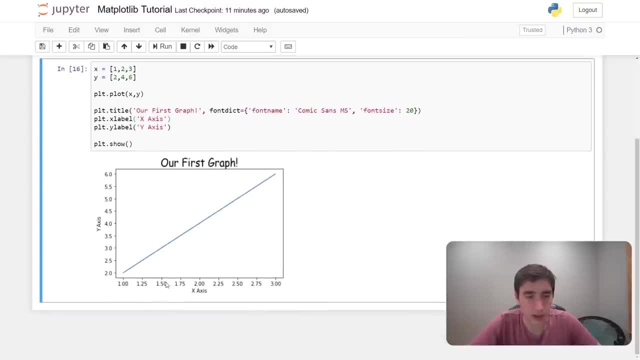 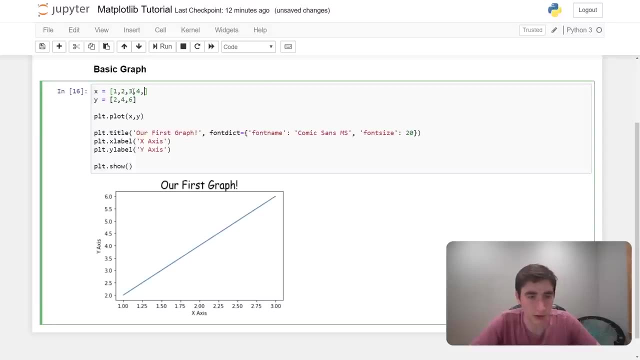 All right. So now, one thing that's bothering me is the tick marks. Let's say, I just want to do integer numbers And I'm going to add a couple more values to our graph, So I'm going to go to 5.. 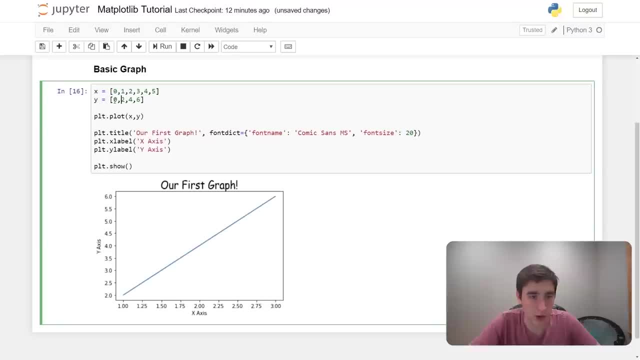 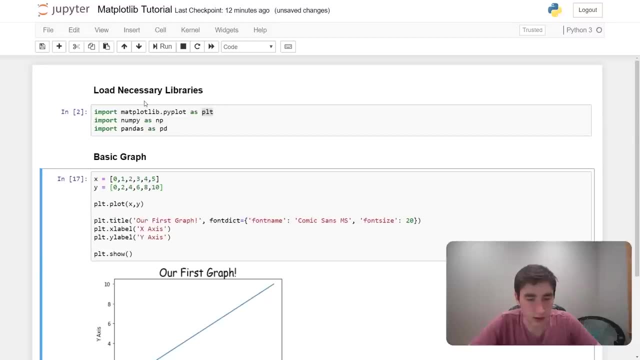 And we'll start at 0.. And Y is always going to be 2 times X, So it's going to look like that. Oh wow, It magically did it for us. in that case, I don't want it to magically do it for us. 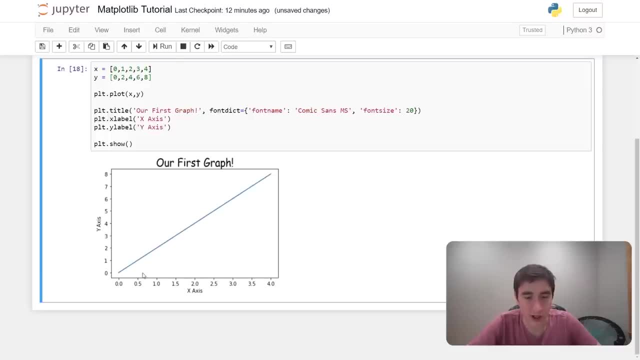 Okay, Let's say we went to 4. And we want it to be 4.. We wanted just the integer values. We didn't want any of the decimal values. So how do we change our ticks? So we can do that by doing plotXTicks. 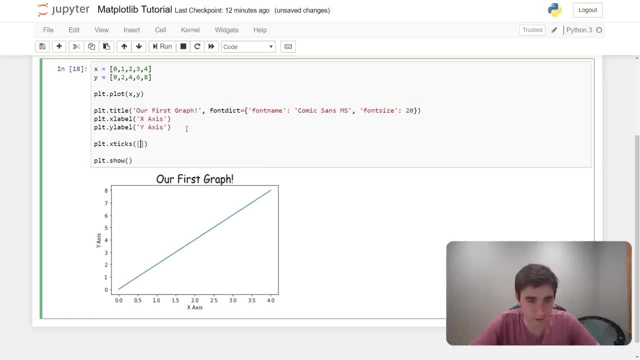 And our X ticks will do 0,, 0,, 1,, 2,, 3.. And I also just remembered this command by using the documentation. And our Y ticks will be how about 0 to 10 every 2.. 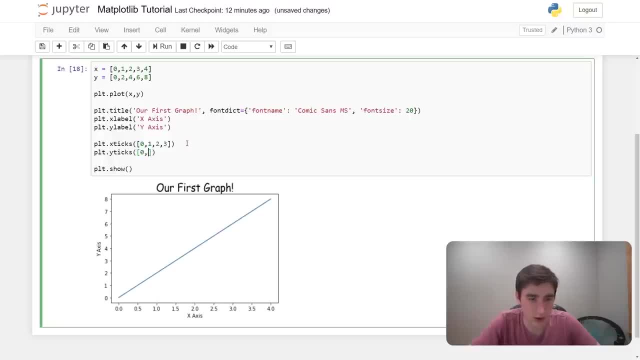 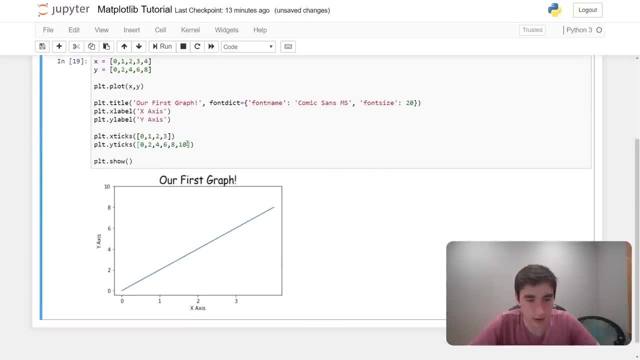 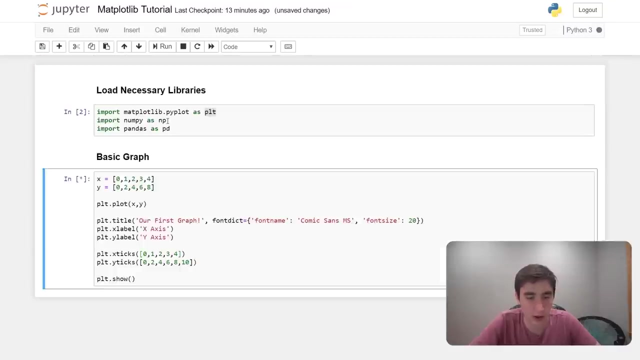 So it was 0.. 0,, 2,, 4,, 6.. Oh my gosh, 10.. As you can see that now we have the tick marks working properly, And maybe I wanted to add 4 as well. 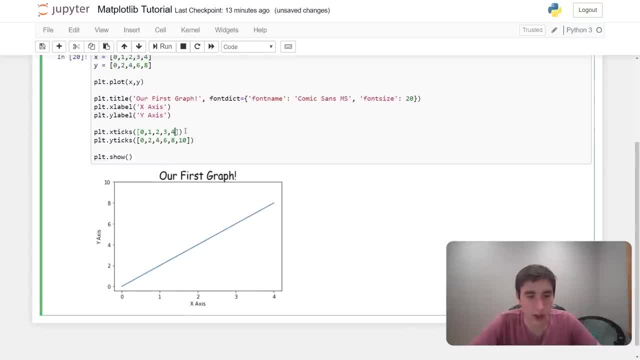 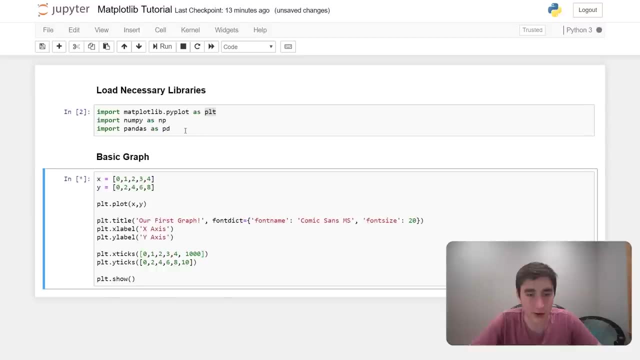 So now we labeled our ticks differently, And one thing that's cool to know is that the graph will automatically resize based on how we set this. So if I set 1 tick to 1,000.. Heh Well, now our graph kind of looks like not too good. 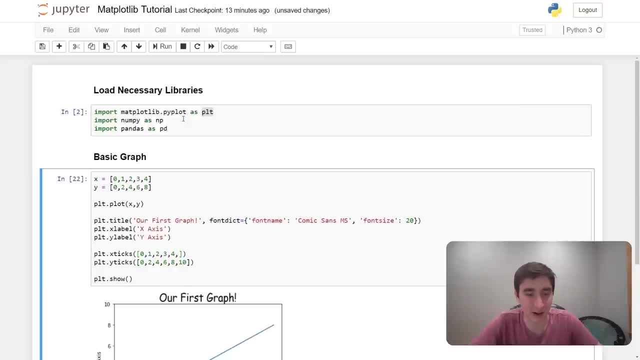 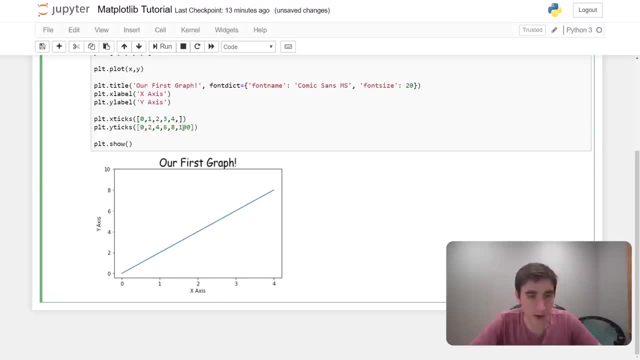 But it's nice that you can easily do that. 4 is better And you can do the same thing with Y. Let's say I wanted to make the last one 100.. As you can see, it changes up the sizing of the graph. 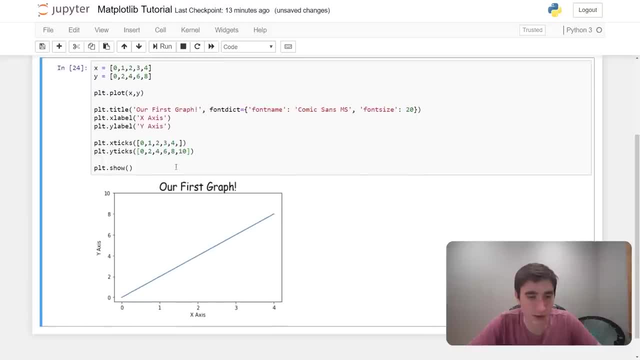 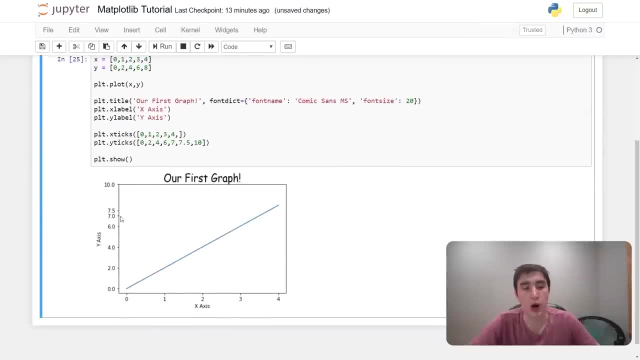 One thing that's also cool, though, is, even if I didn't evenly space these out, if I did like 7 here and then 7.5.. As you can see, it properly puts those at the right spot in the graph. 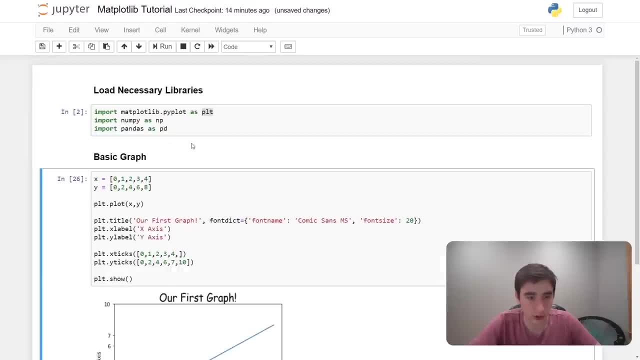 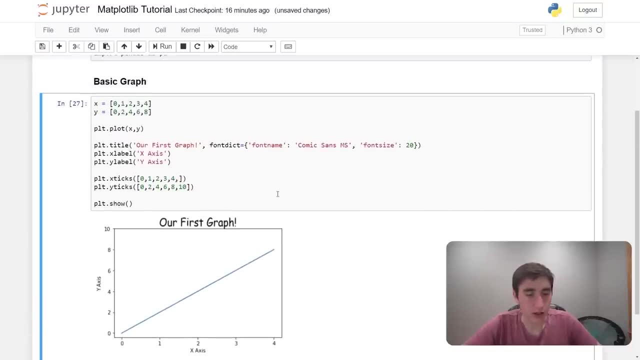 I'll leave it like this. I'll leave it a little bit weird, But yeah, That looks good to me. Okay, So we have our first graph. Let's add a legend and make this line a little bit more exciting, color-wise. 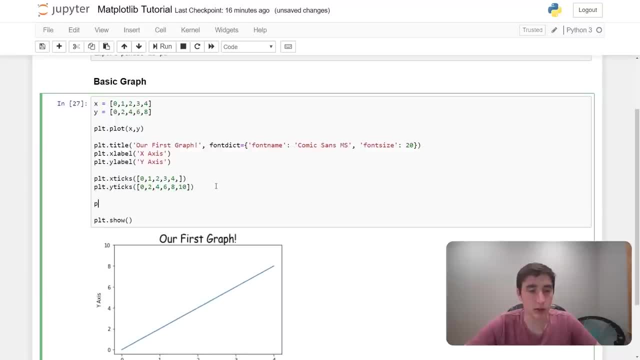 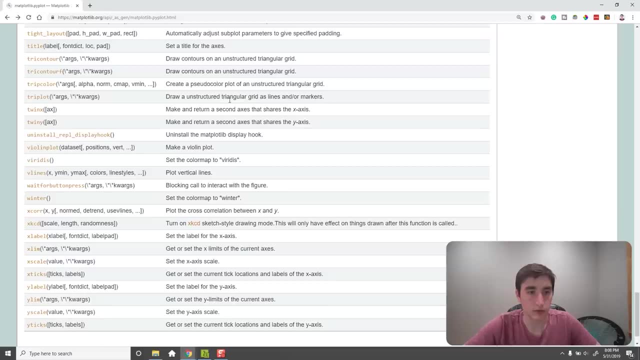 So if we wanted to add a legend, we can do, And I'm going to actually kind of like showing how the documentation is helpful, 5.. 1. If I looked up legend fig legend, that might work. Just this legend. 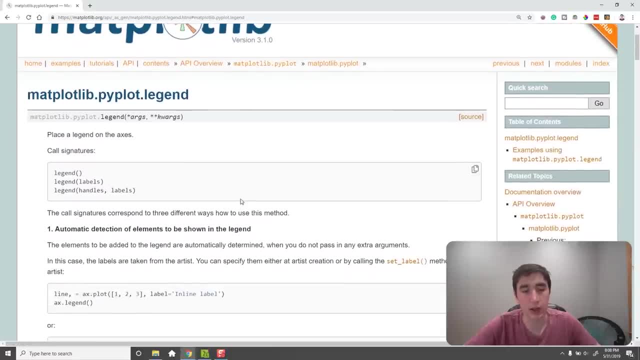 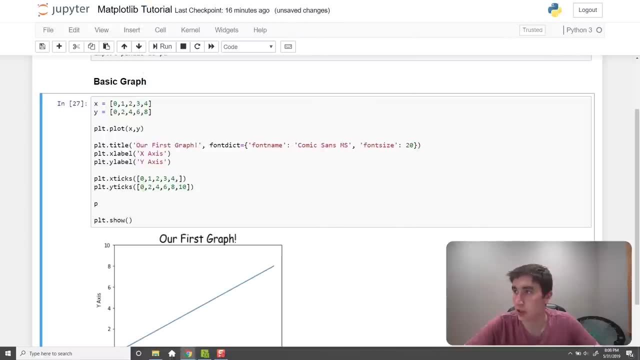 Place a legend on the axes, Like by looking up legend, I figured out that the call is just legend And it gives me some examples, So I always like to refer to this documentation. Okay, So pltlegend. And what happens when I do that? 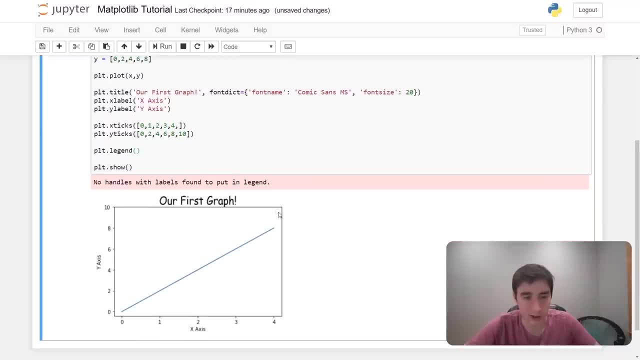 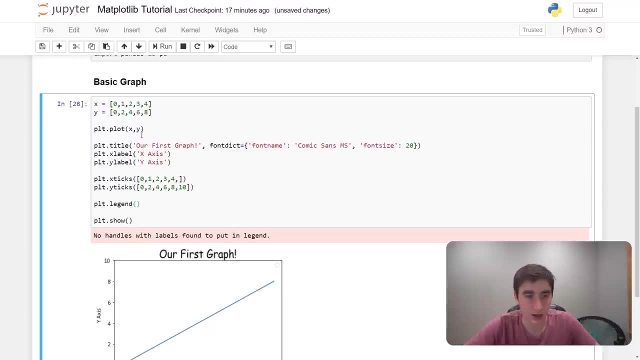 No handles with labels found to put in legend, So it's complaining because we don't have anything to label. What it's saying is: how do we label this line? And the way we do that is by passing in a label to our plot function. 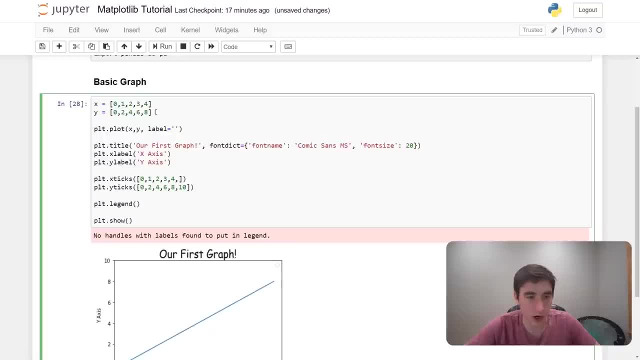 So in this case, our x and y. we plotted y to be 2 times x, So I'm going to call the label here 2x And, as you can see, we get 2x right there. Okay, Let's say now that we wanted to change up the color of this line, maybe make it thicker? 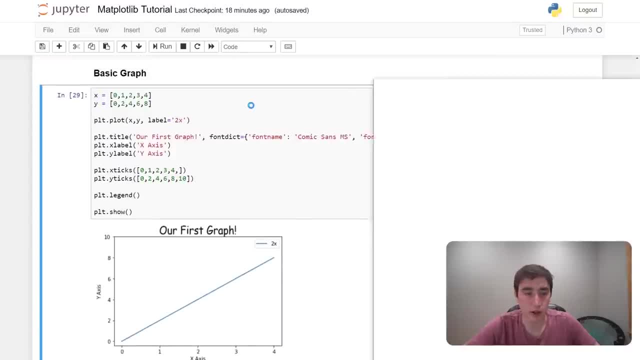 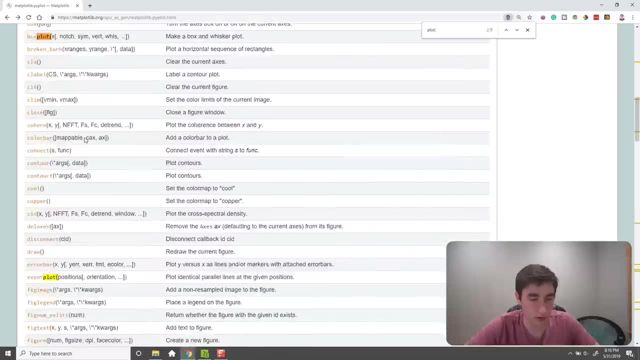 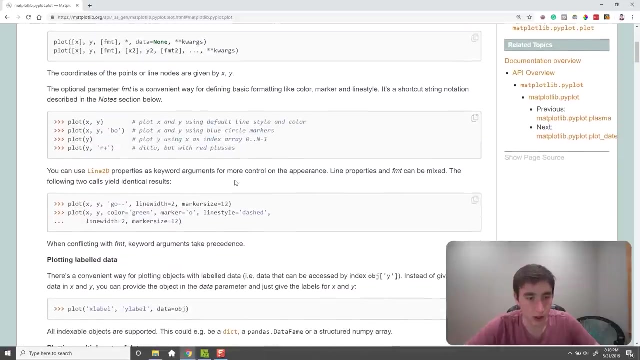 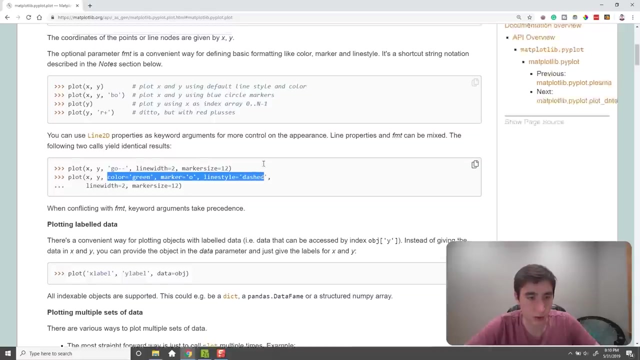 Do some other things to it. If we go to plot- where is plot? We'll see all sorts of properties that we can do in plot. So what I'm seeing right here is: you can pass in all of these different parameters to our plot. 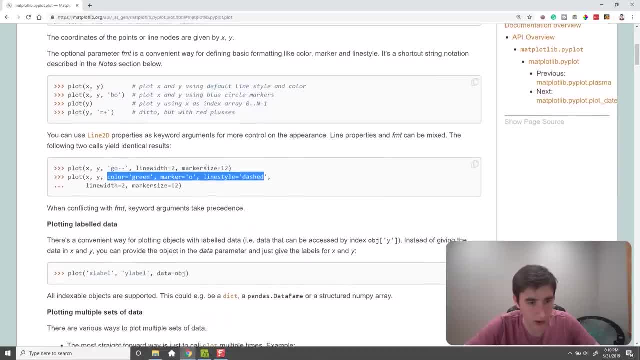 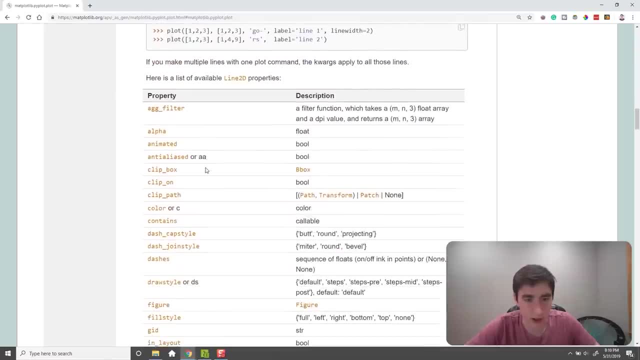 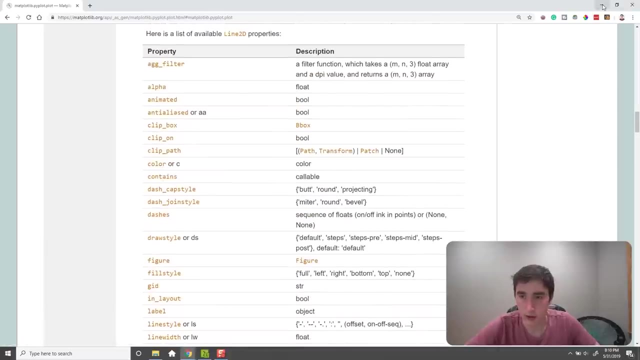 And it probably lists off what we can put. Maybe not, It's not super specific, But if you look hard enough, yeah, you can see all of these properties that you can pass into the plot function. So one thing we could pass in is color. 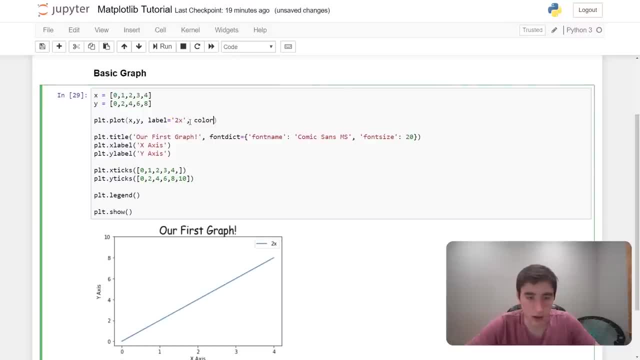 So if I passed in color equals red, it will work And it will know, I think, the common colors. So if I did yellow, if I did like yell, which is not a color, it's going to yell at you. 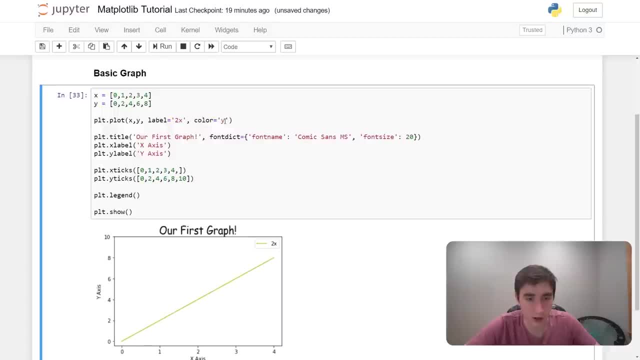 It might even work with Y. Yeah cool, And we also can pass in hexadecimal colors. So I could do like ABABAB And we got like a grayish color. This is helpful because you can use like a color picker tool and pick pretty much any color we want here. 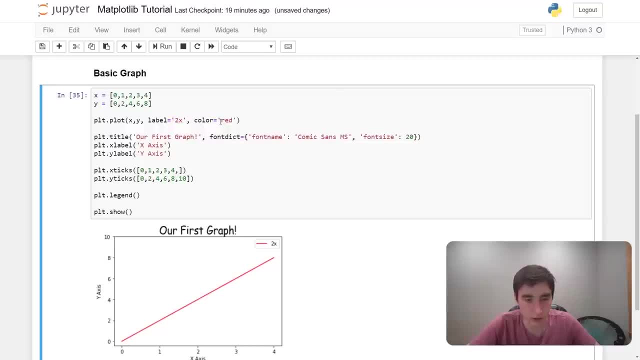 But we'll stay with red for now. The other parameters I could pass into that. Let's see what else we had I could do. I think line size equals, let's say, 12.. Oh, that is not a parameter. 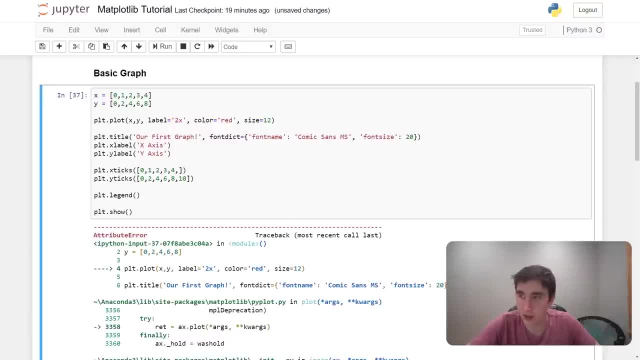 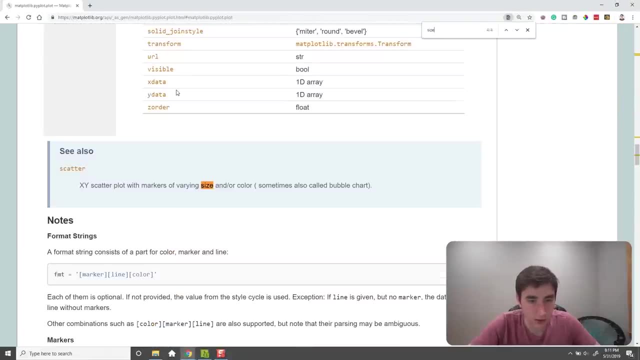 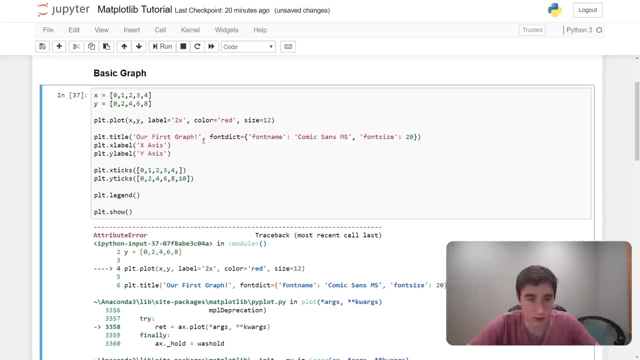 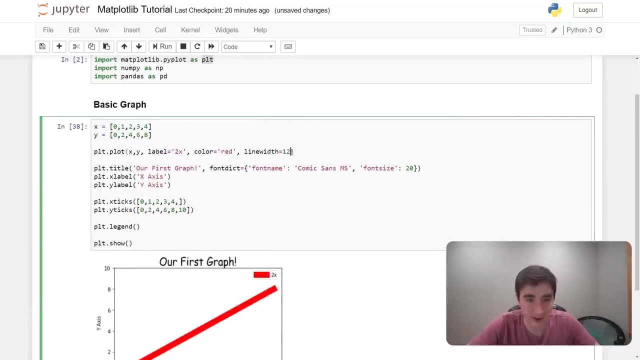 Ah, not a parameter either. Go back to my documentation: Size, Marker size. Maybe that's it, Marker size. Oh, I also see line width here. So line width equals 2.. Oh my gosh, Line width equals 12. makes this big line, maybe 2.. 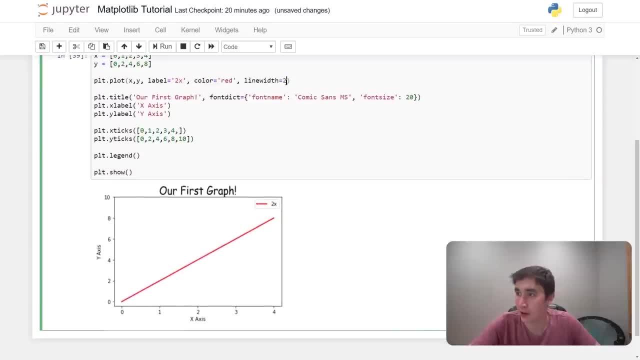 It's a bit bigger than I think what we had We can also do. we can label a marker. So let's say I wanted to add dots into this. As you can see, you can't really see it too too well. 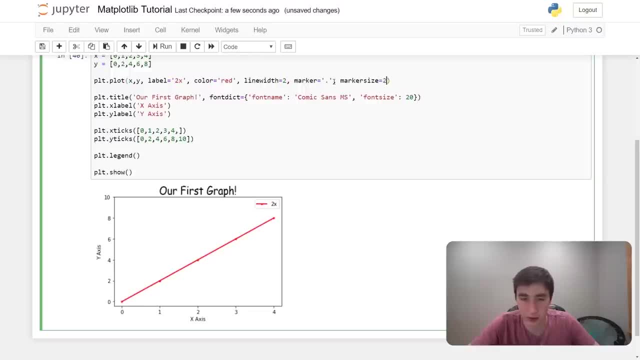 But maybe if I made the marker size a little bit bigger- And I'm just kind of passing this in so you can kind of see what you can do- Oh, that didn't work, Let's say 10.. Yeah, as you can see now you see big dots on our graph. 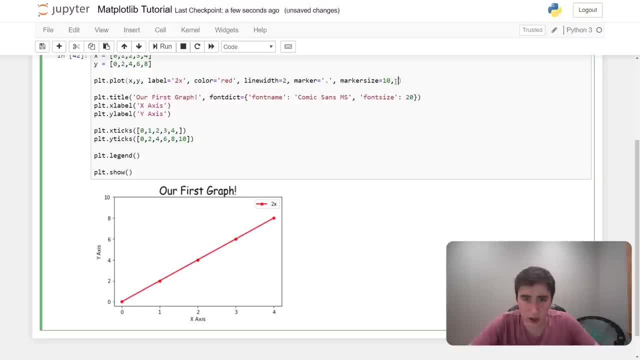 I can also do marker, edge color. There's all sorts of properties. I'm just like continually passing these in, But now you see a different type of dot and whatnot. So this is pretty cool that we can have all of this customization. 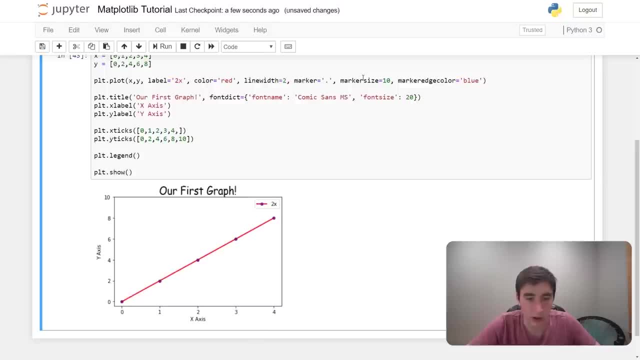 It sometimes takes a little while to get what we want, But it's usually. It's just nice to have this power. And one final thing I'll pass in is line style. So there's all sorts of line styles we can pass in. 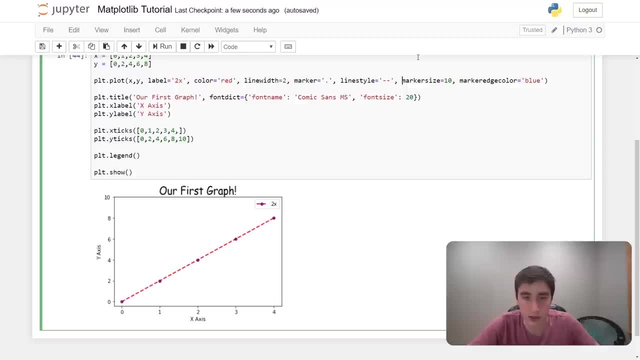 And you can read all into the different ways you can do this in the documentation. One thing that's pretty cool. One thing that's pretty cool is that instead of listing all of these keyword arguments, sometimes we just want to make a different type of line quickly. 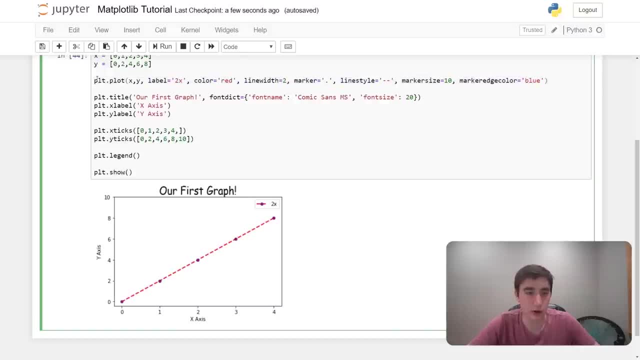 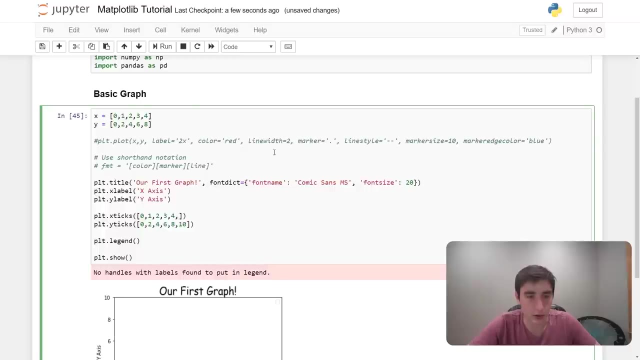 So there's actually a shorthand that you can use to kind of do pretty much the same thing. So, if I comment this out real quick, we have no graph. What you can do is there's a shorthand notation that allows you to kind of have a pretty good amount of customization quickly. 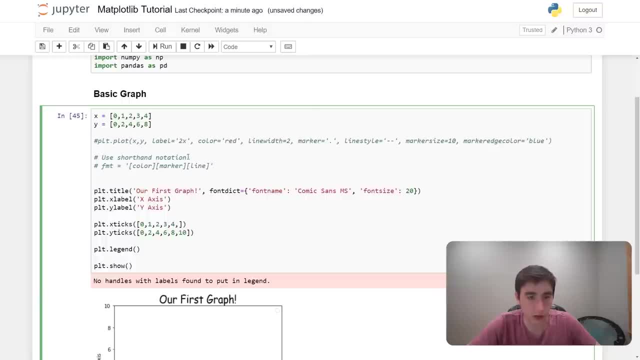 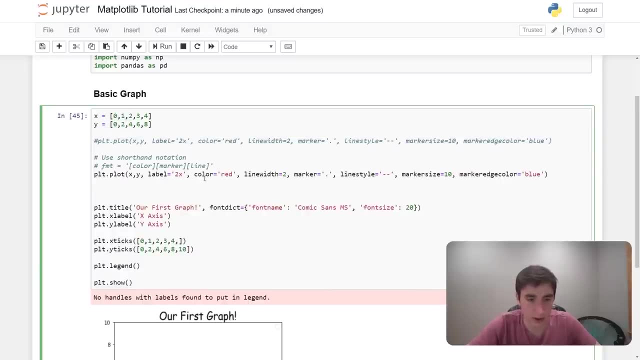 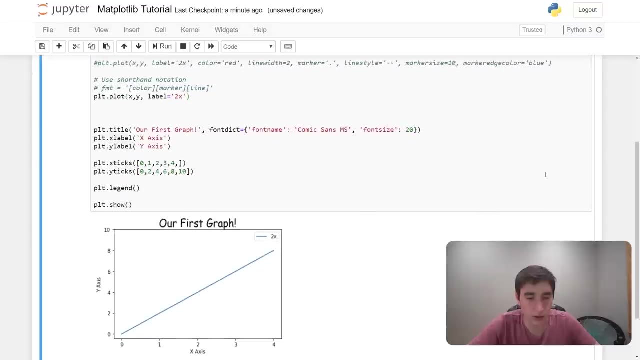 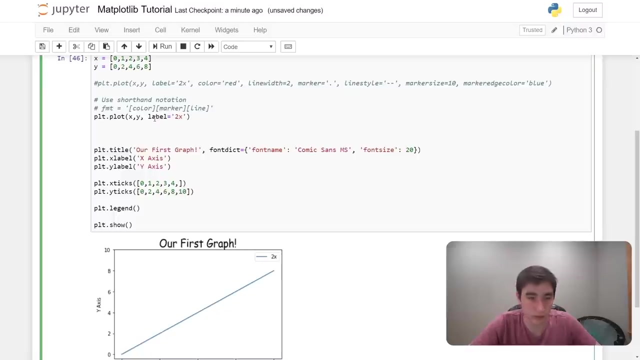 So the shorthand notation is color marker line, Marker line style, I guess. So if we go and copy this line from above, let's say we just passed in this. Now what we can do is, before we add our label, we can pass in the shorthand notation. 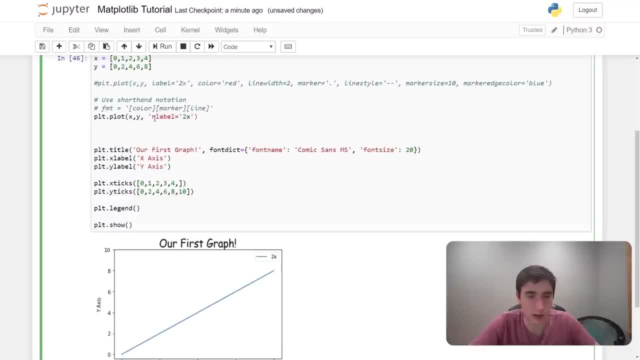 So I can do color. We'll say red, And I think it just accepts letters. We can look into the documentation and see exactly what it does. Marker, We'll do a dot And then line will do a dash. So watch what happens when I do this. 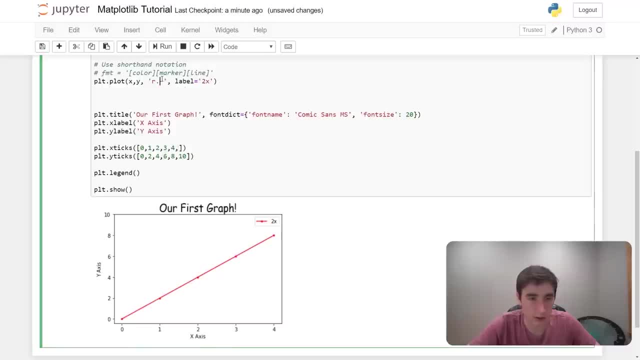 It gives us a nice line with dots in it. If I do two dashes it gives us a dotted line. If I do like a different type of marker, I can pass in like a caret. like that. It gives us a line with carets in it. 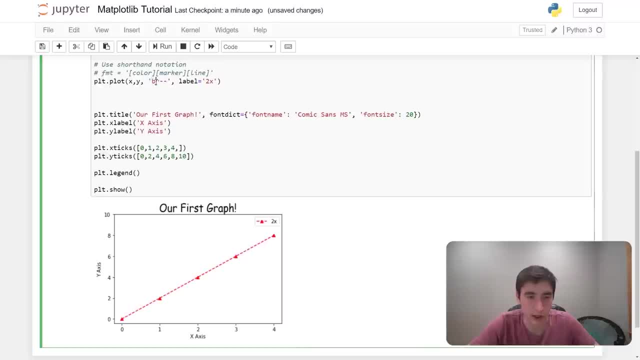 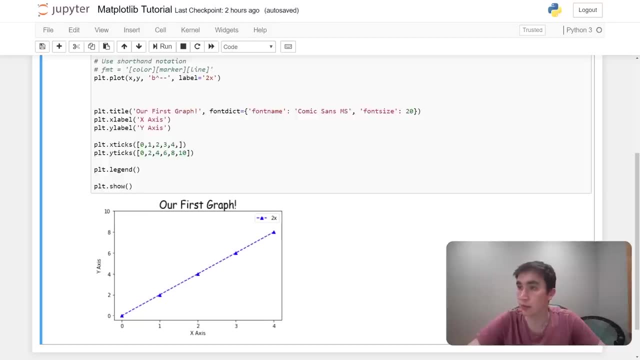 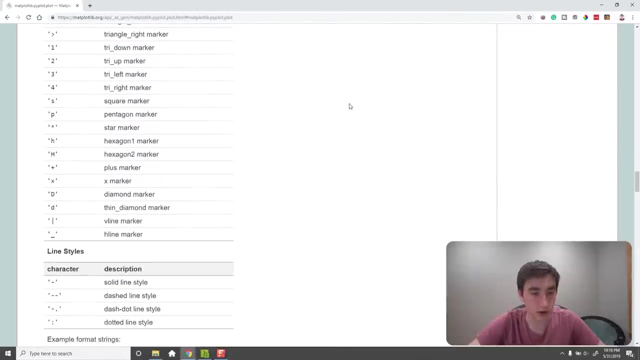 It's kind of cool that you can do this shorthand notation and get different types of lines Very easily. Just to follow up on the whole shorthand notation, I'm pulling in the docs for the plot function. It shows all the different markers you can use and the different line styles supported and the different colors supported. 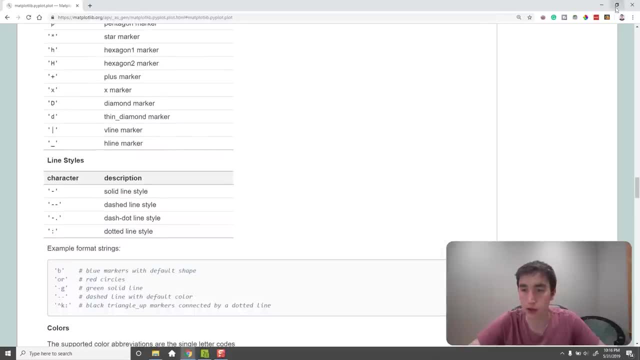 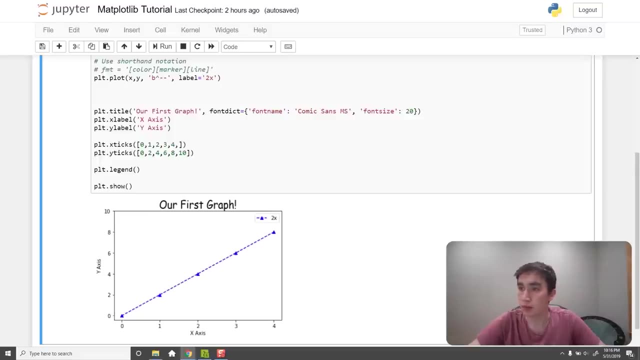 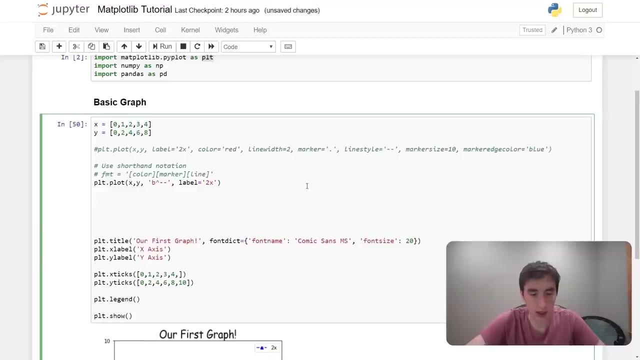 So check out the plot documentation to see all that. All right, Let's move on to our next thing, And that will be, I guess. let's just add another line real quick to our graph. So we have our first line. Let's add line number two. 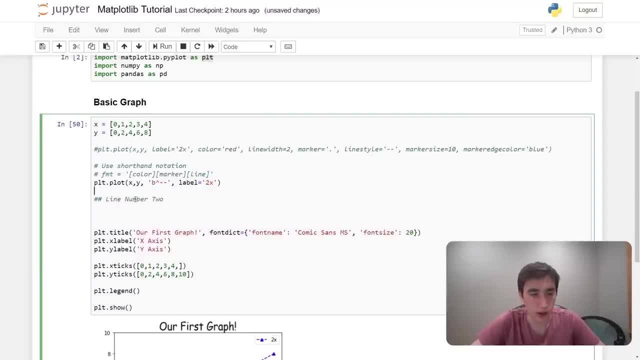 And this one will make a little bit more interesting. And the thing is like here we had a very straightforward like you have X and you have your Y. But this is not always easy to do, especially if you have like a function like sign, where you want to plot it at like a bunch of values. 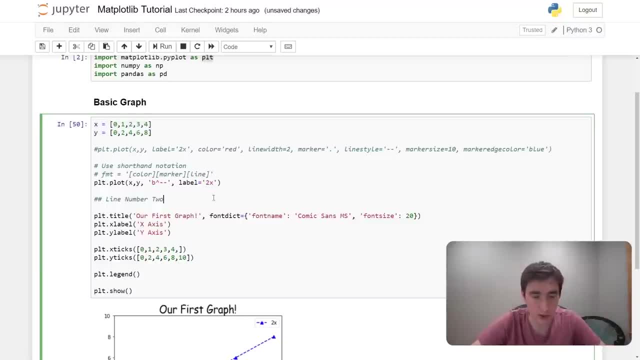 But those values are all, like you know, crazy decimals, So I'm going to show you how you can handle something like that. So this is where we use numpy, So I'm going to call this X2.. I'm going to say that X2 equals nparange 0 to 4.. 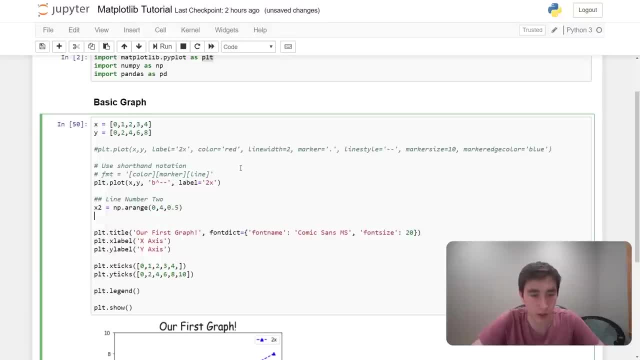 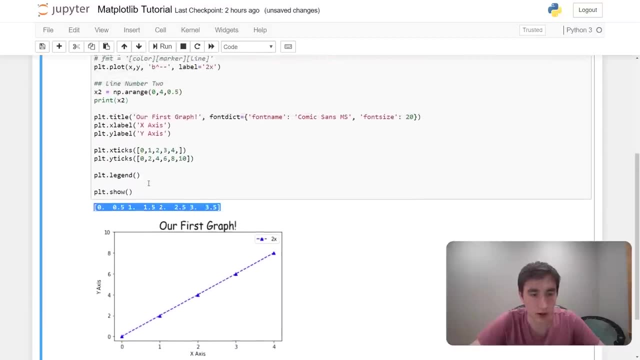 And we'll go by 0.5 as our tick. So if I print out X2 real quick, you see that this gives us a numpy array with 0,, 0.5,, 1, 1.5,, 2, 2.5,, 3,, 3.5.. 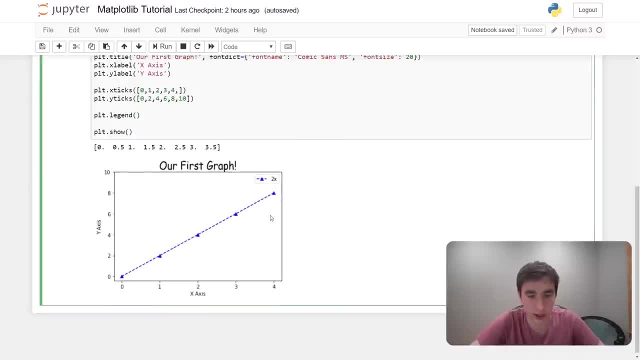 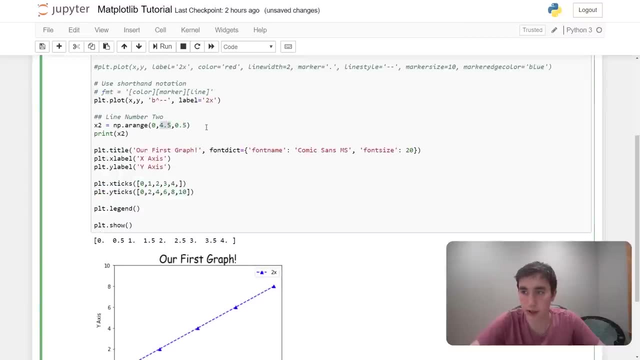 I'll actually make it go to 4.5, so it goes to the same spot as our other graph, because this is exclusive here. So we have that, So that's going to be our Xs, And so what I can do here is I can go ahead and plot that. 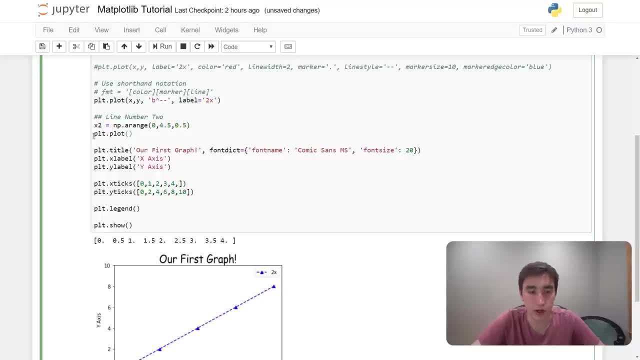 And I'm going to plot the square function for it. So I'm going to pass an X2.. And then, instead of passing in a Y, I'm just going to do X2.. And I'm going to do squared. What happens here? 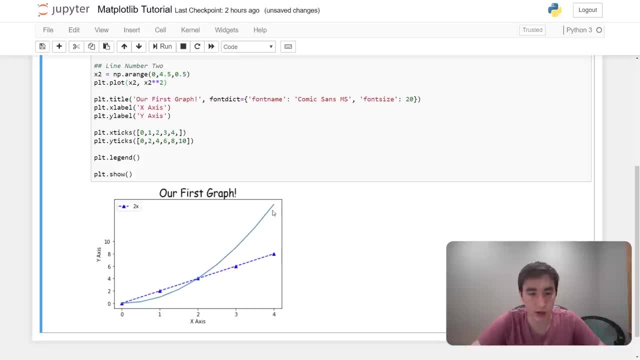 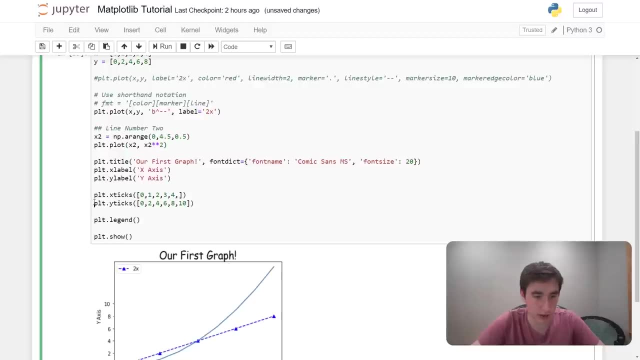 So now you see, we get X2 squared. It goes a little bit higher than our original axis was set. So I'm going to change up the ticks, Or maybe I'll just kind of comment this out and see what happens for our tick marks. 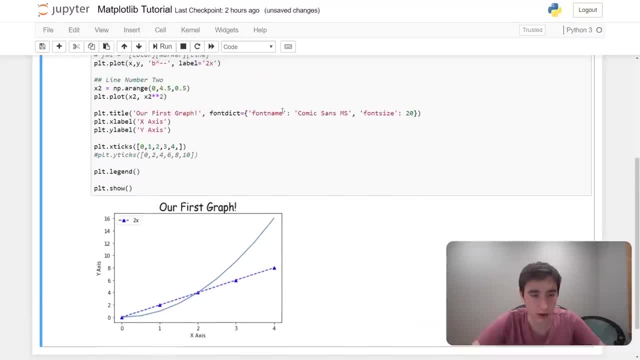 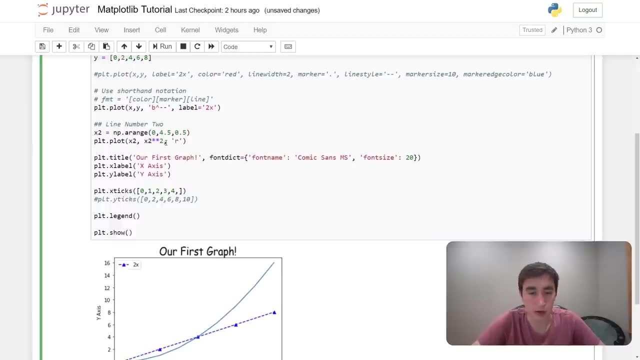 Yeah, I'm fine with just leaving the default that it gave us. Looks good to me, And now we have two blue colors, So let's make this a different color. Maybe we can make it red. We want to give it a label as well. 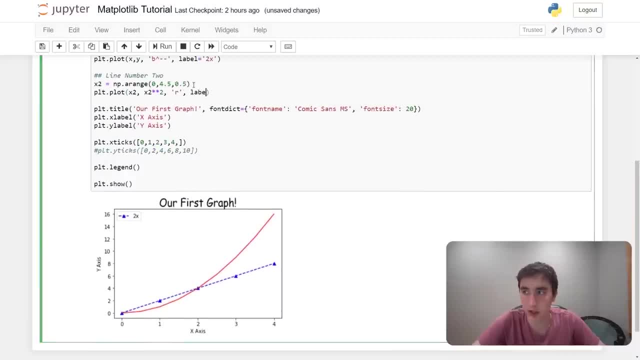 So I'm going to do red And I'm going to say: the label is equal to X squared. And one thing that's cool is that it automatically moved this legend to the top left because the positioning was better now that this goes up to the top right. 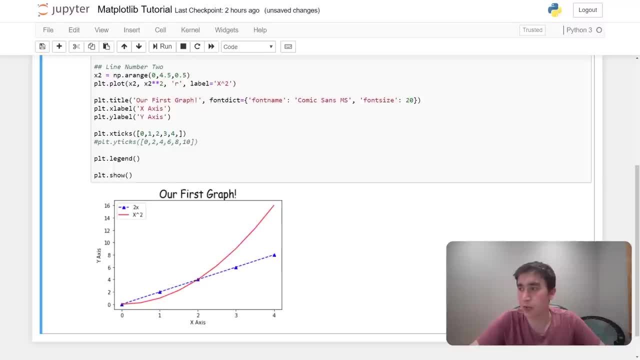 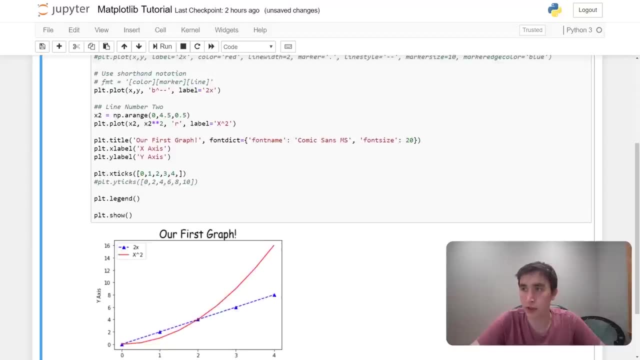 So we have two lines up there And from the original image I showed, there's some stuff that's still different. One thing that's kind of cool that you could do is, let's say, you had a graph that stopped, but you wanted to kind of show the projection of it in the future. 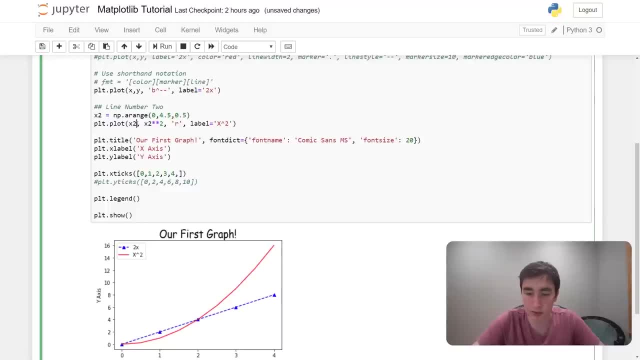 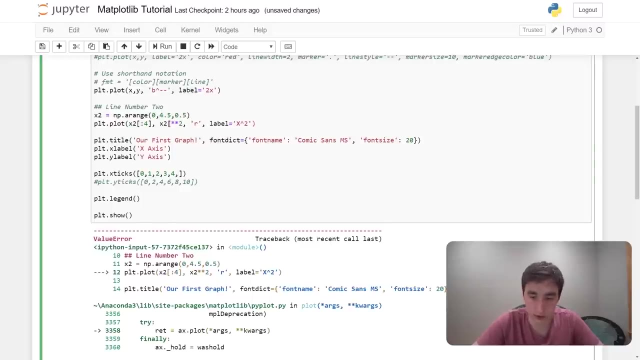 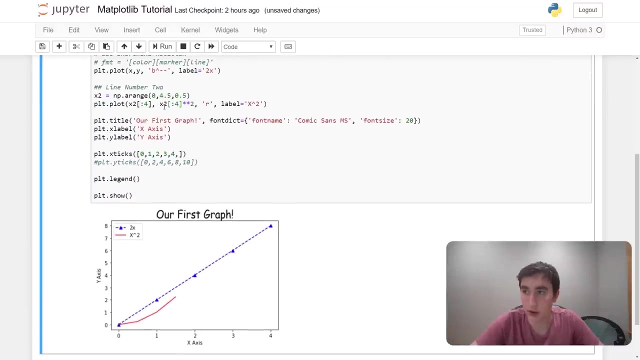 So what I did to show that type of a phenomenon is I did like X2, take the first four values here and we'll plot that. What did I do? Oh, shoot First four. Is that what I want? I think that will work. 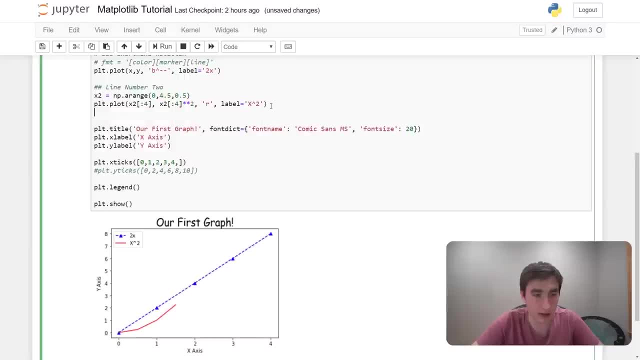 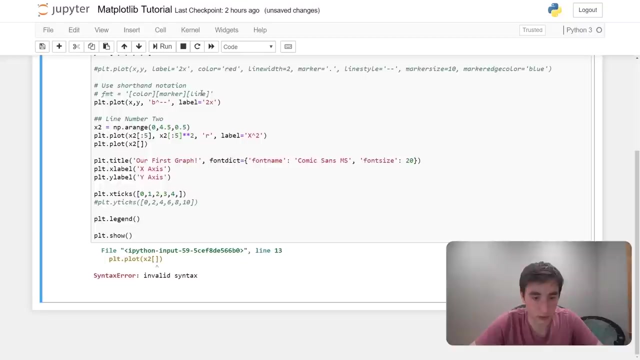 Take the first four and plot that, And then for the last values. so from, let's say, five or three, Let's make this a little bigger, Make this six or five, Bear with me here. From four onward, we'll make it a dashed line. 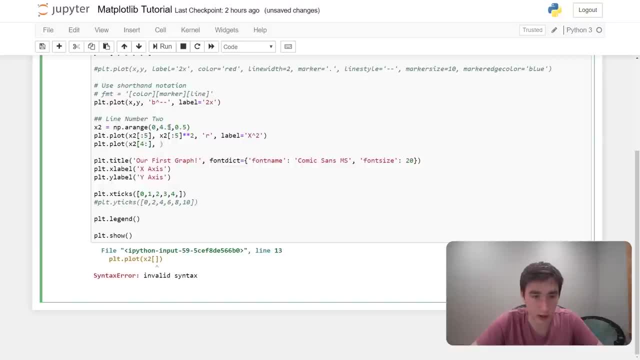 And I had a little bit of overlap because I think it will look better. You'll see, in a sec, Four dash: We'll make this still the same function, but this time we're going to make it a dashed line. So there you see. 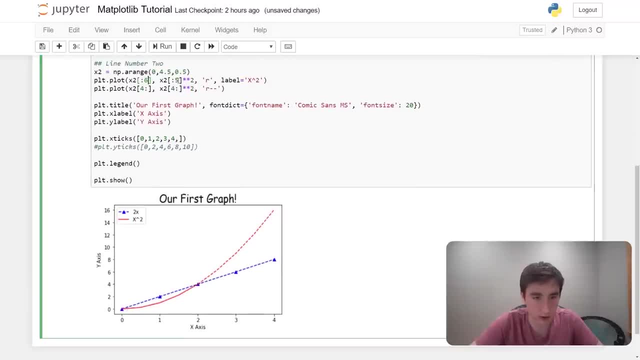 And I'm going to actually make this a little bit different. There you see, like maybe something ended here and then you make it dashed the rest of the way, You could do something like that using the format I just showed. All right, What else do we have? 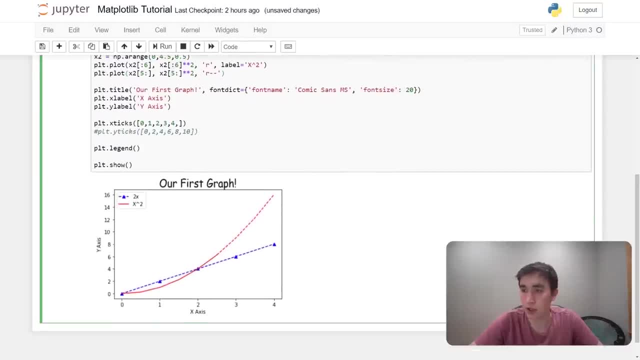 I'll probably clean this code up a little bit. Another thing that I showed in the original graph that I showed when I was introducing this video was a resize. So let's say we wanted to resize our graph. Well, we should do that, probably near the top of our graph. 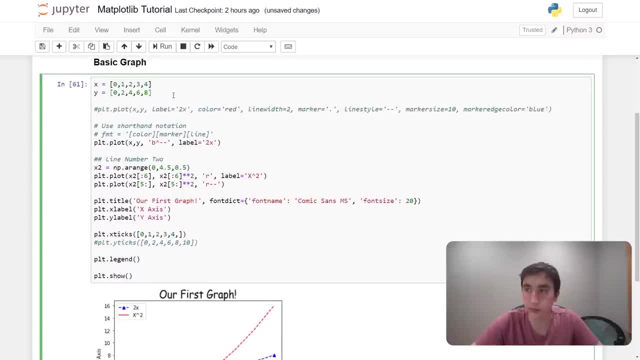 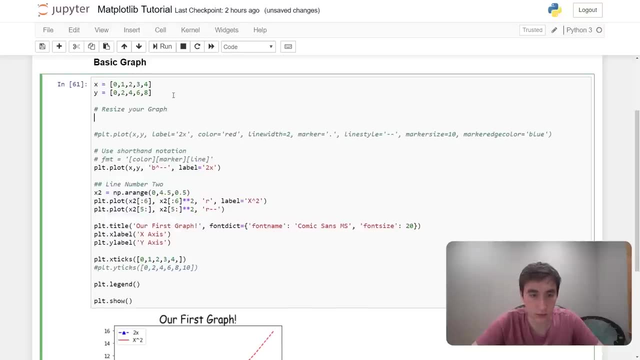 So I'm going to go ahead and do resize your graph, I'm going to go ahead and do plot dot figure Pass in fig size And we're going to say let's make the dimensions five by three. It's kind of an arbitrary five by three. 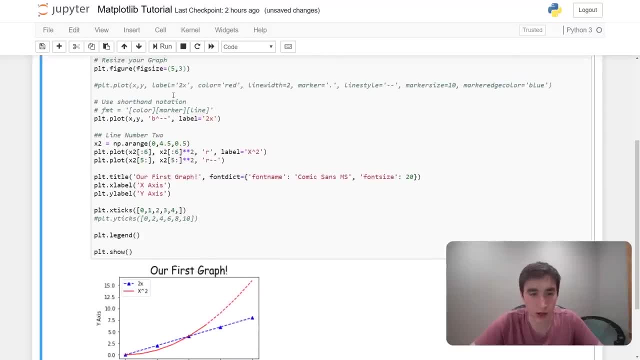 That will give you kind of the ratio of your x to your y. But to specify how many pixels it is you're going to want to pass in a second parameter, which is dpi, which basically is pixels per inch. So I recommend using a value of around 300 here. 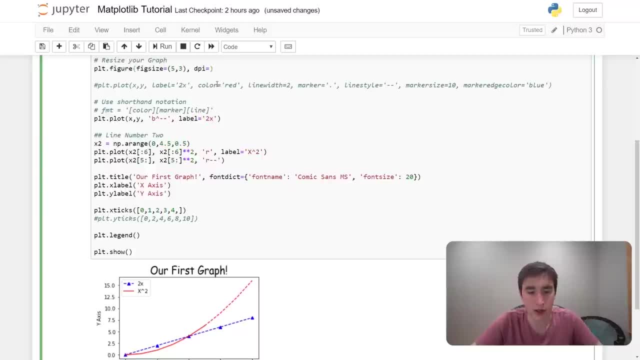 If you do smaller values, you'll have more pixelated graphs. So if you can afford having a bigger image, having a bigger dpi is often nice. So in this case we have pixels per inch of 300.. So this is going to actually be five inches by three inches. 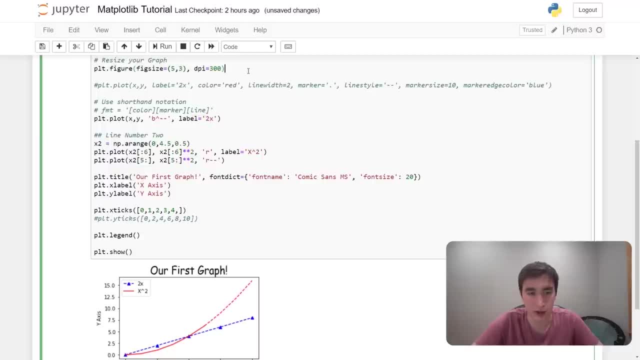 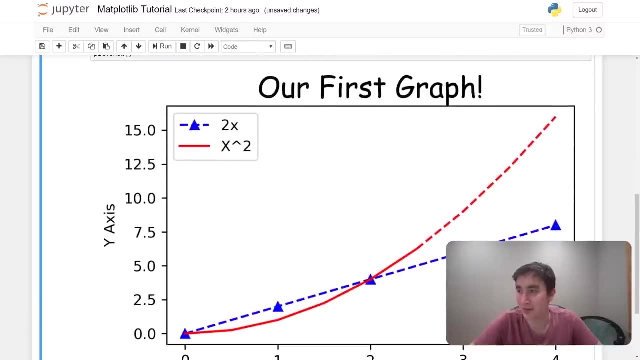 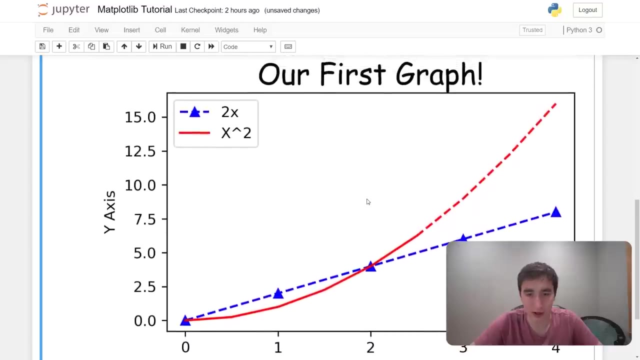 So the total pixels will be 1500 by 900 here in this graph. So now it's much, much bigger. Maybe it's a little bit too big. I'm going to be blocking this graph, So I'm going to make it a little bit smaller. 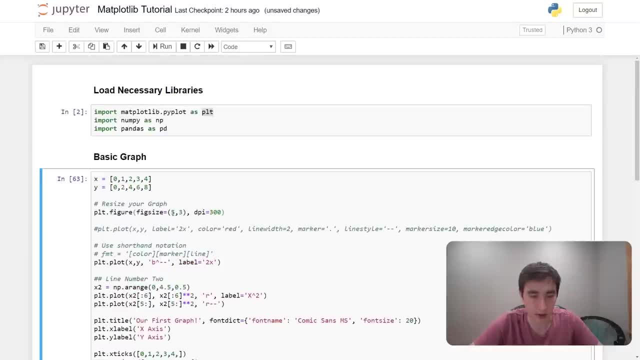 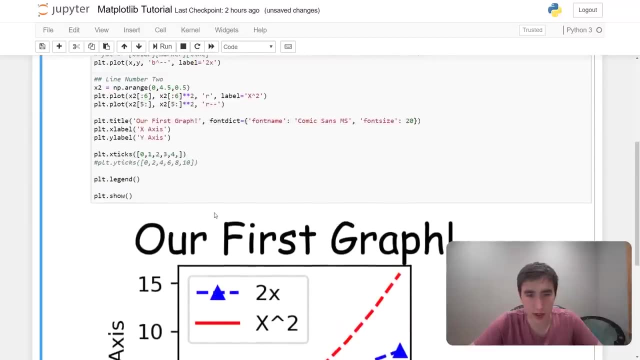 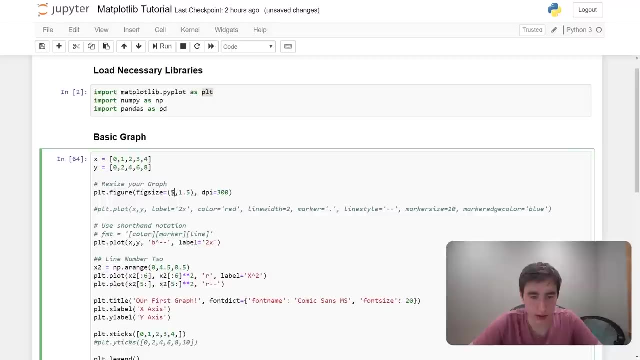 But you get the idea then here, So I'll make it like two by 1.5.. That's not a good dimensions. now, though, I mean just play around with this. The biggest issue I have right now is the graph looks so big. 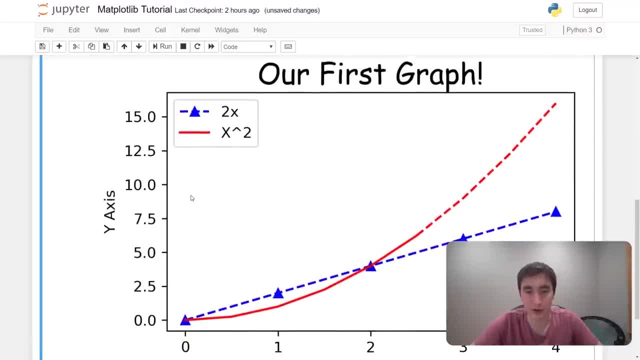 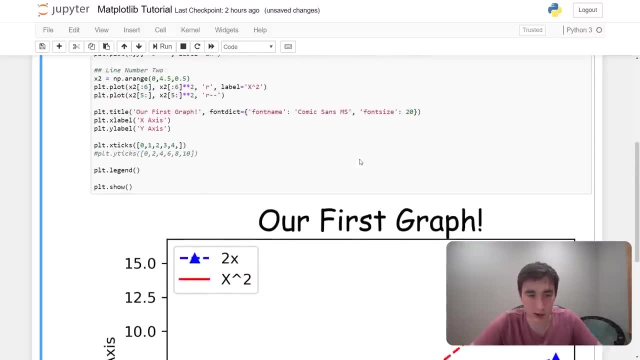 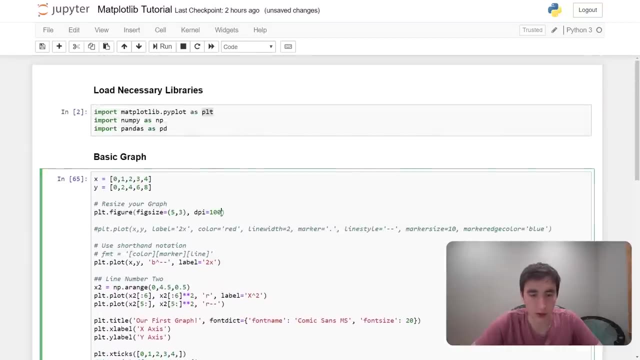 because I have my screen super high resolution or super. The view is like very up Close, because I want to make sure you guys can see my code. But yeah, this would be a 1500 by 900 graph. I'm going to, just for the sake of the graph, decrease the dpi. 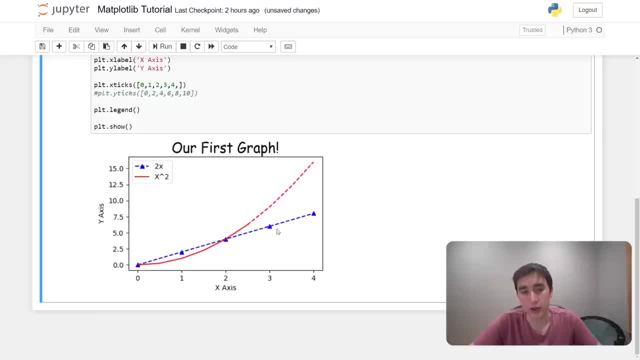 and make it more reasonable The issue. you can't really tell from this image, but if you really zoom into the graph and maybe, if you like, printed the graph out, it would look maybe a little bit pixelated with a dpi of 100.. 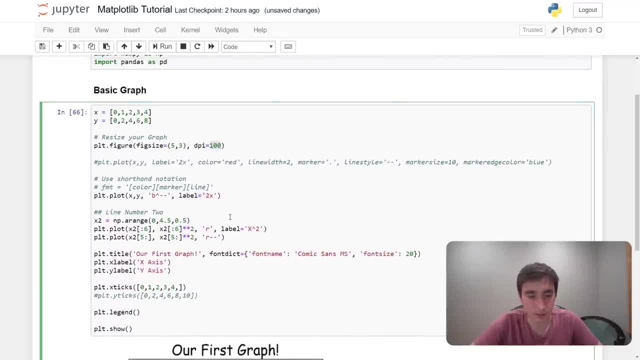 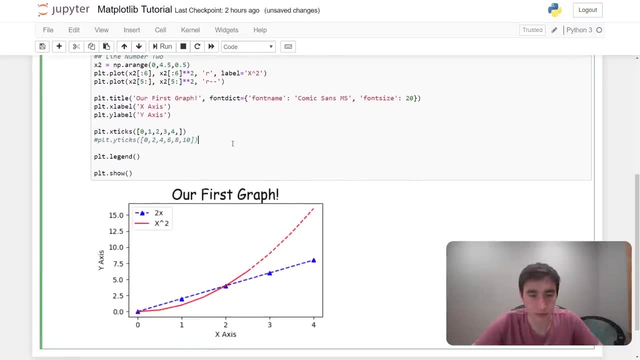 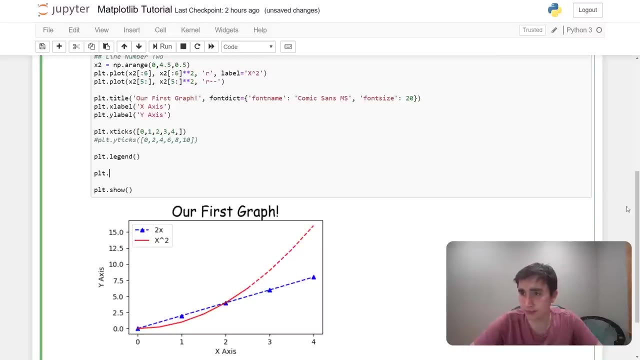 So probably try to keep this value higher if possible. And then another thing you want to do is you'll want to save your graph. So to save, we can do plot, Save fig And we can do, say, by graph, PNJ. 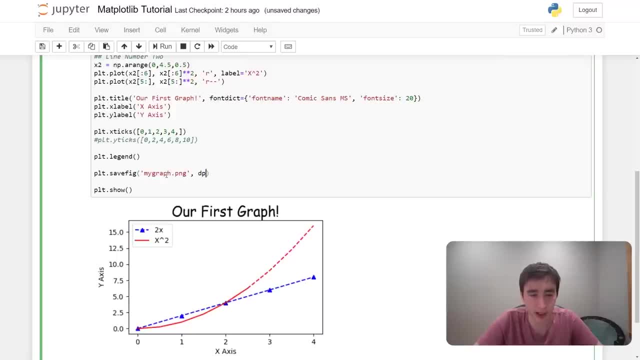 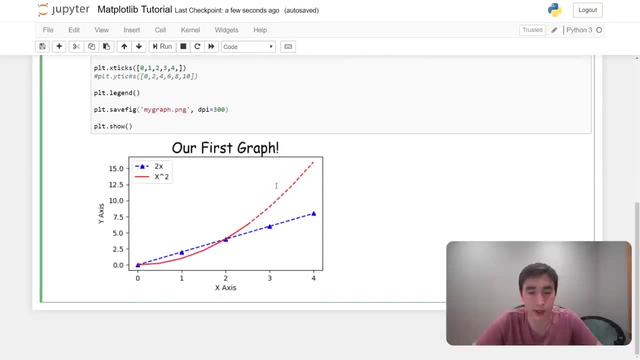 And one thing that's nice, too, is I could pass in the dpi parameter here as well. So let's say, when I actually save my graph, I wanted to be bigger, But for the sake of being able to show you guys in a smaller format. 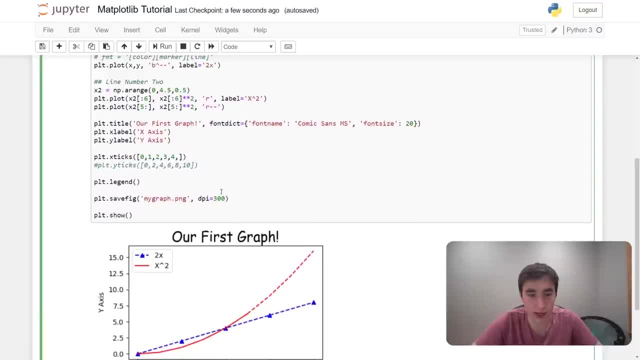 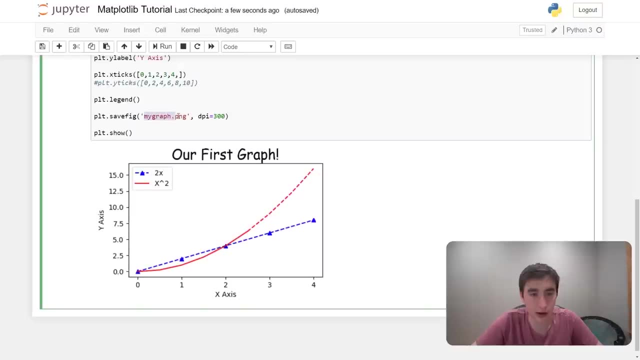 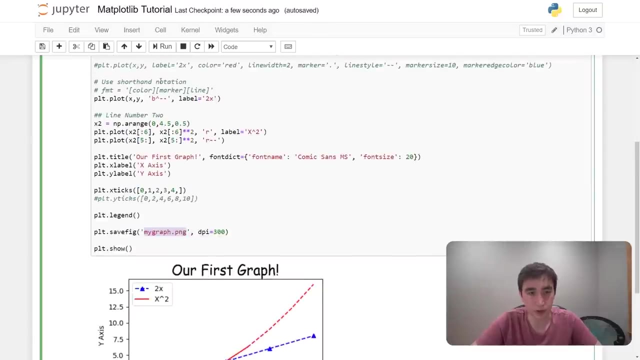 I wanted the 100 above. I can still go ahead and save it with 300 and then kind of solves both of my problems, And so this, then my graph dot PNG, will save in the current directory that this matplotlib tutorial is in. Yeah, we'll save in the current directory. 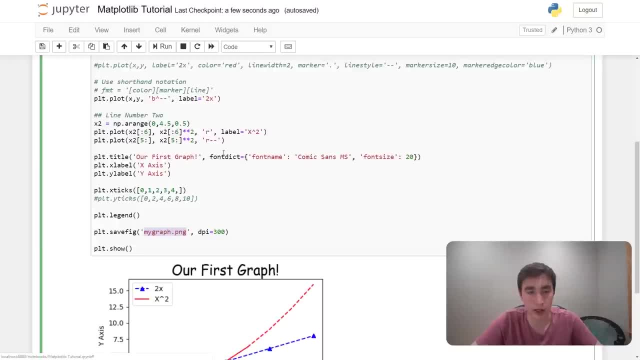 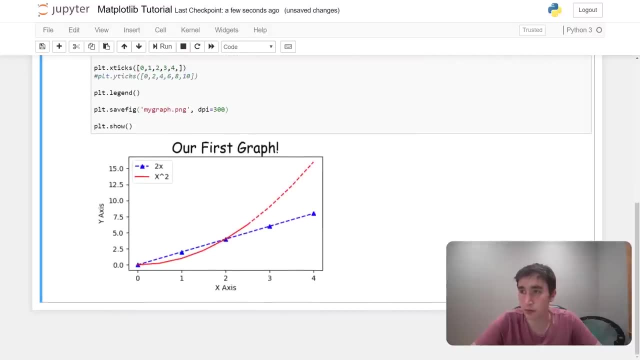 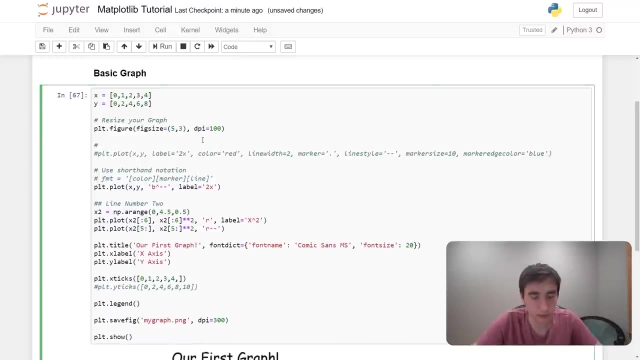 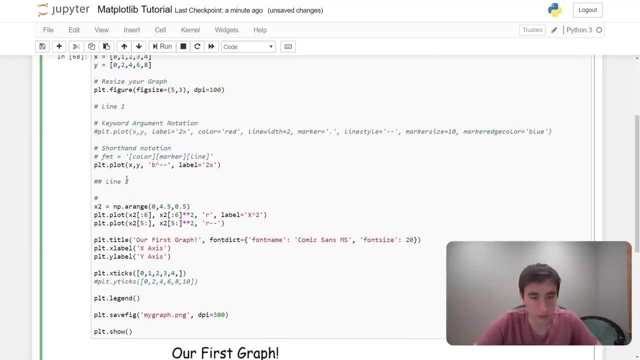 Whatever directory your file matplotlib tutorial is in, this graph will also save there when we run this. Cool, Now we have that saved. All right, Let me clean this up a little bit, And just to note the reason I did this is because this is exclusive. 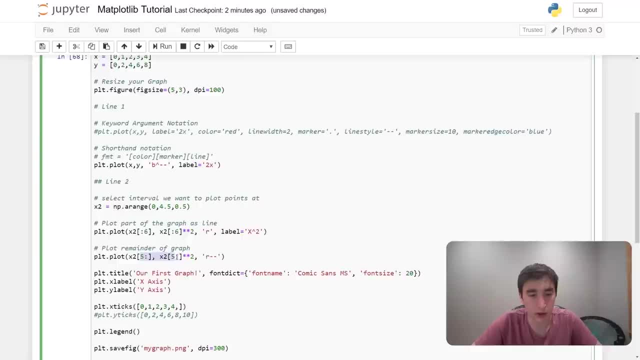 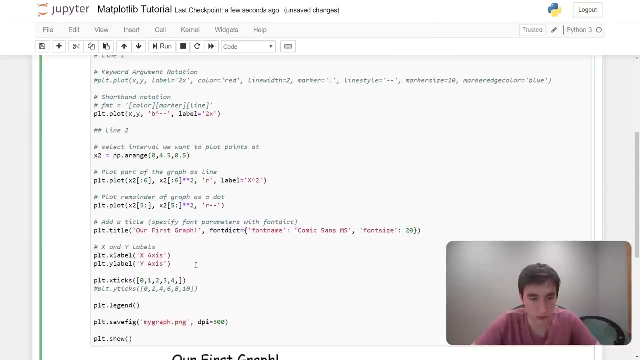 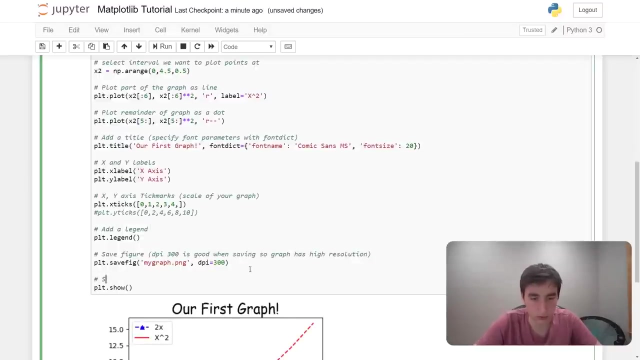 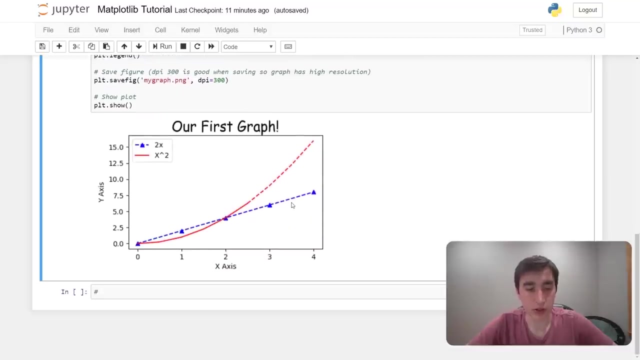 the six here. So when I do five onwards, it picks up. This actually ends at five because it doesn't include six. So it actually covers everything here. All right, Now that we've shown line graphs a bit, let's go and do quickly, do bar charts. 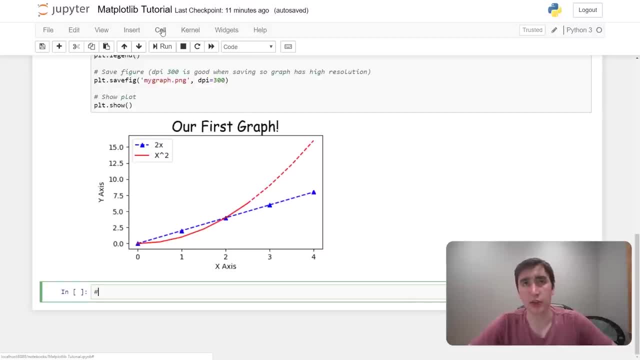 And after bar charts. I think we're going to just end this video short and I'll do the real world examples in a video that I'll post next week. I just think this video might get a bit too long if I include everything in just one video. 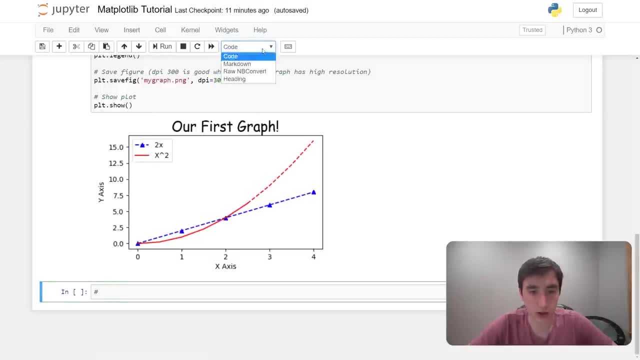 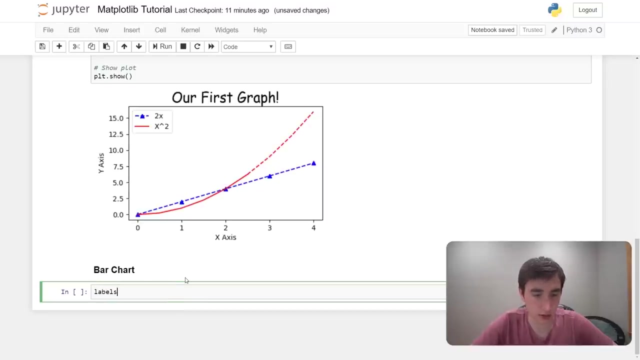 So all right, So I want to do bar chart. Okay, So bar charts are pretty straightforward as well. Let's say we had some labels- A, A, B And C- And some values, Let's say one, four and two. 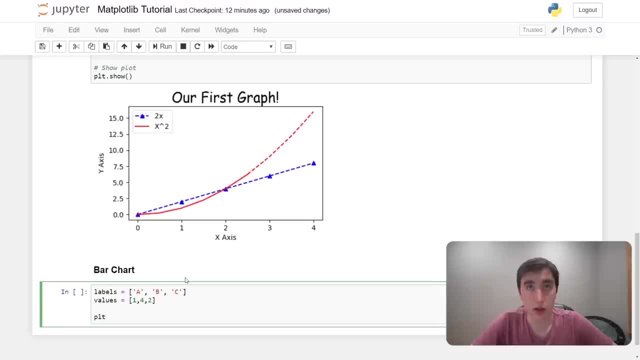 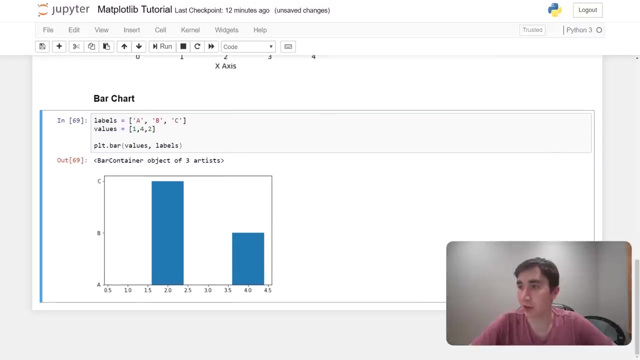 Well, if we wanted to do a bar chart, we could just do plot dot bar of labels, comma values. I probably did that wrong. It's values, comma labels, And we get not what I was looking for. Okay, Let's see. 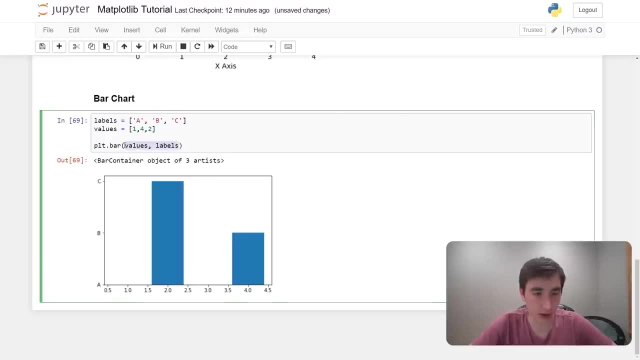 It is actually labels first, then values A, B, C, Cool. So that was pretty straightforward And I can do the plot dot show. We can do all of the adding of titles and whatnot the same way as before in the line graph example. 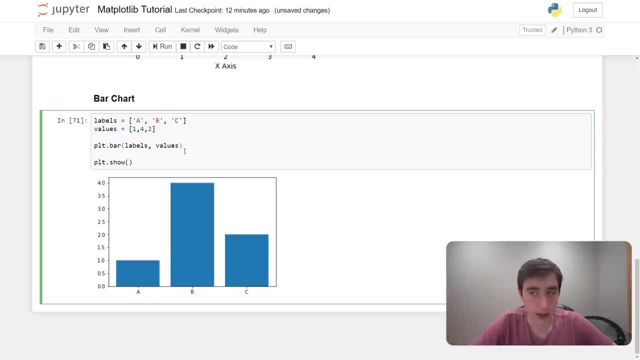 Let's skip over that for now. We could also resize it. let's say So I could do plot dot show Plot dot figure Fig size equals, let's say, six by four. It's going to use whatever the default DPI is. 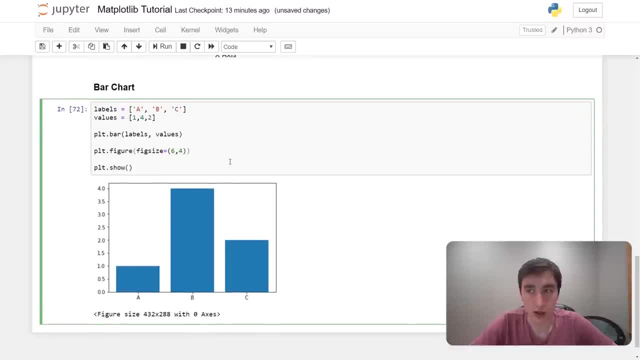 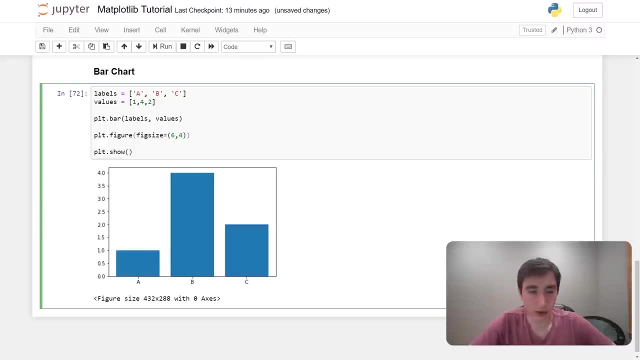 And then one thing that's cool that you can do with bar charts is you could add different patterns to these. So to do that and you can really play around with the documentation, do all sorts of different things. I just am kind of following. 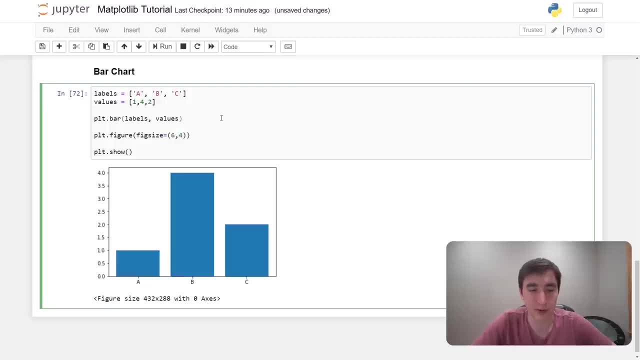 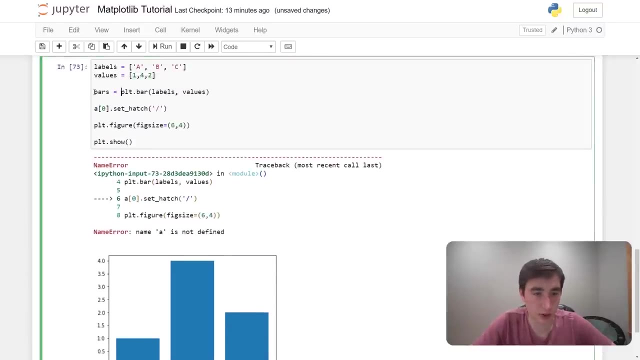 the graphs that I was showing in the intro of my video. So I wanted to just show kind of what different hatch values look like. So I can make the first one have, I'm going to say, bars, equal plot dot bars. There we go. 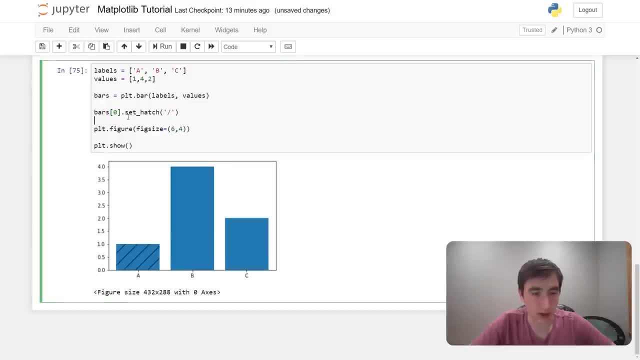 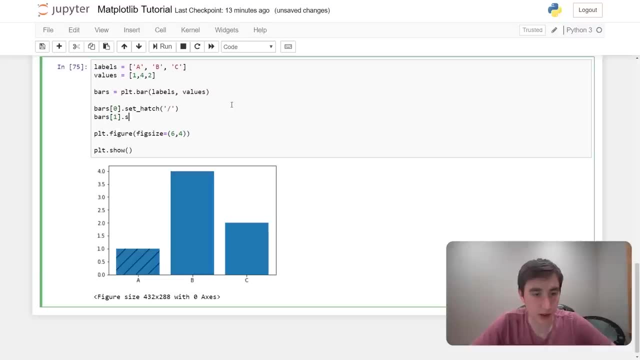 Now I do bars, zero, set hatch. That's going to give me the lines that you see down here. I can do the same thing with the second value. Let's make this circles And you can find all the hatch values in the documentation as well. 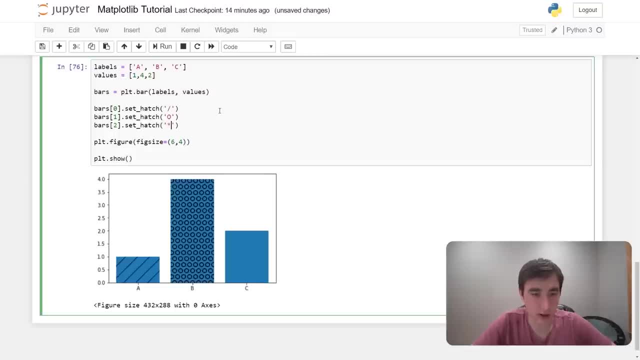 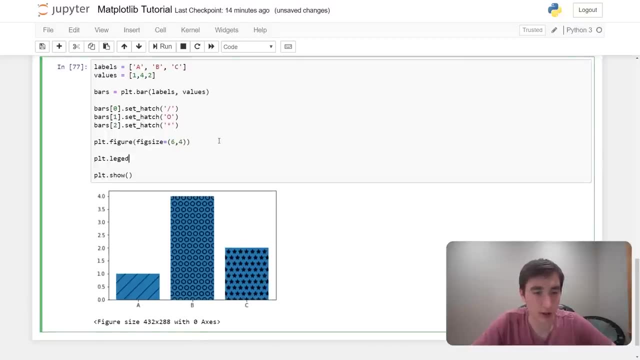 Let's do the third value. We'll do stars. So now you get kind of a cool little bar chart. I can also add a legend to this very easily, And this will tell me right away that we have A, B and C. 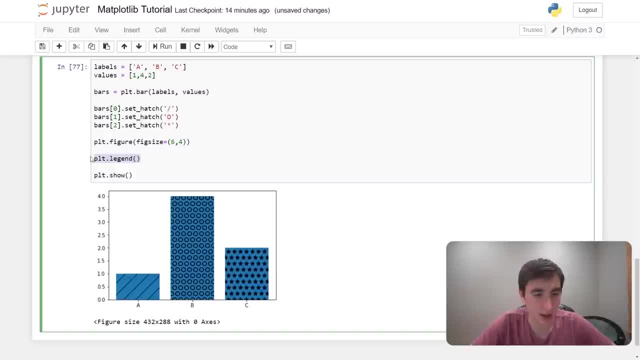 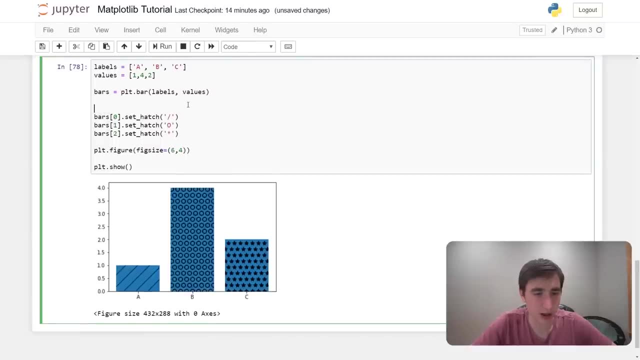 But I mean, they're labeled right here, So a legend is probably not necessary in this case. All right, Let's see What else did I want to do with this. And then, if you wanted to make this a little bit neater, 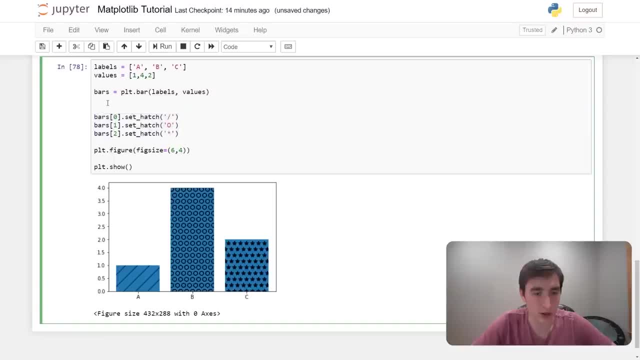 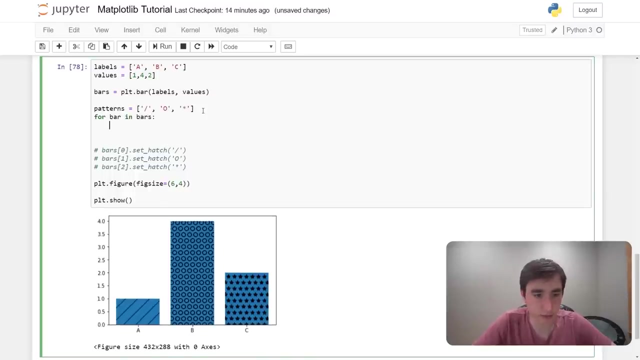 if you had like many more, it might get tiring to do this. So you could do something like patterns equals slash, O and star And you could do instead of this notation you could do for bar and bars: Bar dot set hatch. 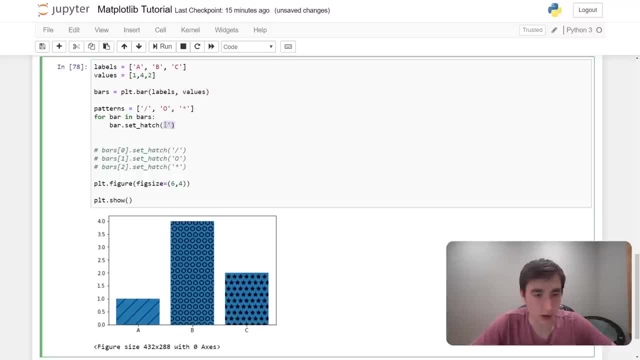 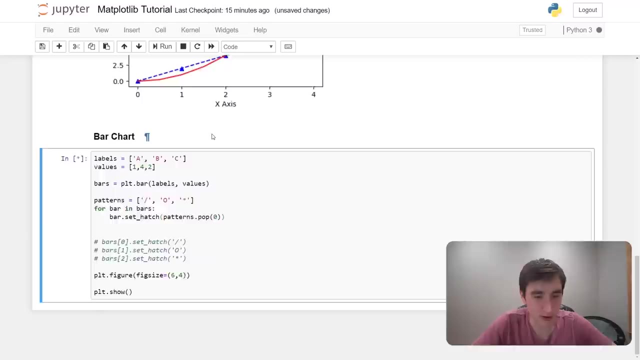 I guess we want an index as well. We'll just do actually patterns dot pop first item off. So this will get us our right one for each one. It should. Yeah, look at that. If I did pop regular, I think it would take off the last. 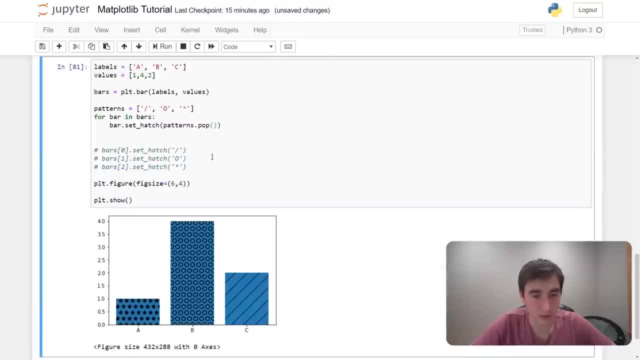 So this will be stars instead of Yep. Look at that. Yeah, So basically what it did, is it just popped off the first item for the first bar, popped up the second item for the second bar and then popped off the final item for the third bar. 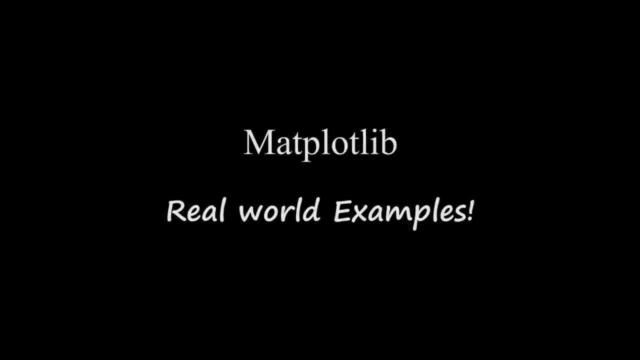 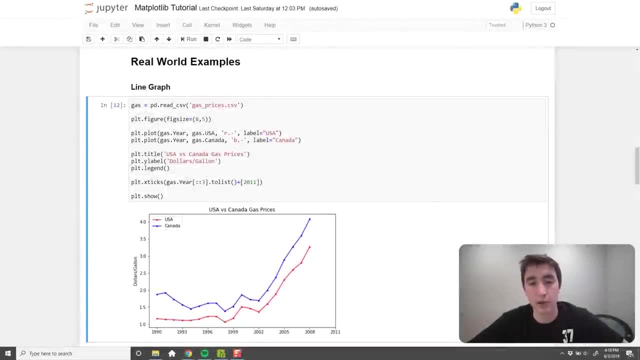 As you can see there In this video we're going to build off of what we didn't in the last video, which was kind of an introductory video to MatPot lib library of Python. So in this video specifically we're going to be kind of doing some real world types of things. 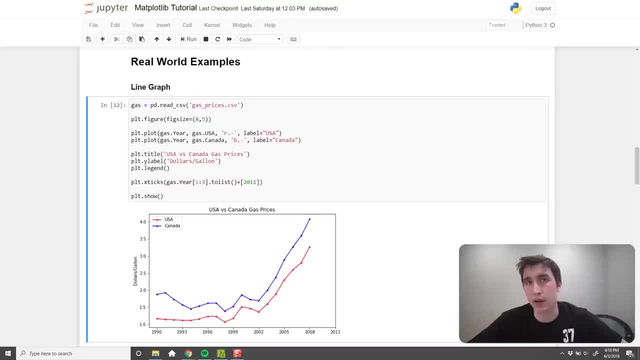 We're going to be doing some real world type examples, So basically combining our knowledge of the pandas library with the MatPot lib library to create all sorts of different plots based on CSV style data. So we'll start out with a spreadsheet that I'll provide on my GitHub page. 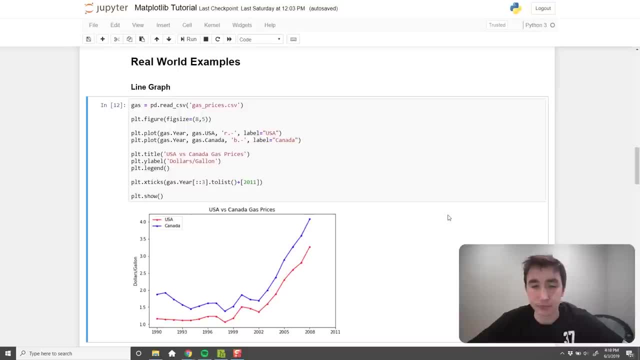 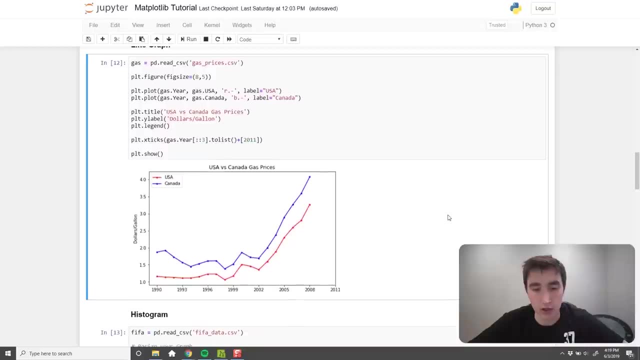 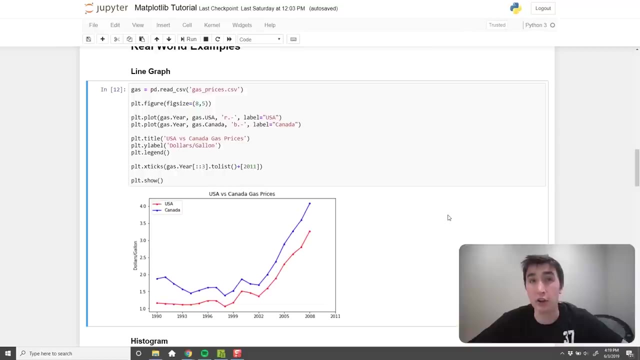 link in the description to gas prices over time for different countries. So with that data sheet we'll build charts, which is the one you see here. Then the second data set that I provided is a list of all of the game, the video game. 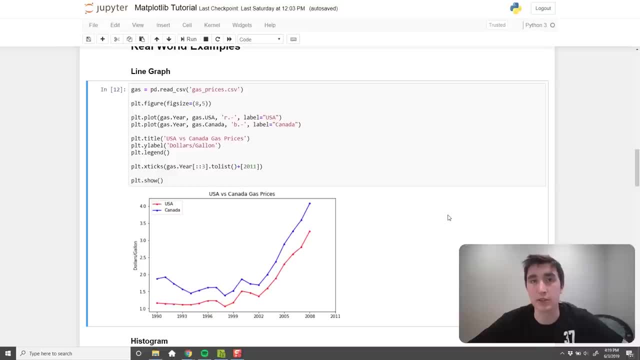 FIFA's player stats. So if you're not familiar with that, basically all of the soccer players or I guess, if you're an international viewer watching this, all the football players in the game. FIFA provided all of their like overall stats in the game. 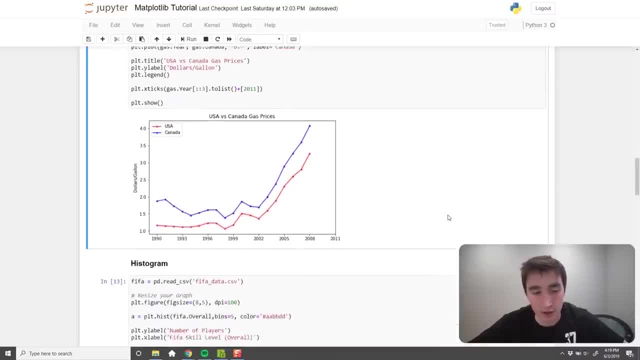 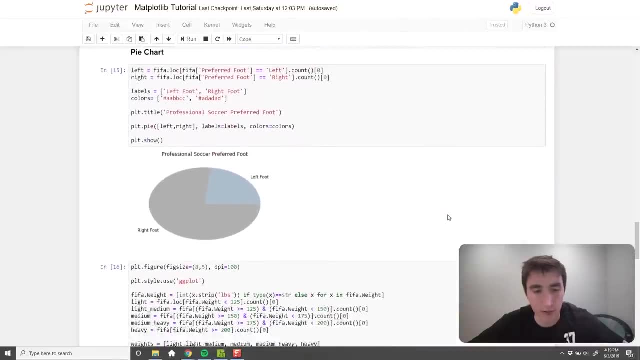 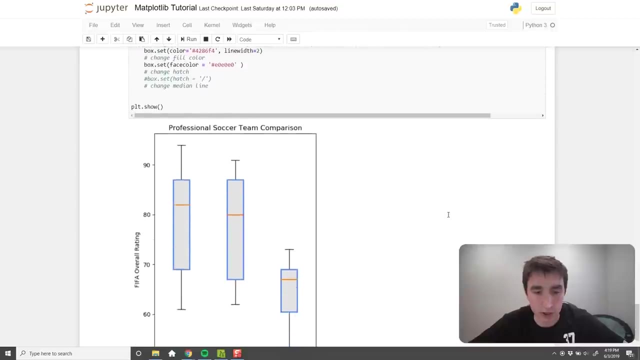 And we'll build graph, all sorts of charts off of that. So we'll do like histogram stuff with players all rating in FIFA, some pie chart stuff, more pie chart stuff a little bit more complex, And then finally some box and whisker chart stuff based off the FIFA data. 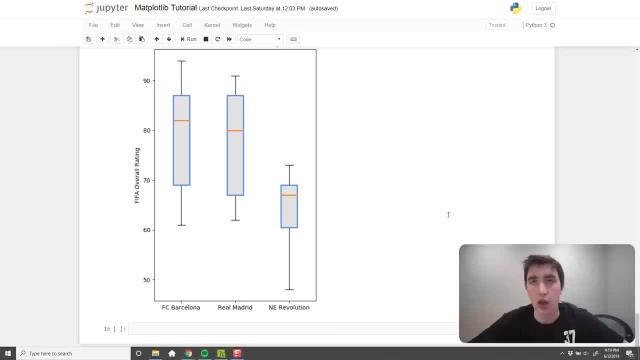 And, if we have time, maybe one or two more graphs. Before we begin, a couple quick, I guess, announcements. First is if you've enjoyed any of my videos, it'd mean a lot to me if you can subscribe, And also along the same lines. 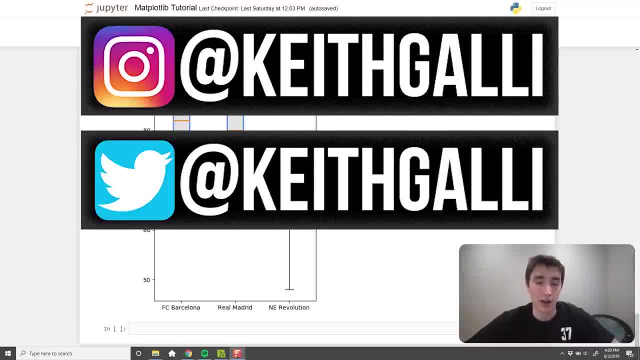 if you don't mind, also following my Instagram and Twitter. Basically, the more followers I get on all my social media platforms, the more content, the more serious that I'll take this and the more content that I'll produce. All right. 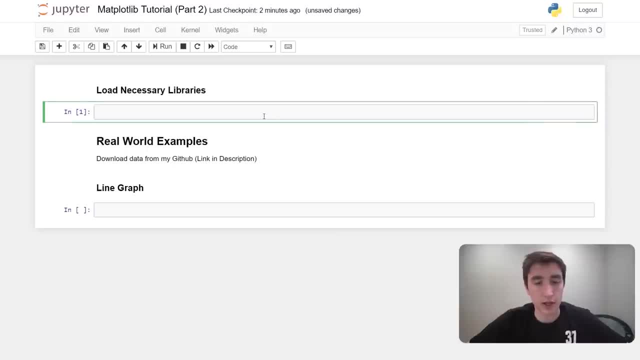 we'll start this video off the same way we started the last video. Make sure you load up the necessary libraries. I'll be editing with Jupyter Notebook using Python 3, but you can be using other IDEs and text editors as well. 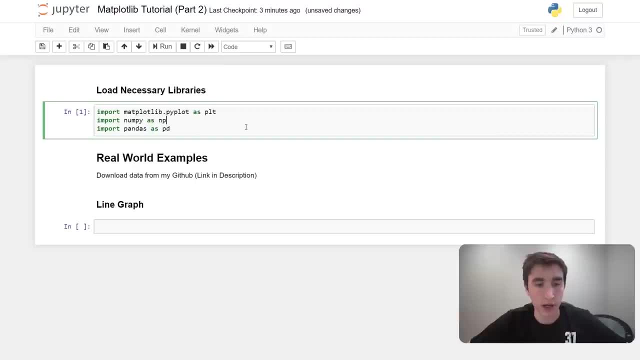 So we're importing these three libraries- Plotlib, NumPy and Pandas- Then the next step will be to download the data that I provided for this. So to do that, go to my GitHub, which is in the description, and we want to download two different files. 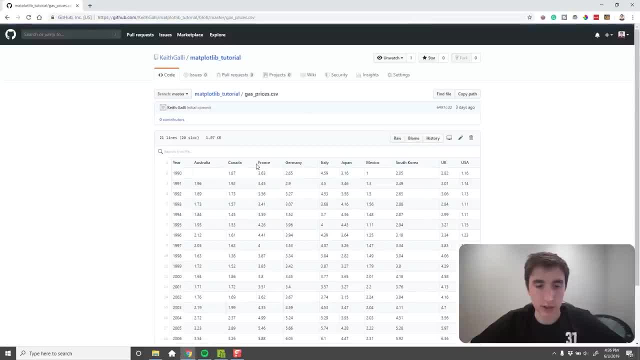 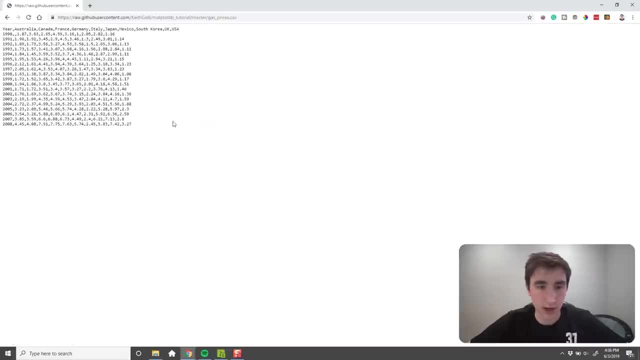 So the files. the first file we want to download is this: gas prices. So the easiest way to think to download this is go to the raw and then just do, save as you can And you want to save it wherever you have your. 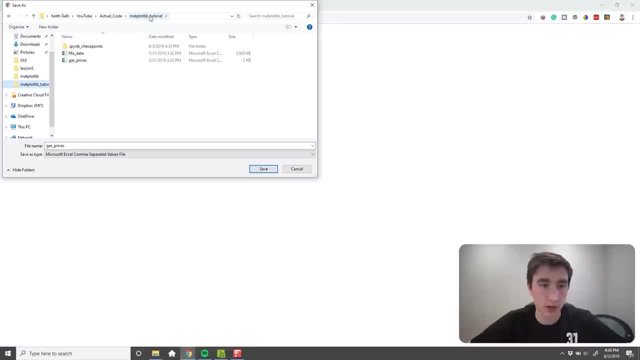 your code, So my code. these Jupyter Notebooks for me are in this matplotlib tutorial directory, So I would save this value here. As you see I already saved it. And then for the, the other data file, the FIFA data set. 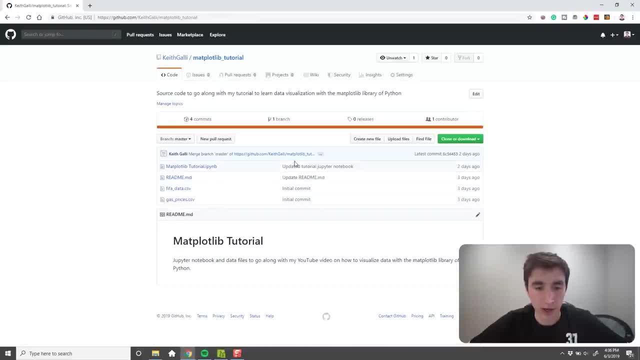 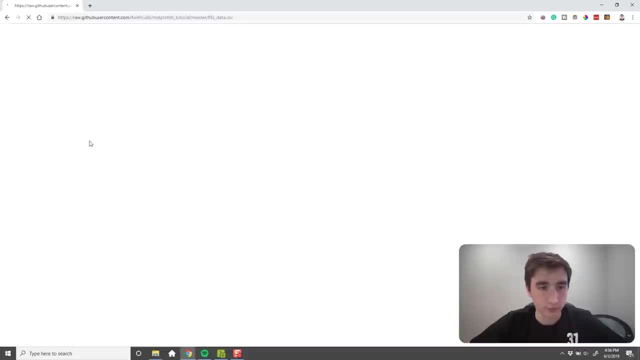 we're going to want to do the same thing. So go back to the main file. in the GitHub, click on FIFA data. This one you can't even preview, but just click view raw, right click and save as. uh, save it as a CSV file. 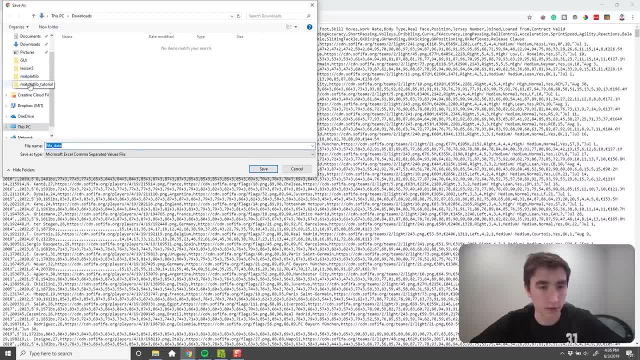 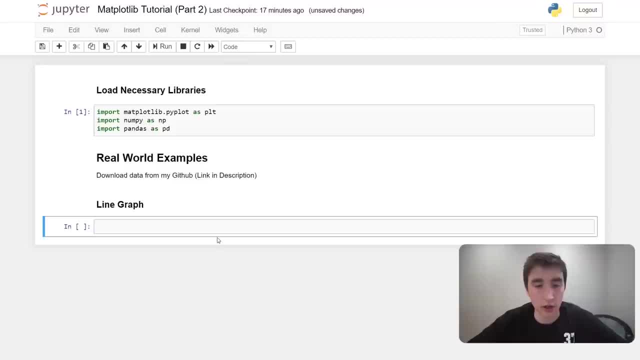 So a comma separated values file, And you'll also want to save this in the same directory that you have the file that you're writing your code in. Okay, So now that we've saved the data, let's start playing around with it. 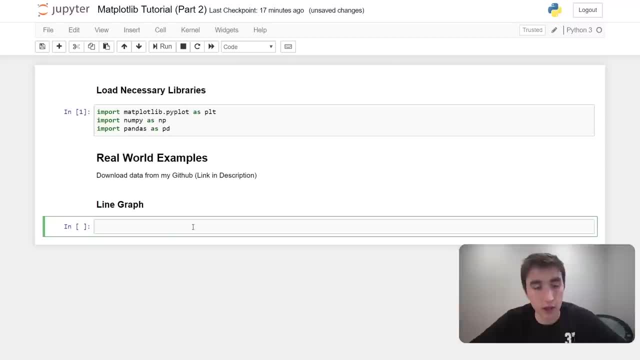 And if you remember from my pandas video, the way that we can look at a CSV file with pandas is we can do something like: we'll call the CS or we'll call our data: gas equals PD, dot read CSV. Then we need to type in the name of the file we want to read. 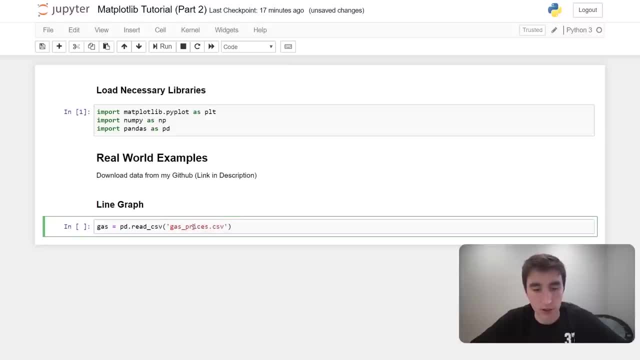 We've saved it as gas prices dot CSV and we should be able to run that No issues. And we saved this file in the same directory that this mat pot lib tutorial file is in, So that's why this worked If you save this file in a different directory. 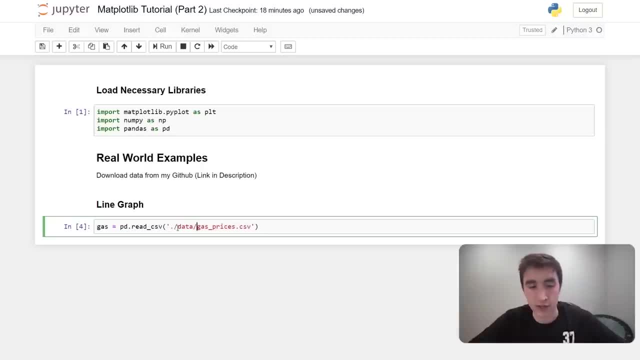 you can um specify where you saved it. So if you save it in like a data folder, you would specify it such uh type of syntax. Okay, Gas. So now what we can do is look what to see what's in our 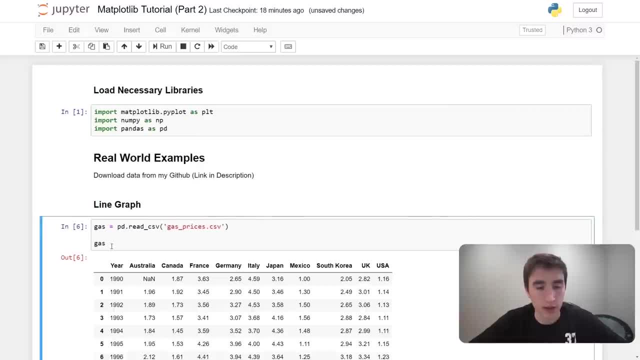 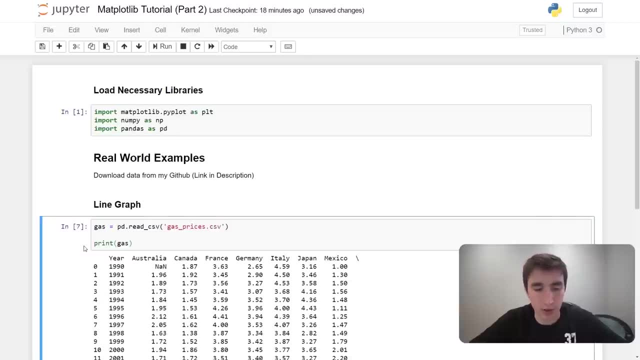 um, this data file. So if I just do gas and this works in Jupiter notebook but in another, uh, if you're just using like sublime tax, you'd have to like print gas, Um, or you could just be looking at the actual CSV file in like Excel. 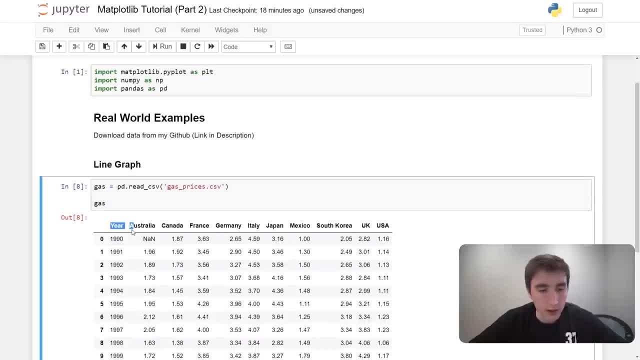 So gas we have year, and then we have all these different countries And their price in us dollars per gallon for gas that year. So the way I look at this, we're going to have year as our X input, So ah. 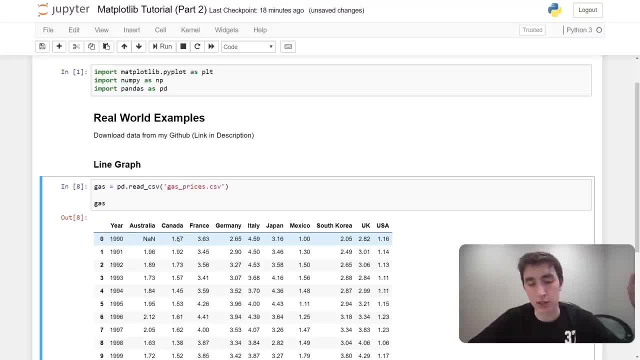 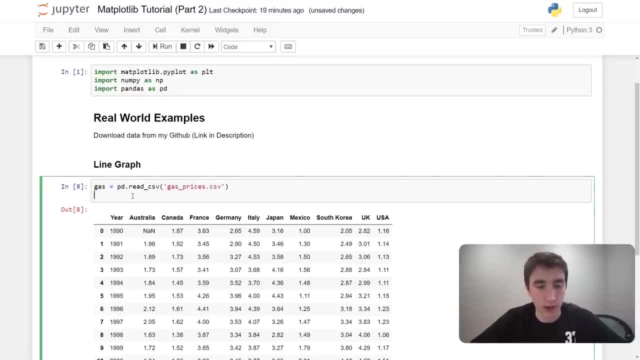 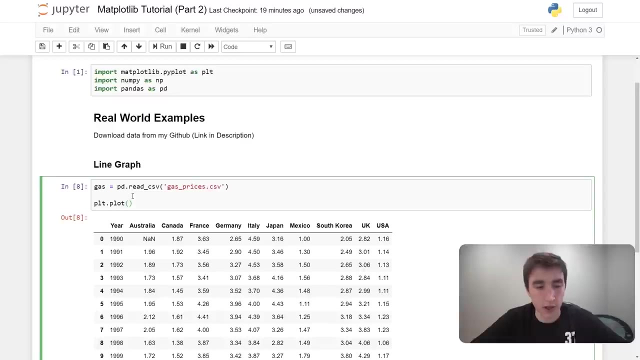 stop texting me. So, based on the year, each country has a different gas price. So the way we can access that is we can do something like PLT dot plot, And so our X data is going to be gas dot year, Our Y data is going to be 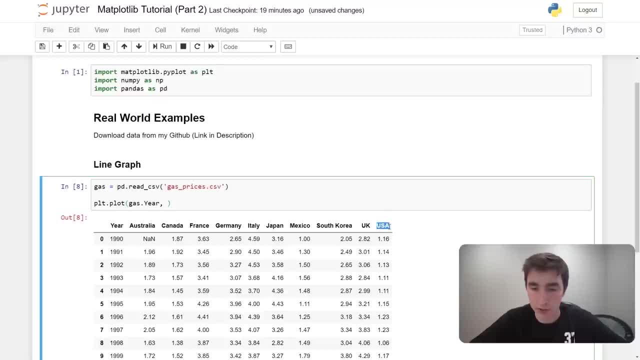 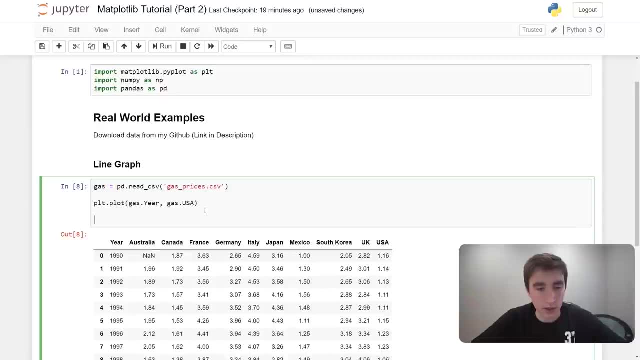 let's say we start with USA, So USA is all caps here. So I have to follow that same syntax when I'm accessing that gas at USA, And then I can do a plot dot show And I think already there we'll have a basic graph up and running. 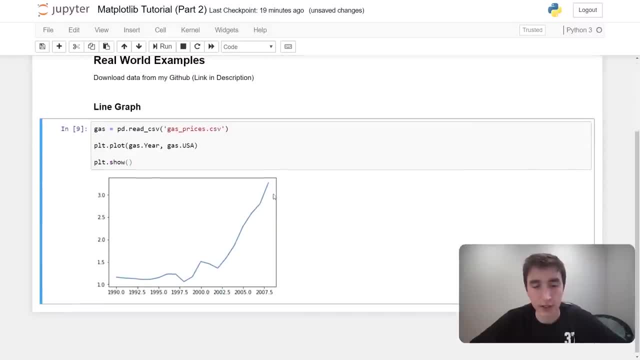 So, as you can see, yep, this is the basic graph for our data, And we could also add another country. We could do plot dot plot. Let's add Canada year gas dot Canada. I think, yeah, as you can see. 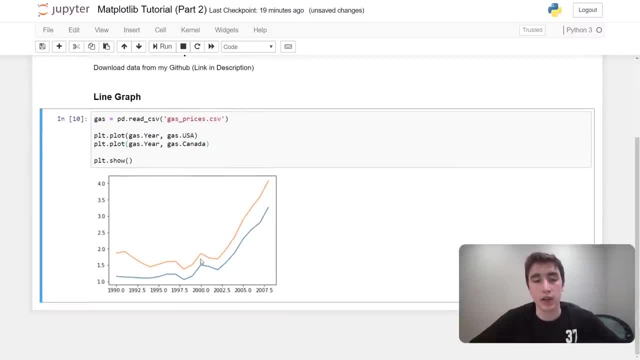 now we have two different graphs And, as you can see from this um, it's easy to see- more easily than just reading the CSV- that, oh okay, Every year gas in Canada is consistently higher than in the USA, So but we have some problems with this graph. 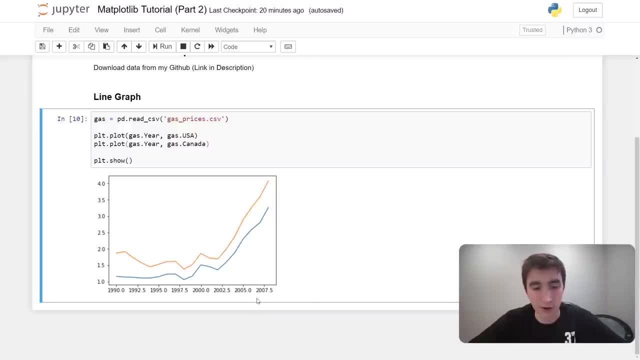 So, like one thing that I see that's an issue is all these years, like I don't know. I think it just makes more sense to be looking at the exact year, especially since this data wasn't, like, broken up by month, So like 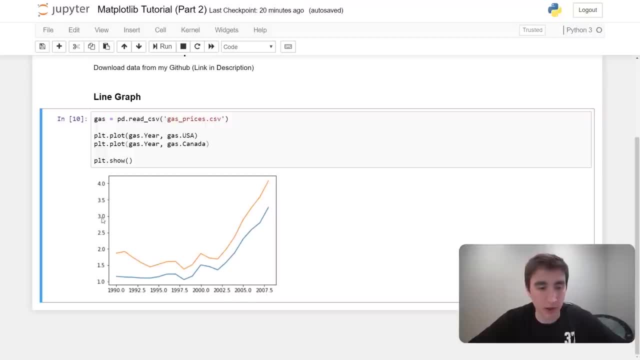 I don't like the X axis labels. We have no title, We have no real good indicator of what these values mean over here on the Y axis. So we need to start fixing some things up And quickly to note if you have like a multi word. 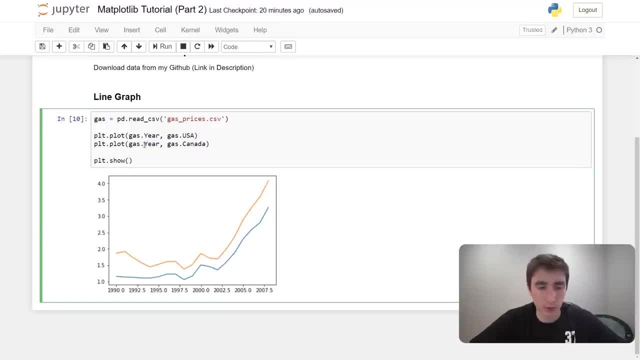 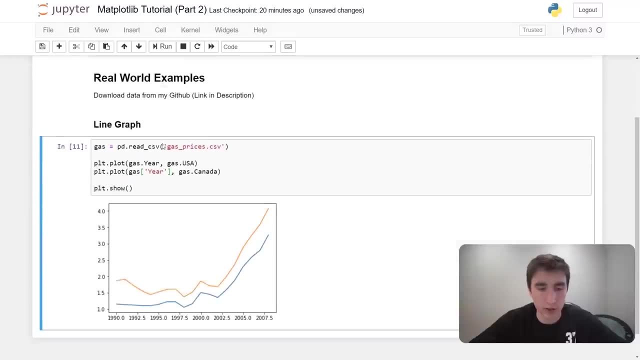 name. this format of dot year probably won't work, So you could also do bracket notation to access that field. As you can see, it still works. So if we had something with two names and I don't remember, let me look at the data again. 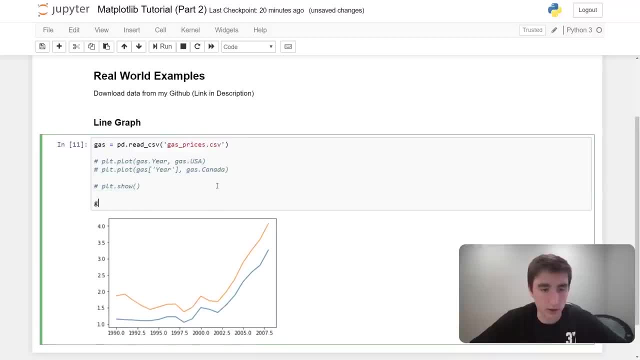 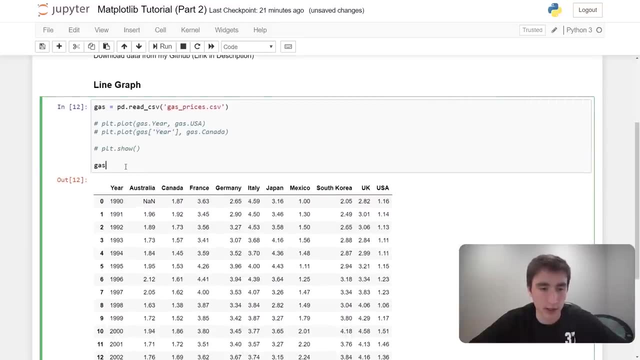 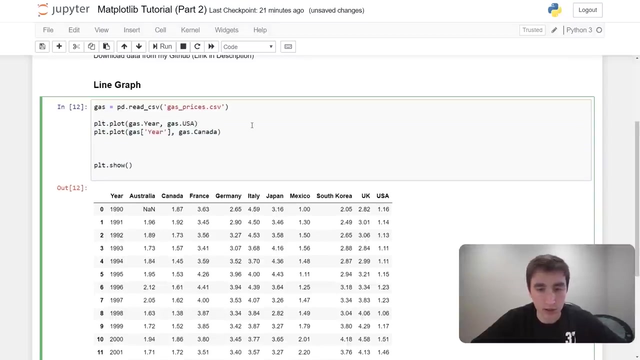 see if any countries have that- uh, South Korea, for example. like we would have to use this syntax, So I'll actually plot South Korea's um gas in this list, their gas prices. So plot dot, plot gas year, gas dot South Korea. wouldn't work. 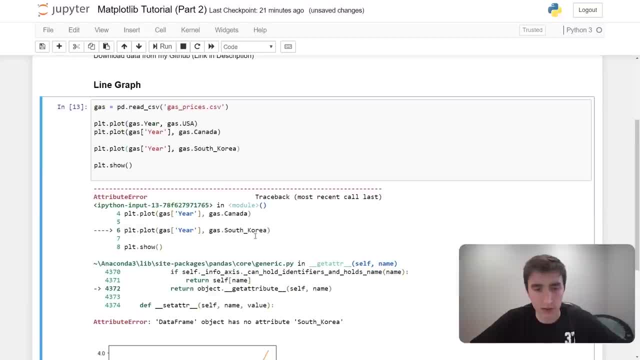 Maybe actually it would work with the underlines. I'm not sure. Yeah, South Korea is having issues, So what we can do is South space Korea. Now we have three lines and, wow Yeah, The gas in South Korea is even more expensive. 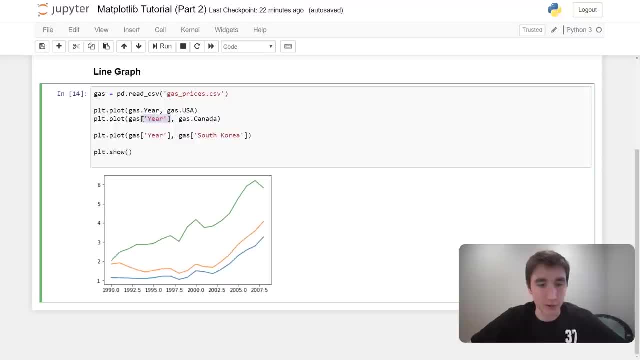 Okay, It's just kind of bothering me mixing these different ways to do this, So I'm going to change this back to year, changes back to year and only leave South Korea like that, Cause it kind of has to be like that, Okay. 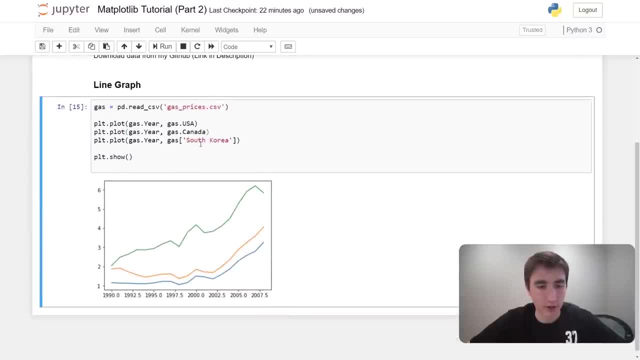 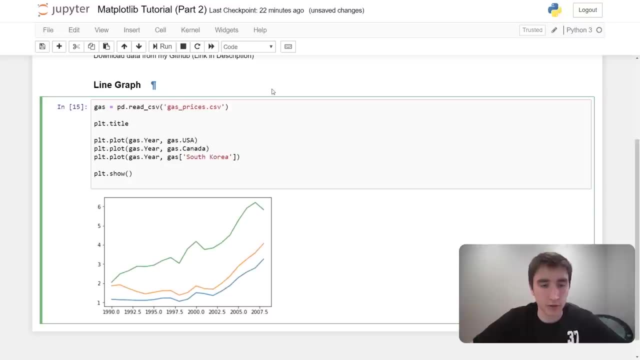 So now we have some plots. Let's make this uh graph overall better though. So to start, let's add a title. So to add a title, if you remember from my last video, and feel free to review that again, we can just use PLD. 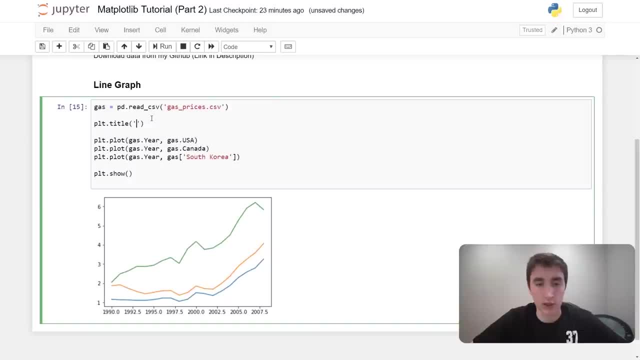 dot title. I can label this like gas prices um over time and us dollars, And so it still doesn't make too much sense because you see all these lines but you don't know what they represent. I mean, we only know that what they represent because we see the code here. 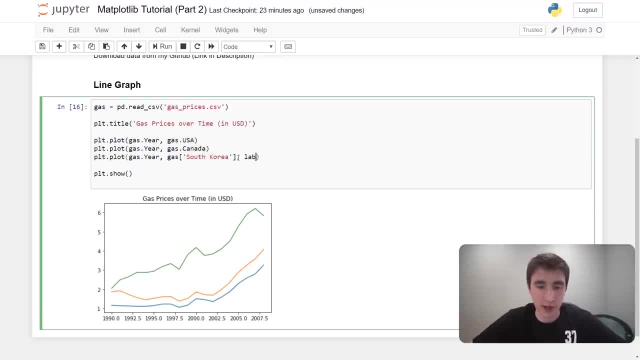 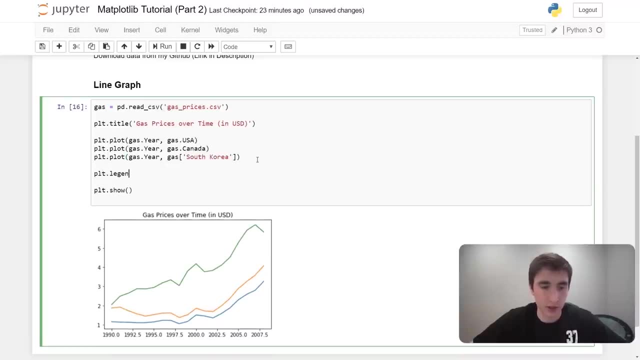 but we should add a legend. And so to add a legend- we're not the first- give these plots labels, because if I don't give these labels, watch what happens. Plot dot legend. Oh wow, It worked. I was not actually expecting that to work. 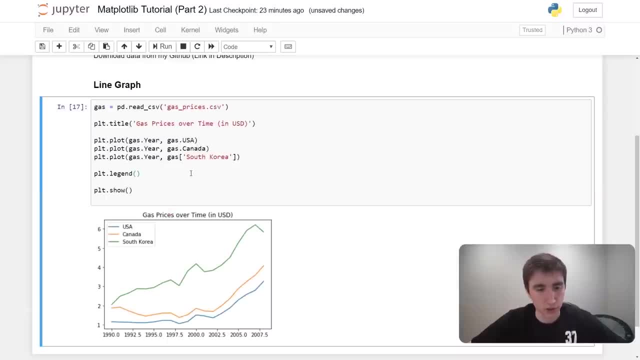 Um, I'm trying to think why that is that it worked whatever It worked, without needing to add the labels specifically. Uh, so that's kind of nice for us, I guess due to the fact that we're, you know. 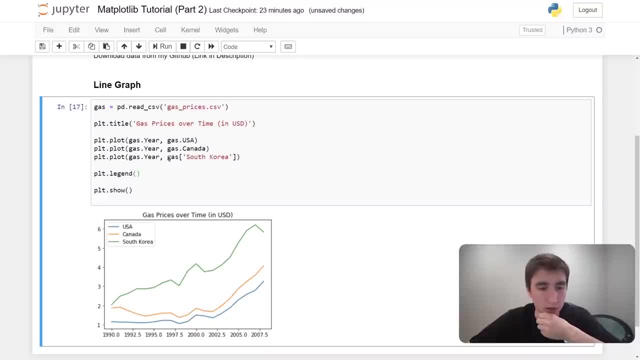 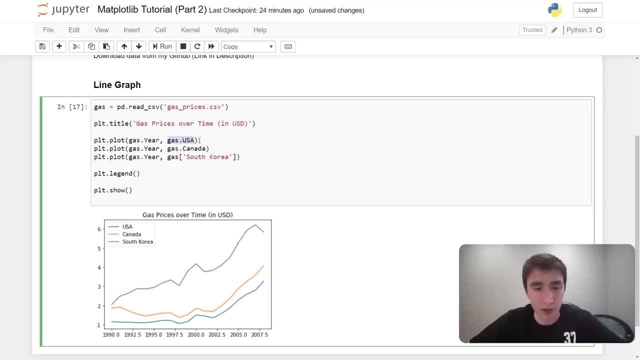 from a nice CSV that already has headers. that probably worked. But in our last video, uh, you have to add label. So I could actually change the label if I wanted to, if I wanted this to just say United States. See that? 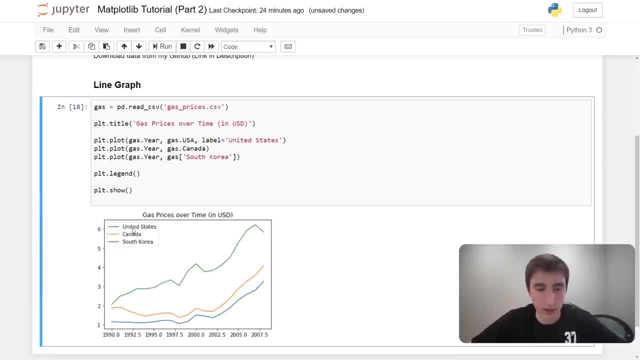 Change it like that So you can add this option or label parameter If things aren't working for you properly. but for us it just kind of magically did the trick. Okay, So this is looking already a little bit better. I might make the graph a little bit. 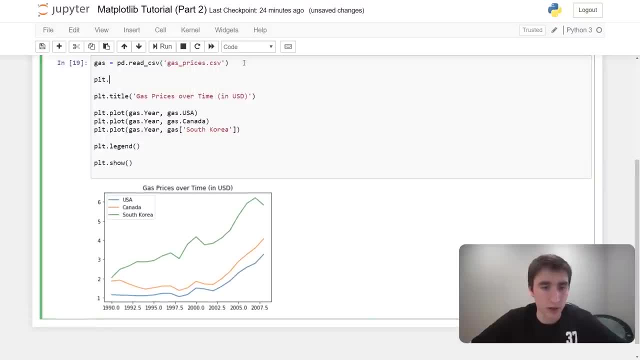 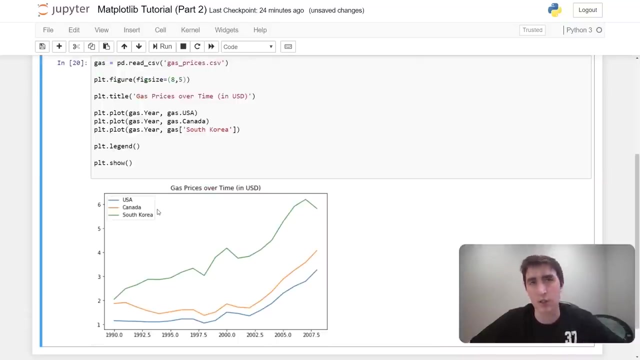 bigger. Let's do that I can do plot dot figure. Fig size equals, say, 8 by 5. So that's a nicer size. I think it's more easy to see everything. The legend is a more reasonable size in comparison. 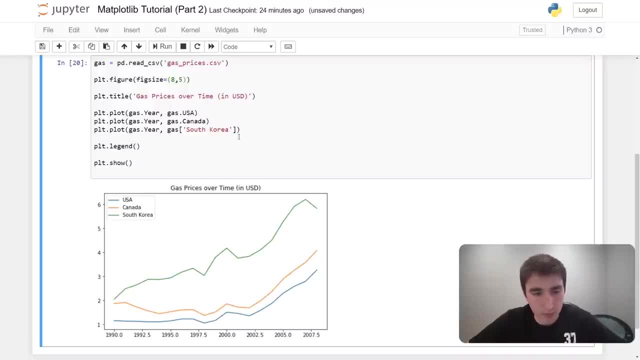 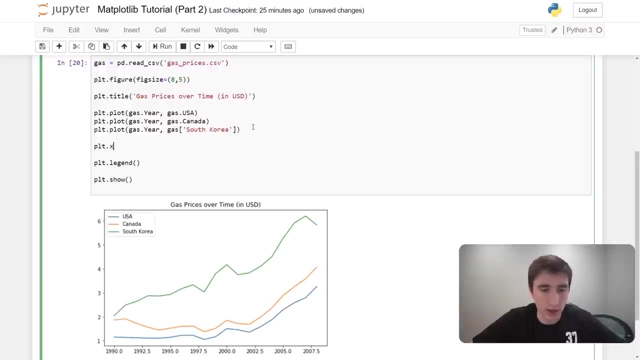 of everything in there, So that's a bit better. What else can we do to this? Well, we don't have any labels for axes, so we should definitely do that Also. I really don't like that. these tick marks are not exact years, So I think the next thing I'm going to do is change up the ticks. So 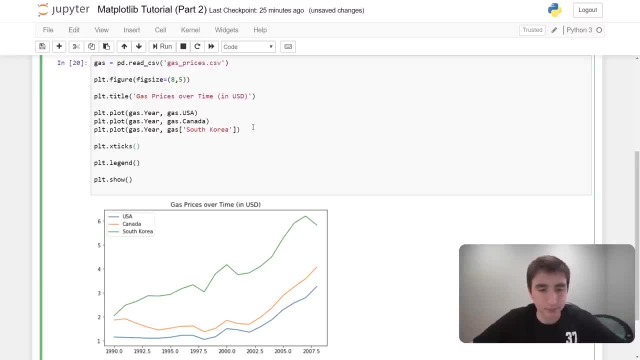 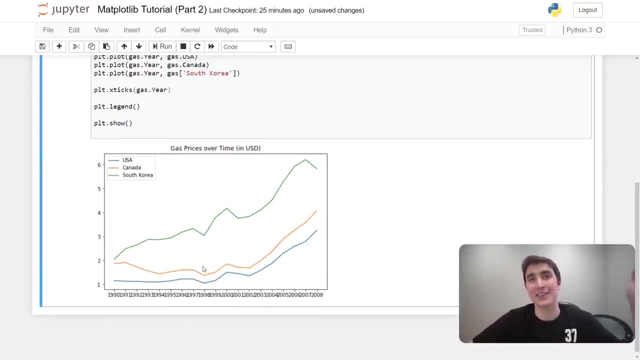 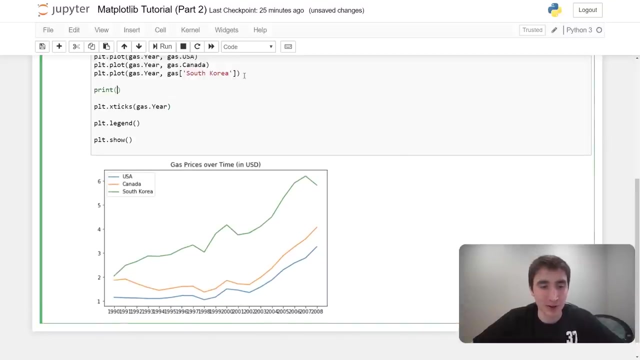 x ticks. What we can pass in is just the year here, So now it will have a tick for every year that we have data for. Wow, and that looks absolutely fantastic. Yeah, obviously issues with this Two squished together. So what can work well is, if I print out gas dot year, you see we have part of a panda's. 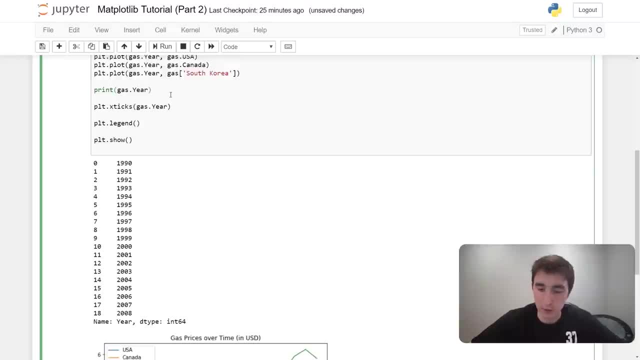 data frame. but we have every one of these years, If we remember, some good old list comprehension but list Iterating syntax, maybe that would be the word. But you know, when you want to get certain items, like the first five items on a list, you go zero to five or you could even just do five. 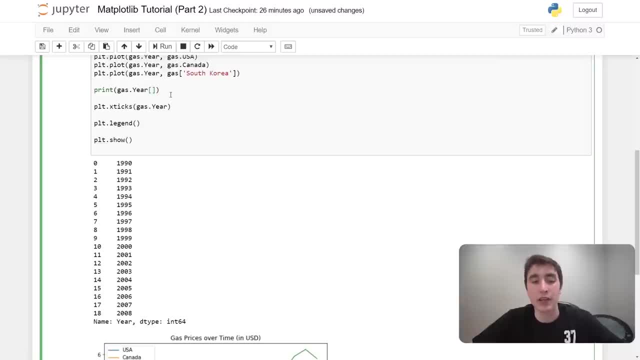 What we want to do is iterate, you know, maybe take every three years. So what we could do to do that is we don't care where we start. So we want to start at the beginning, we want to end at the end, but we want to skip every three years. So now we get all the years in a. we get 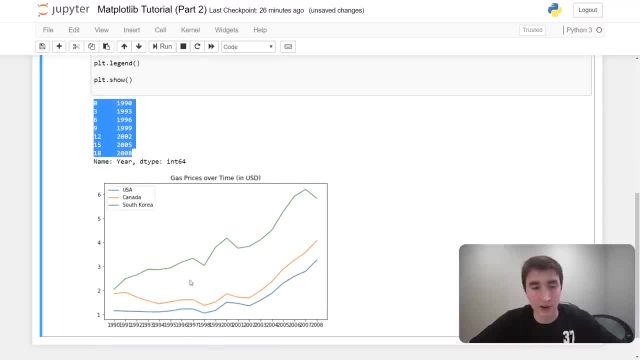 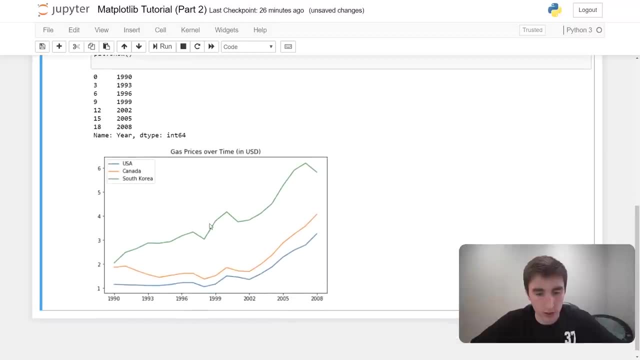 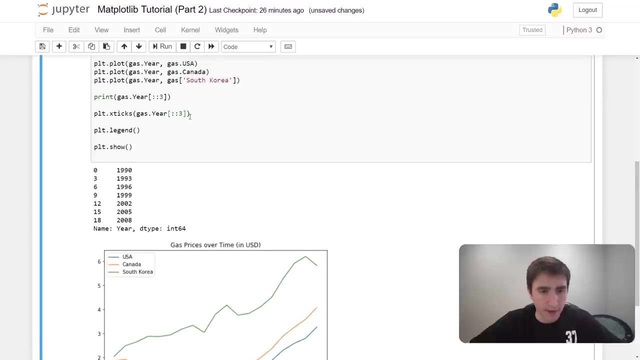 every third year, which will probably be better when we graph it down here. So I'm going to do that now. So guess, year tick, tick three, colon, colon three, Cool, That looks pretty good. All right, I also kind of would like to have exact values here, kind of show exactly where. 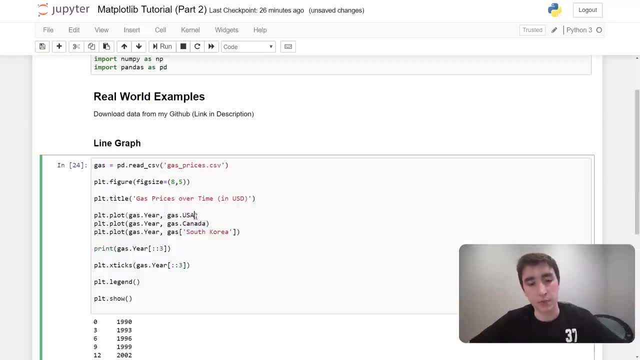 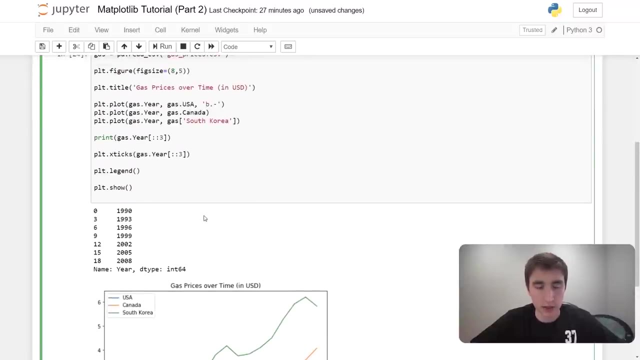 we're plotting the points So to do that. if you remember the shorthand notation from the last video, we can do stuff like: we'll make USA blue dot dash. So blue is the color and we want a dot dash, We want dot markers and a dash, a straight line. That's basically what we're saying. 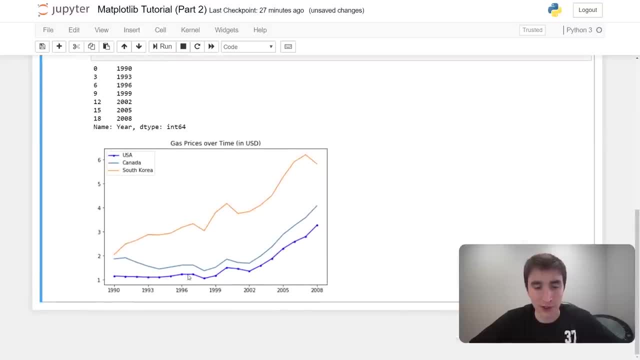 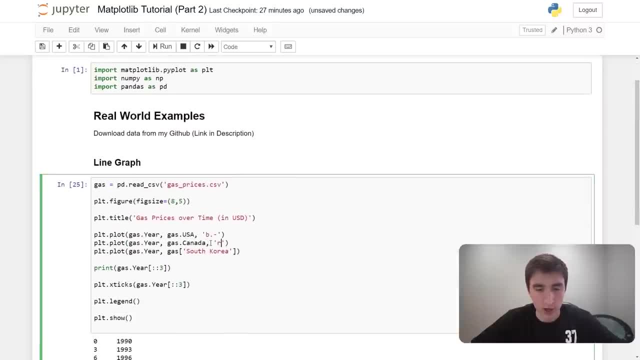 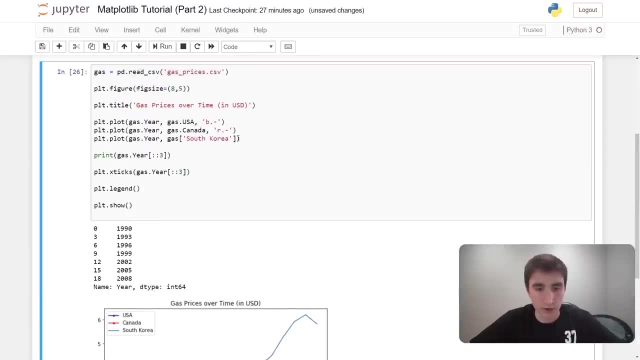 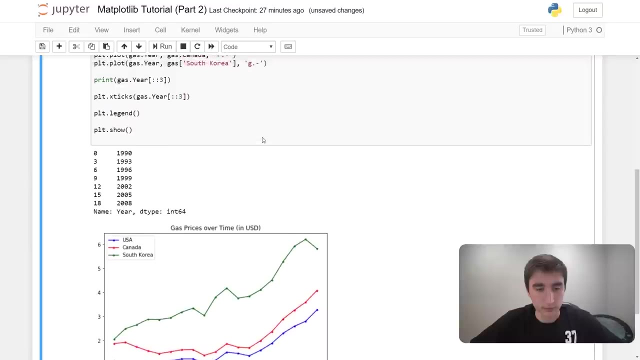 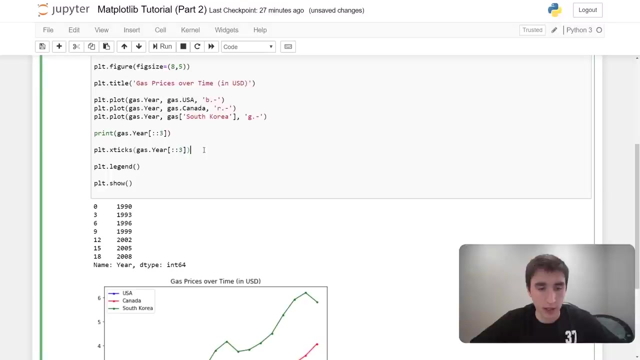 do the same thing for the other ones: Red dot dash. And what's cool too is you see that the legend changes as we do that South Korea, let's say a green dot dash. Cool, I like the look of this. Still, we need to do some more modifications. Let's add labels to our X and Y axis, So X label. 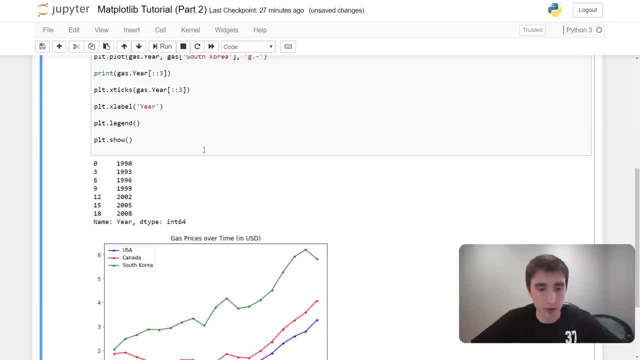 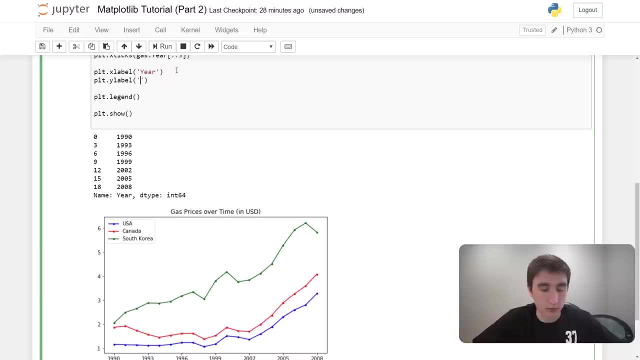 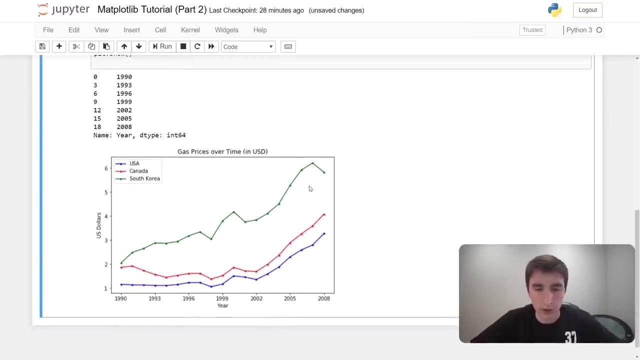 will be year. That's pretty self-explanatory. Then the Y label will be US dollars- Cool, So now you can see. you know, okay, And year 2008,. South Korea paid approximately $7,000 a year, So that's. $6 per gallon of gas. We're all translating all these values to US dollars, While Canada paid about $4 and the US paid about $3. So that looks pretty good to me, And we can easily add some more countries here, So I could like add Australia, for example. 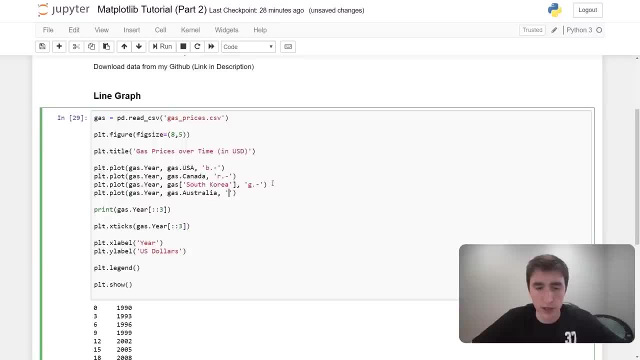 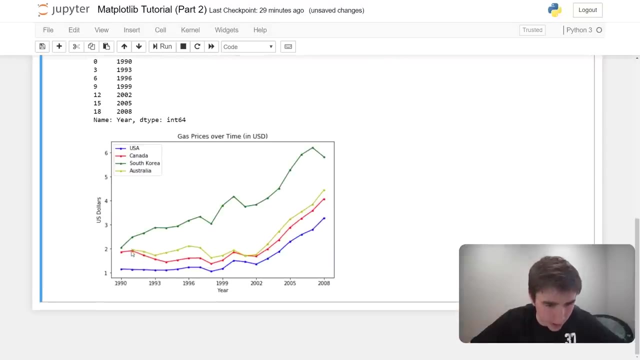 and we'll make them. I don't know what color to use. I don't know that any more yellow. Sure, It might be an ugly color. It's not too bad. but yeah, there we have Australia. It looks like they're missing maybe a data value for 1990.. I'm not positive, but yeah, we can easily do this for. 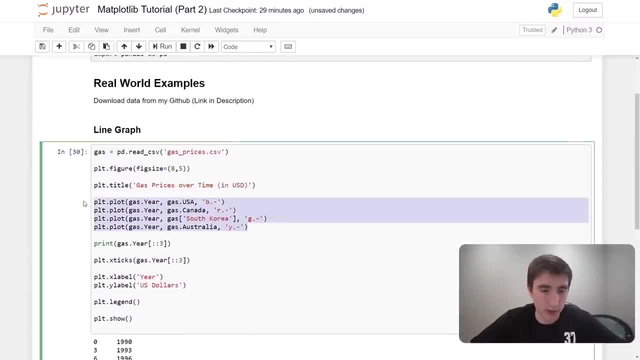 all of our different graphs And we could even do something like comment this out temporarily, Something like for country in gas, Let's see what happens at that print country. Yeah, cool, This is giving us all of the different countries We don't want year. 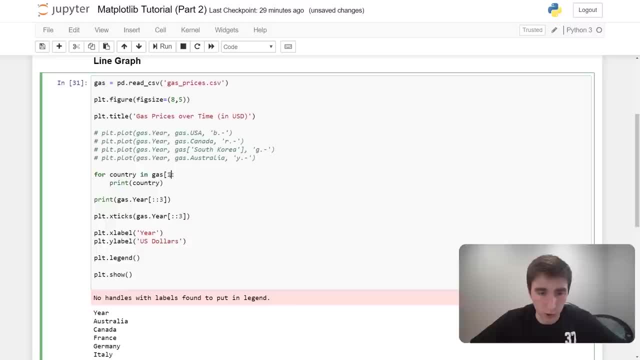 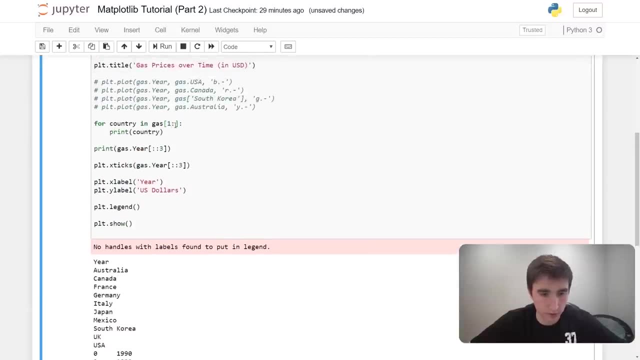 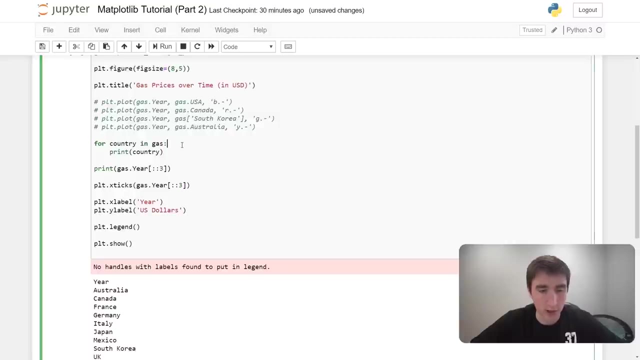 So I'm going to say in gas one onwards. Now we have, oh no, Close, close, close. Okay, I'm going to be a little bit hacky here. If country is not equal to year print country, Now we get all of the countries, And so what we could do with this now. 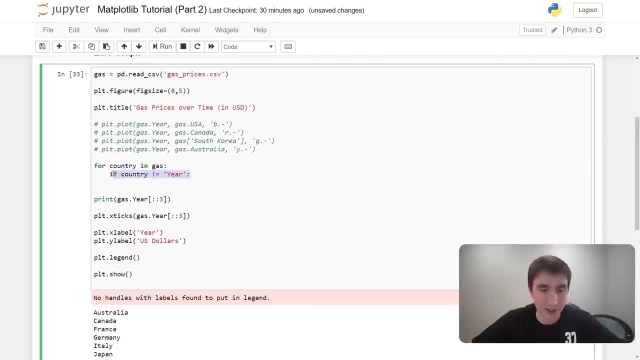 is. you know, there's probably a little bit neater of a way to do this than if country is not equal to year, But I'm just trying to show you how like we can do this very quick and uh, efficiently Do gas, dot, year and then country, Uh, and we'll let it self-select the colors. 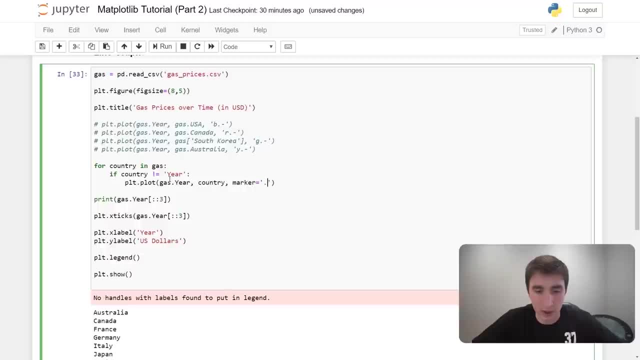 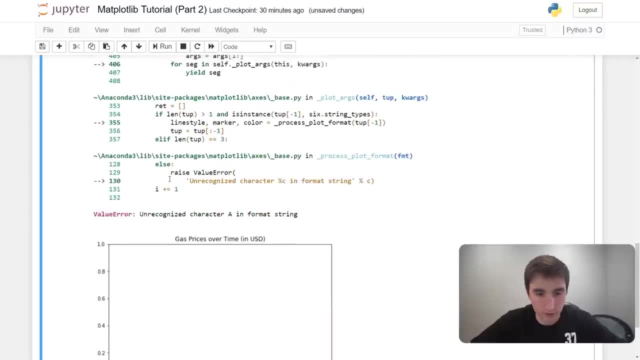 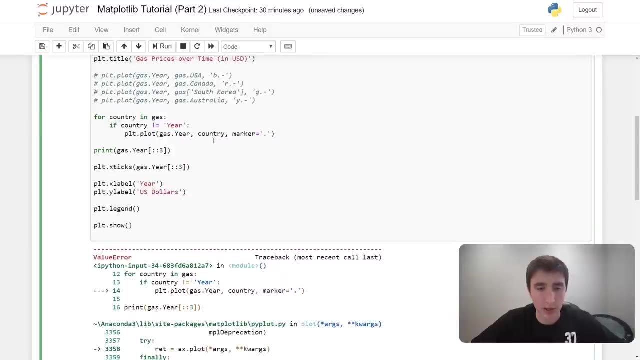 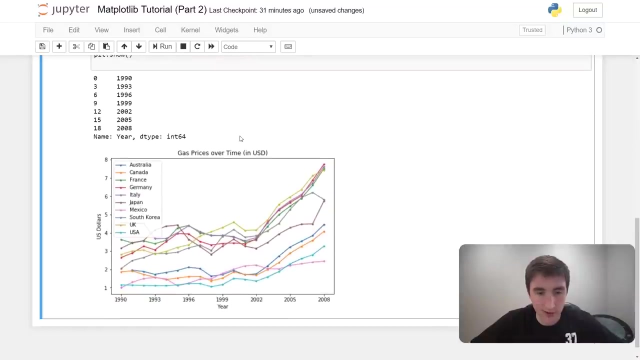 But we could, if we wanted to specify. marker equals dot and I think the line style will be fine already. Oh no, Unrecognized character in. oh okay, Can't just do country, We need to do gas country. Look at that: Now we got all of the different- uh, all of the different countries in our graph. 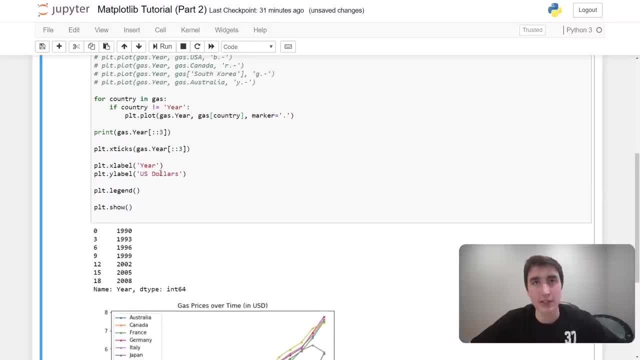 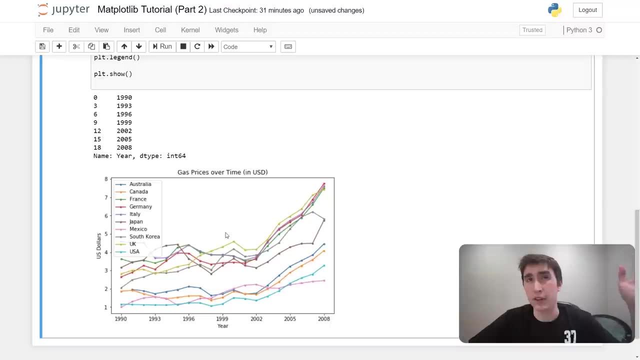 And you could move. there's ways within matplotlib to like move the legend outside of the graph. I'm not going to go into that right now, but another, I guess, comment that I have is: whenever you're doing anything with matplotlib or anything with Python in general is like, quickly do a Google. 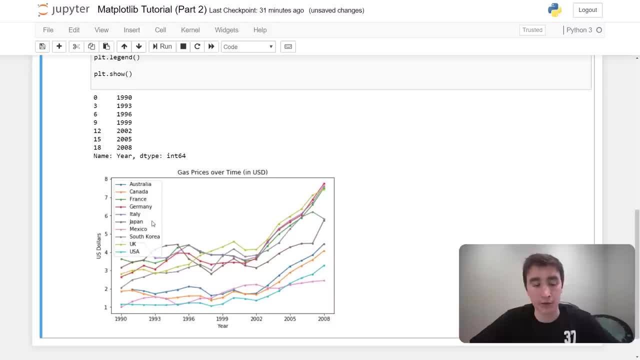 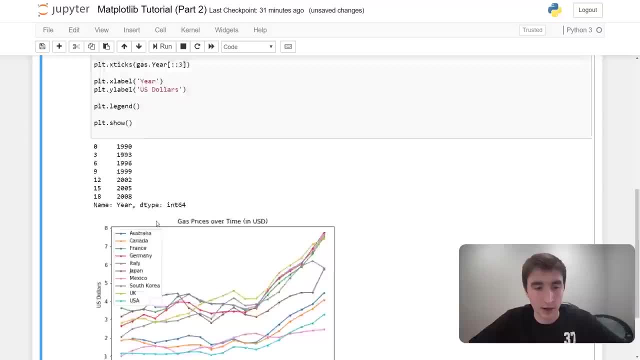 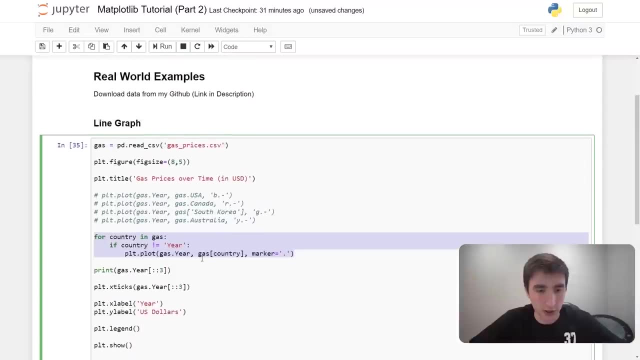 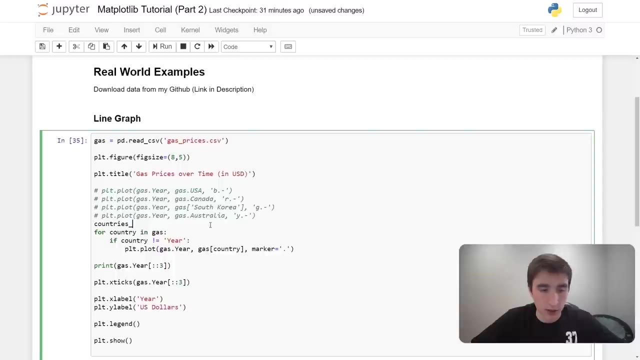 as you and found an answer to it, So I always recommend doing that. Uh, but this is kind of cool that we were able to quickly graph all of these different lines for all the different countries And, if you wanted to, you could like create a list like countries um to look at. 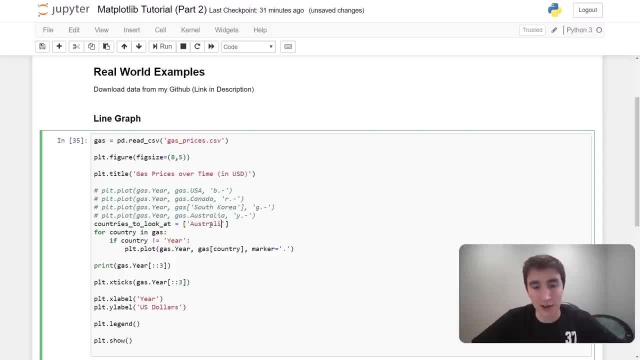 maybe not the best name and you could choose Exactly which ones you wanted to include, And then you would do if not equals year and or actually you could just do if country in countries to look at. maybe I'll do this real quick. 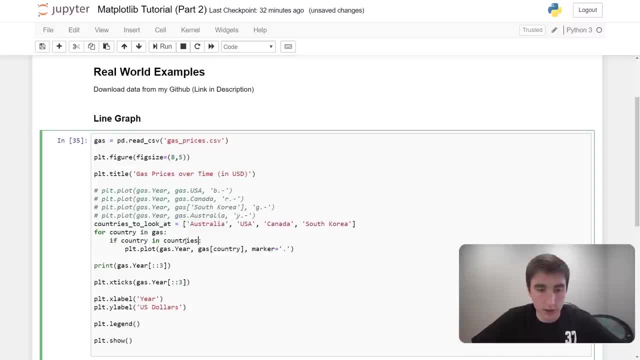 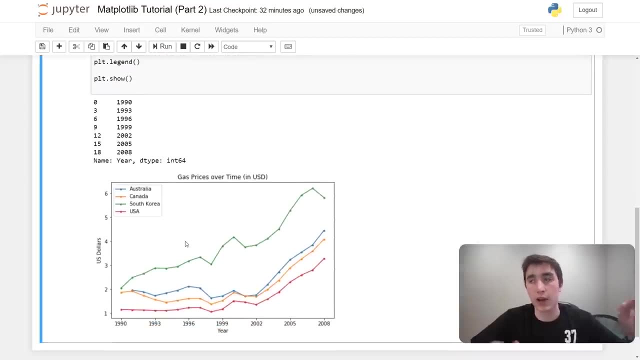 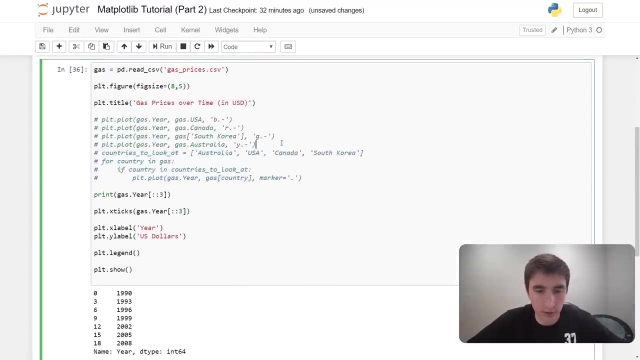 If country in countries to look. So you see, this is another way we can graph specific things. Cool, cool, cool. All right, I'm going to comment this out temporarily and just leave. I'll leave it. I'll push it to the GitHub. 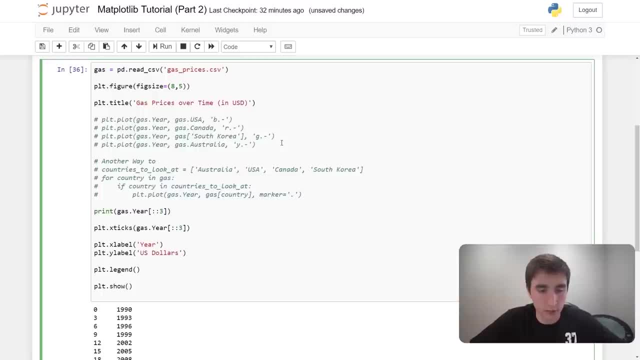 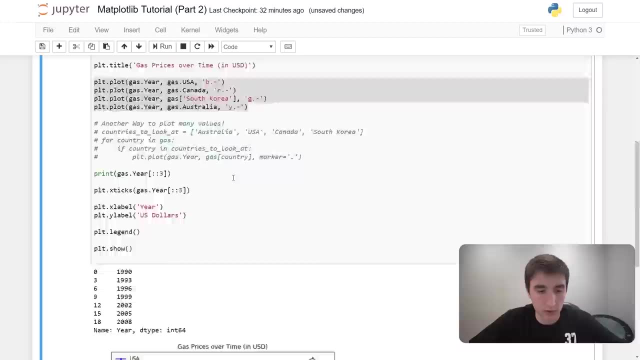 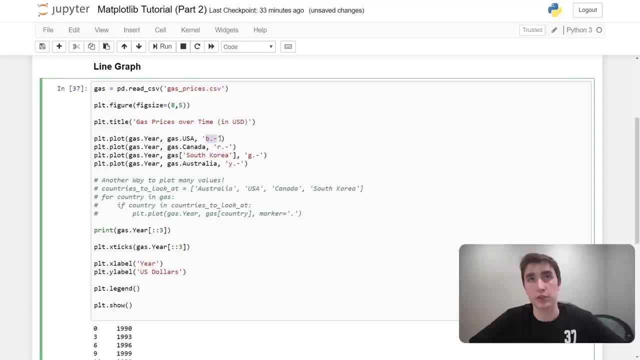 when we're done with this video and we'll uncomment this again. Cool And yeah, you can play around with this style. You can use the shorthand notation or you can use the long hand notation that we kind of used here, but you also can reference the first video. 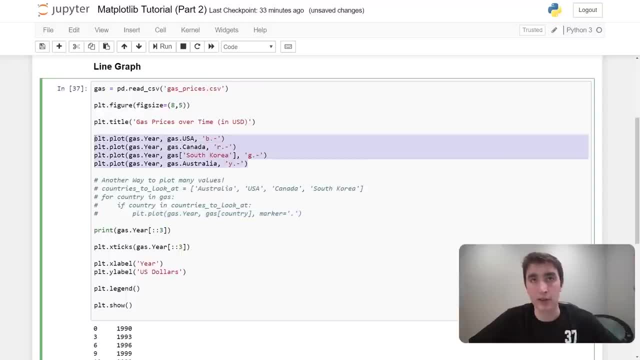 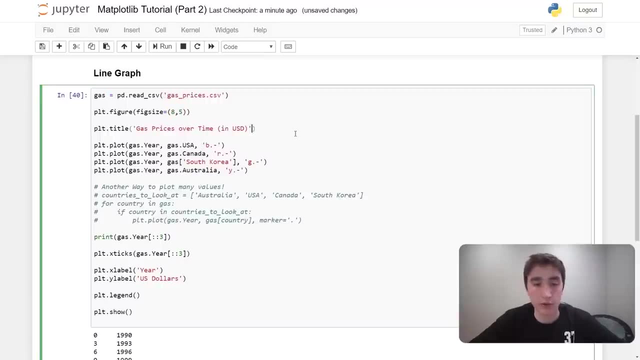 I posted on matplotlib to really play around with your line graph styles. All right, We're pretty much done with this graph, but I'll add a couple of final things before I move on to the FIFA data and doing some other graphs. So the first thing is, um, changing up the font size I mentioned. 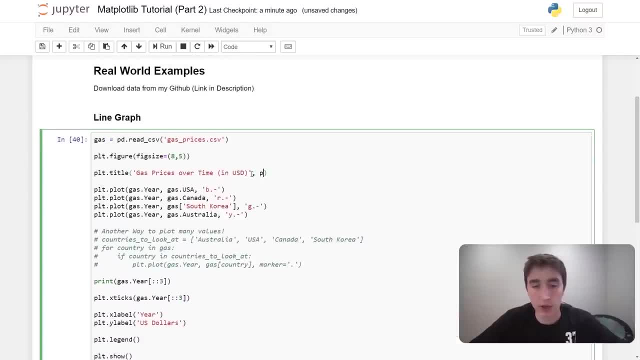 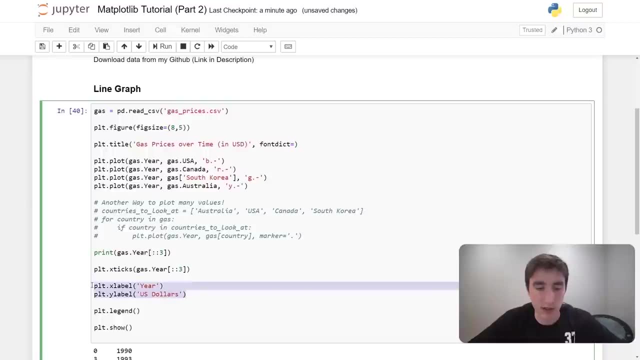 this in the previous matplotlib video I did, but, um, I'm going to go ahead and do a little bit of that. Uh, I thought I was worth mentioning again. So we can add a font stick to our title and actually we can add this to any text-based labels. So you can also add it to the X label and Y label. 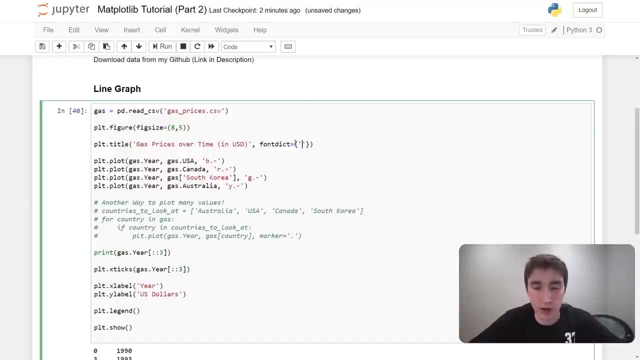 uh, and we can do all sorts of different tweaks to our font Um. I put a list in the description to all the different fonts you can use here, if you wanted to change up the actual font type, Um. but I'm going to keep the font type the same. I'm going to change the font weight. I'm going to 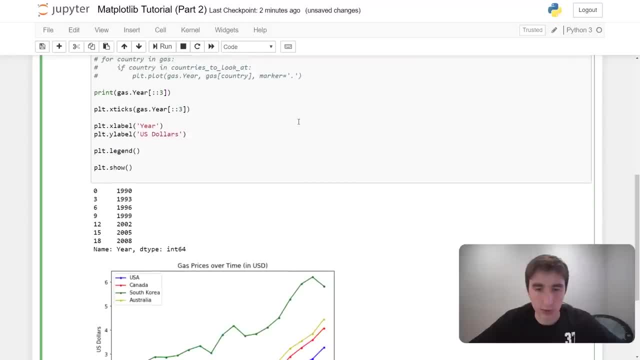 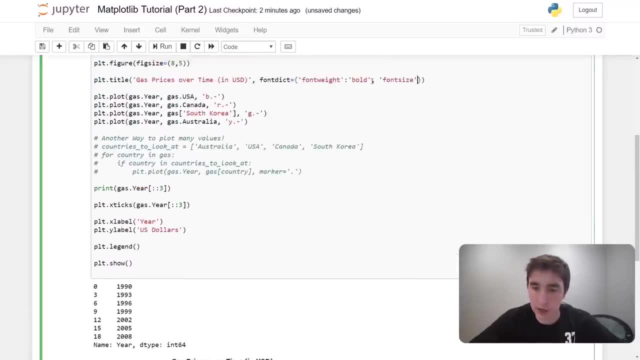 make it bold. So you see it, now It's not bold. but if I do this, watch what happens. Now it's bold. And let's say I also wanted to change the font size. I would say font size, and let's say it's size 22.. So now we have. 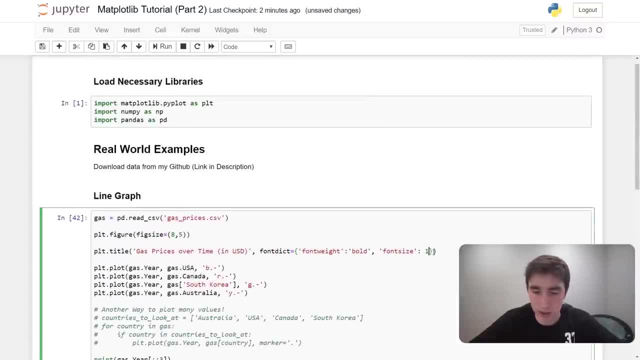 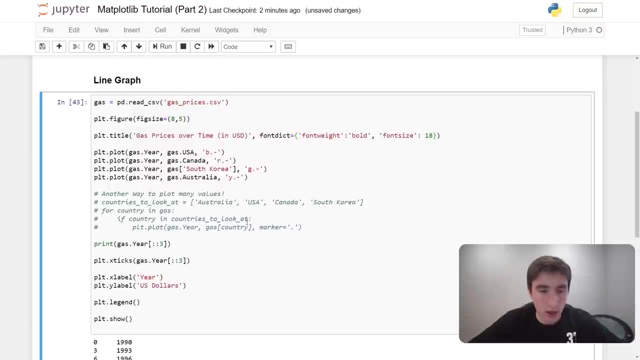 a larger font. maybe 18 is a better value. Um, so you can do that. You can do that for any of your, your labels. Uh, another thing we might want to do is in the when I showed this graph originally. 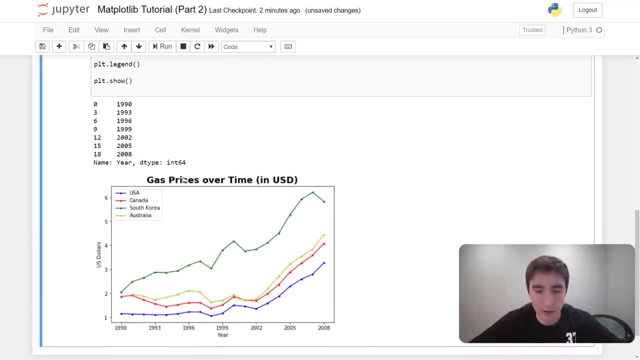 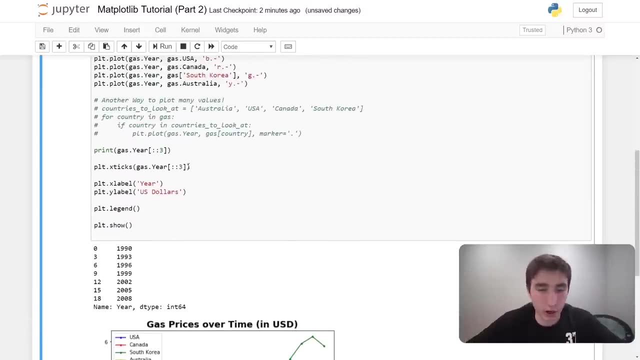 I also added the year 2011.. We don't have values for 2011,, but maybe you wanted to allow for the ability of that showing up and maybe project where they're going. You could do plus you take your ticks and plus 2011.. 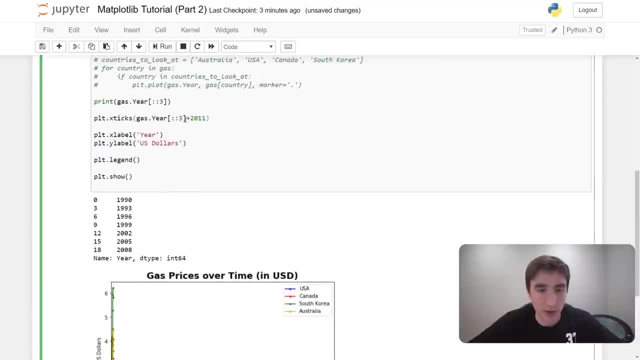 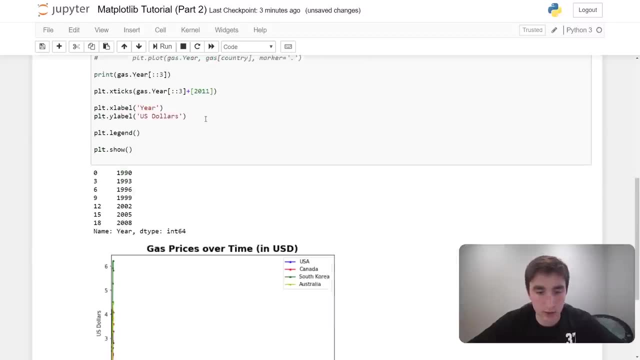 Ah, that did not work. Um, so this is a lit or this is a data frame, So we can't just directly add 2011.. So we need to make it a list. still didn't work And the problem is the data frame. 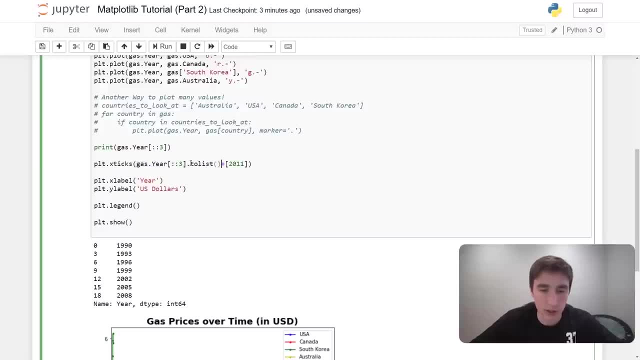 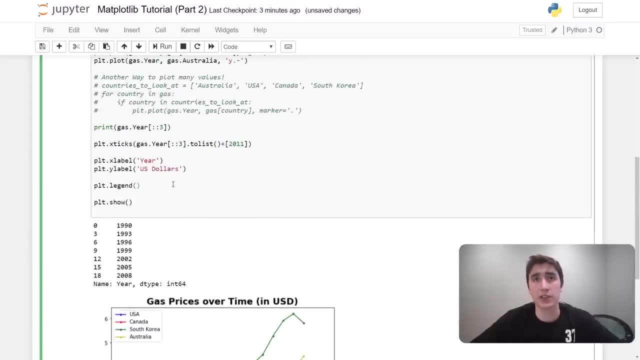 is weird when you add just a direct list, So you can do dot to list and now do this, And now you see 2011 is there? Um? and then if you wanted to actually save this graph, remember we can do plot dot, save fig and give it a name. So gas price figure, Sure, And remember when we're saving. 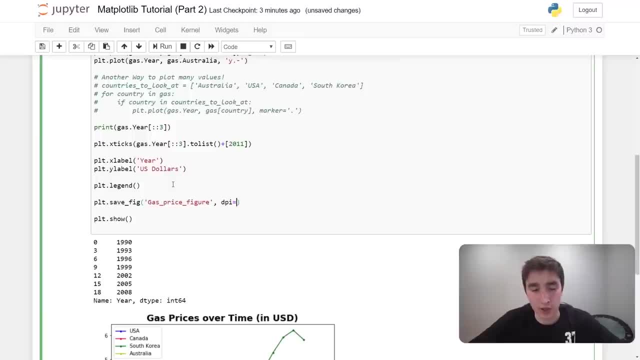 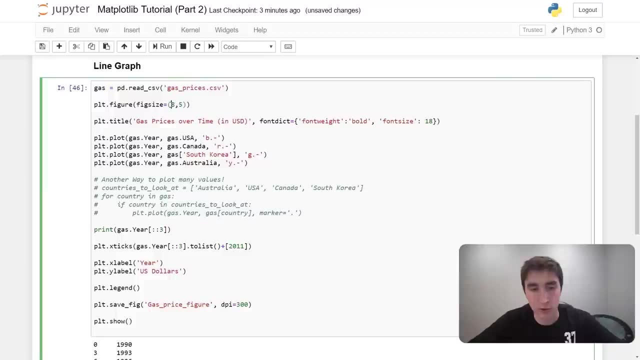 uh, if you change the DPI you'll get a higher resolution image. So 300 is a good value. This is going to make a pretty big image. It's going to be a pretty big image. So we're going to do make a 300 times eight, which is 2,400 by 1500 image. But so really you can play around with. 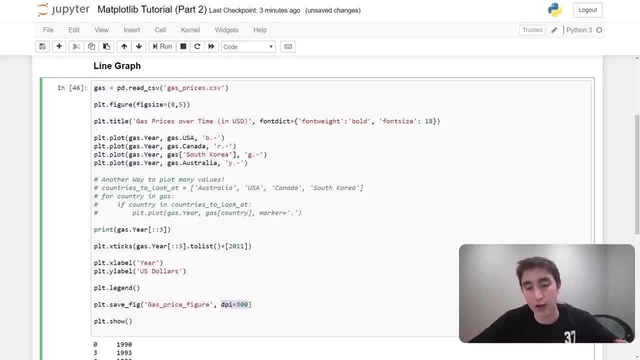 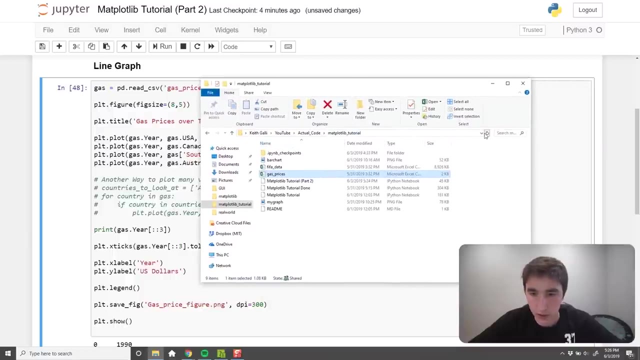 this video, but the higher the resolution, or higher DPI, the higher resolution image you're going to get. So, Oh, I don't want to say this as a PNG. So if I went into that folder that I had, as you can see, uh, where did it go? Refresh- Oh, I don't know where I'm saving this. 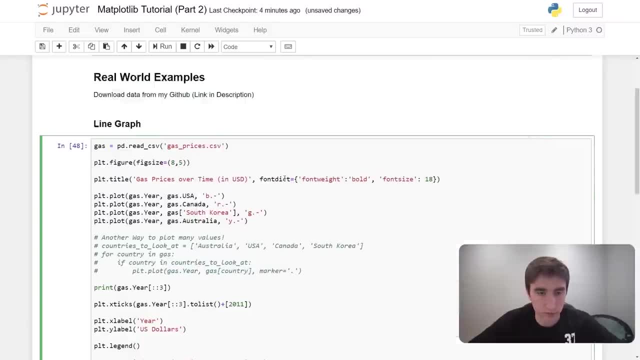 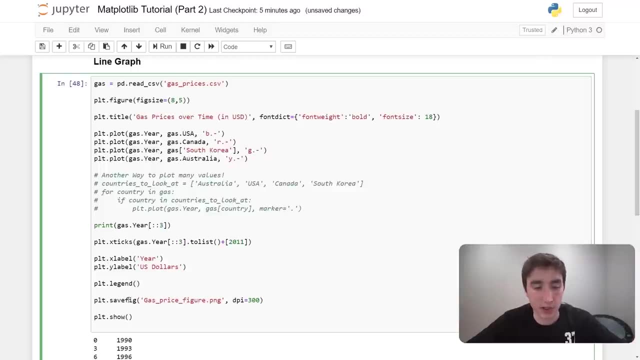 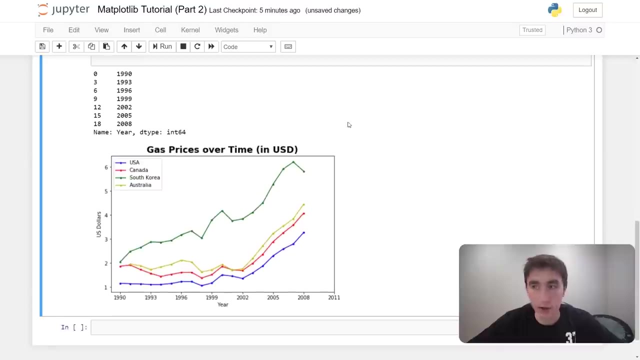 Gas price figure. Where are you All right? Sorry, I typed this in wrong. Save fig. Uh, and you always just you can refresh and look at the documentation I might've gotten. yeah, I got an error here. I should have noticed that before. but yeah, save fig. one word. Do that Now if I go to 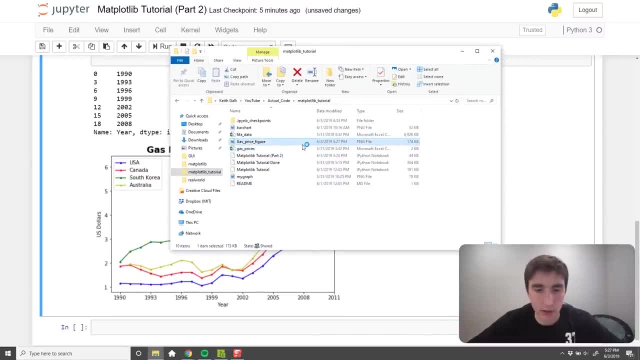 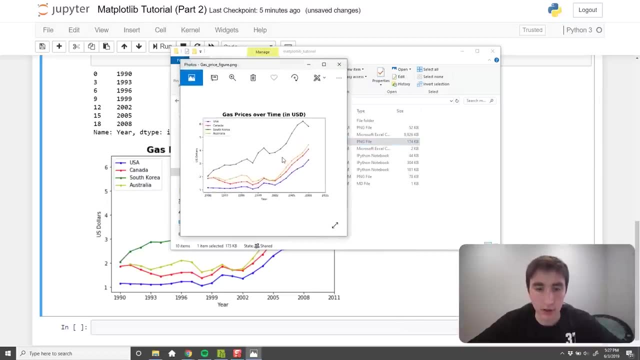 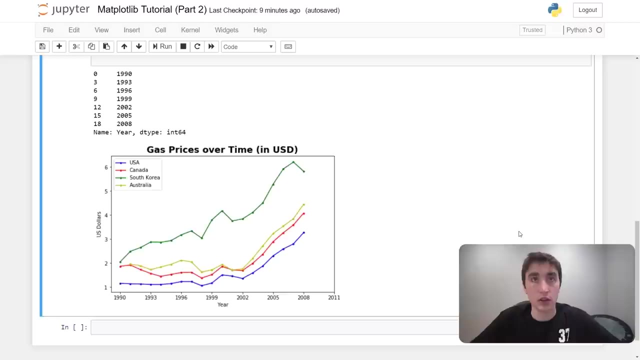 the folder that I have these files in, we've got gas price figure And if I bring that in, you see the figure I saved nicely as a PNG. All right, let's move on to the FIFA data. Now that we're done with the 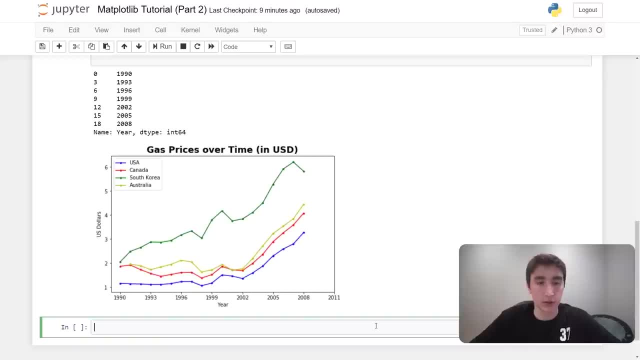 gas price stuff. let's move on to using our FIFA data. So we're going to first going to have to load it in. So, and if you didn't save the FIFA data, um, maybe if you skipped around this video, um, it's on my GitHub page and the link to that is in the description and you want to save it in. 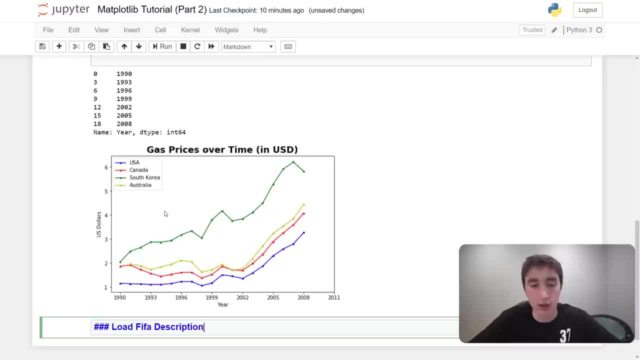 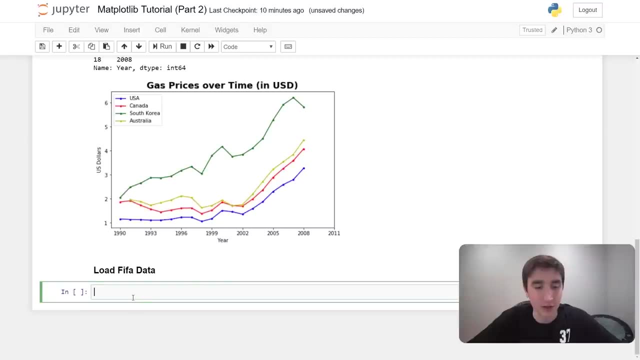 the same directory of the file that you're using to uh produce these graphs. uh, Lou, I'm mixing my words. load FIFA data. Um, okay, So to do that, we'll just call FIFA equals PD dot read CSV. And I believe we called this FIFA data dot CSV. 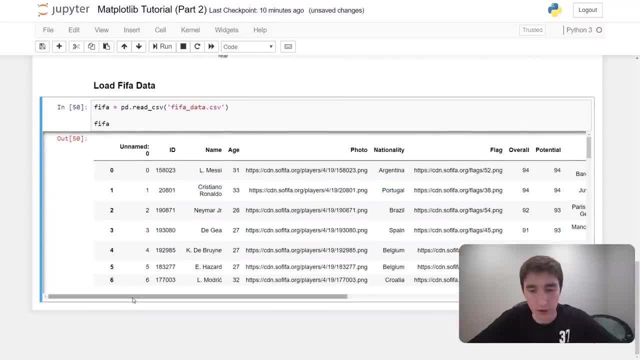 And let's just check to make sure it's loaded in properly. Cool, And this is actually shoot. I shouldn't have loaded at all. Uh, okay, It's still a preview, but you could do something If you only wanted to see, like the first five rows. 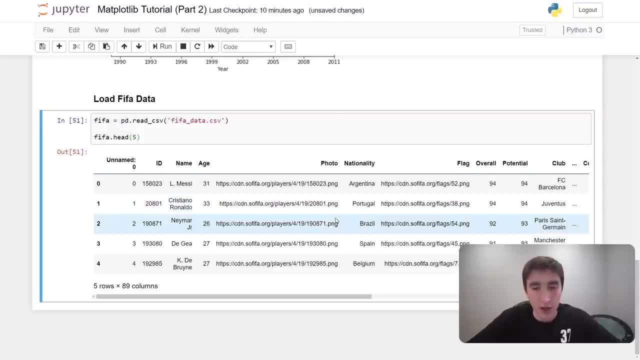 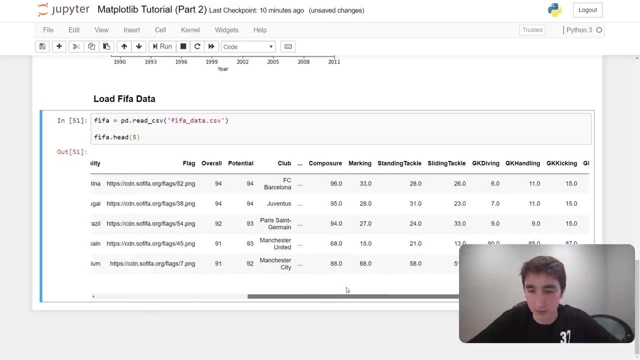 you can do FIFA dot head five, All right. So so you can get a feel for what's in this data. Um, you got like the name of the player and you should probably recognize some of these guys' names: Lionel Messi, Ronaldo, Neymar, all very good players. I think it's right now sorted. 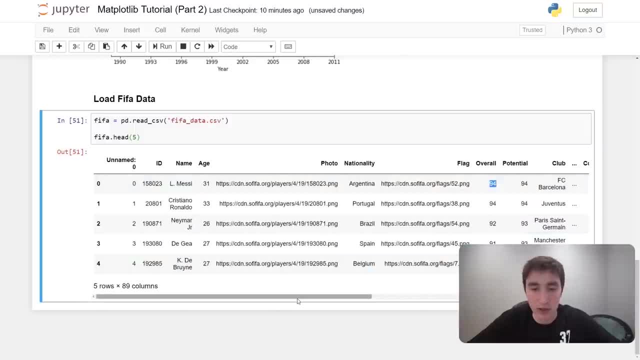 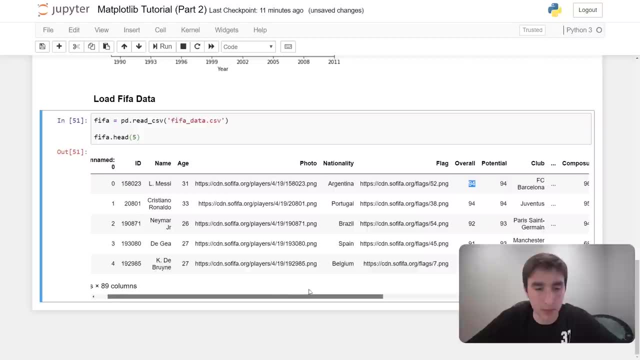 probably by their overall, but yeah, it's all the stats from the game FIFA for these guys, And I think it just provides a good set of data, uh, that you can work from. And also, I took this data from a Kaggle challenge. 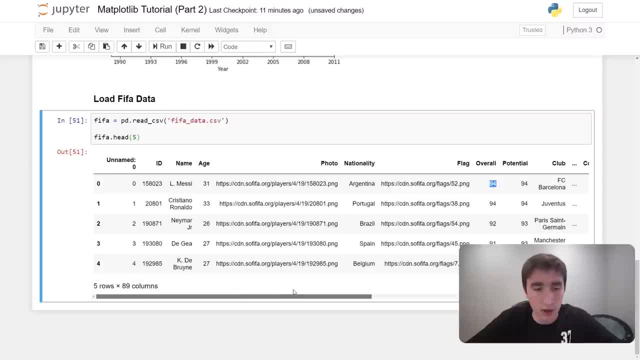 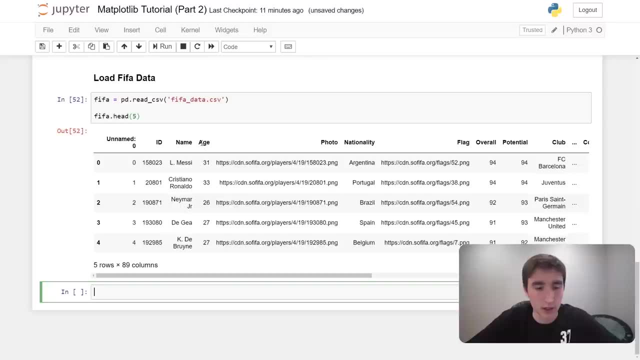 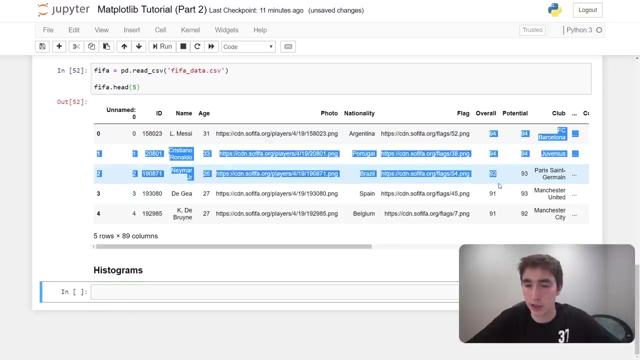 I'm going to link to the original source of the data as well, Um down in the description, Okay. So what can we do with this? So, to start off, let's do some histogram stuff, Okay. So what I think is cool? First thing to do is plot the overall skill level here that you see. 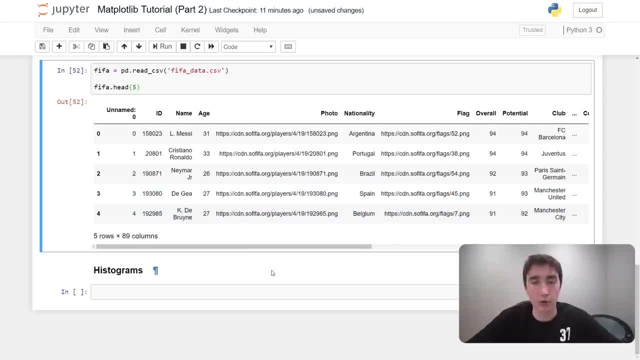 on the right. just figure out in the game, like how many people have above a 90,, how many people have between an 80 and 90,, um, et cetera. So what we can do to do that is we have our data already. 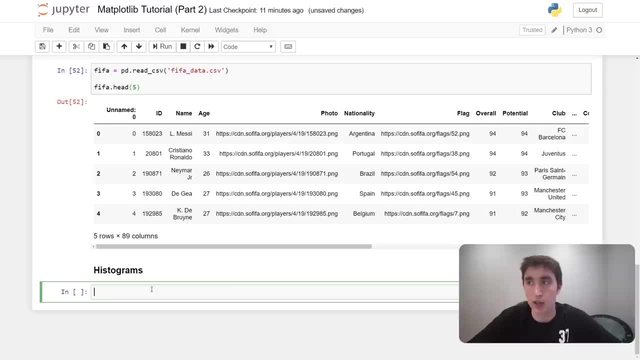 loaded. I don't have to reload it in, but I can go ahead and do um. let's see plot And the way that I remember these commands is like I showed in the last video. you can kind of use the pie plot. 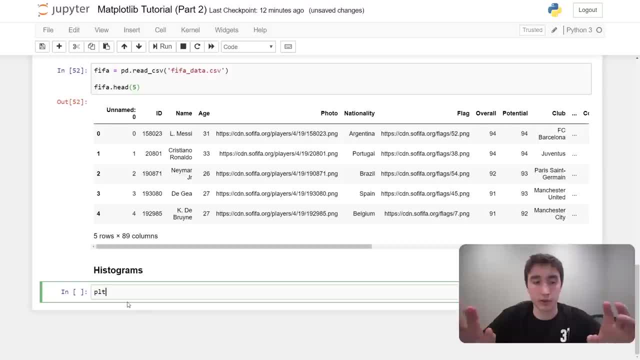 Um, documentation as you're kind of your starting point, And then if you're looking to try to do a histogram, look up histogram within that documentation. the link to the documentation is in the description and you'll find the command hist. So what I can pass into hist is within the 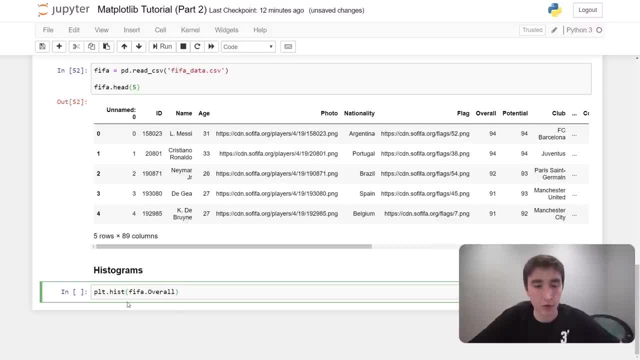 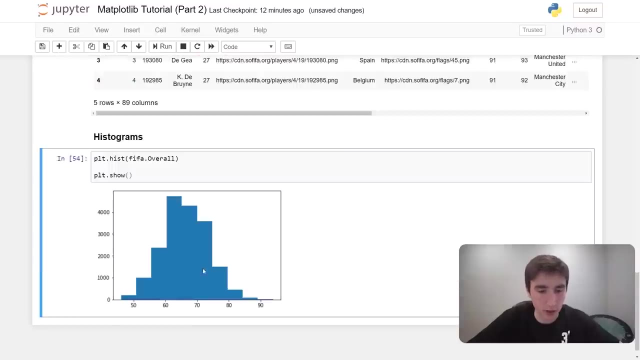 FIFA data set. I'm going to pass in the overall skill level as my input And let's see what happens when I do that, And then I'll do a plot dot show So I don't get all of this random stuff. Okay, That looks pretty good. 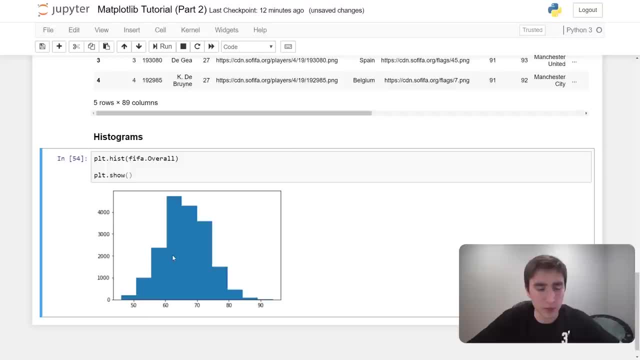 It's already starting to get there. Um, what would probably be more helpful is if this kind of these tick marks were centered for each bin that we have, And I'll do that in a sec. All right, We're going to set the. 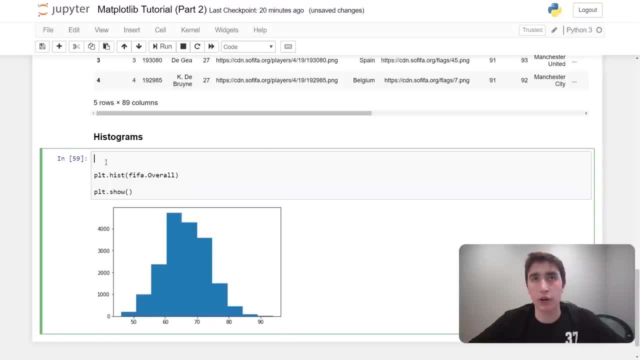 bins every 10 overall skill level points. So, like the highest you would be in the FIFA game is a hundred, The lowest you could be as a zero. So we'll do our bins at intervals of 10 up to from zero to a hundred. 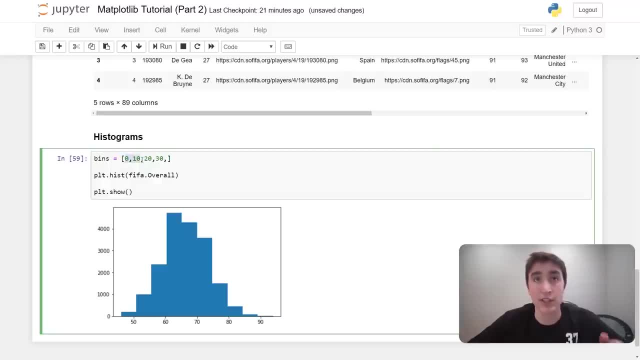 So the first bin that we have will be all players that have a skill level between zero and 10.. And it's counting, uh, that number: 50,, 60,, 70,, 80,, 90, and then finally 100. Cool. 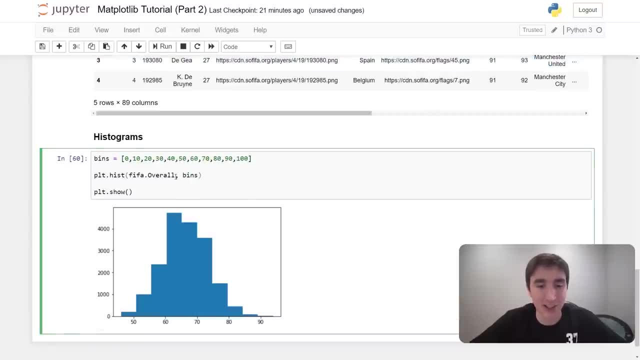 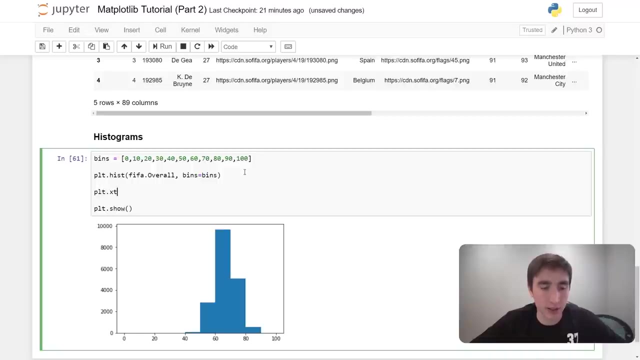 So, oh, I didn't do anything yet. Now we can set the bins parameter of the, the histogram, to our bins. Now we got a nice- uh, a little bit nicer- of a graph. Now the next thing I'm going to do is set our X ticks to be the bins as well. 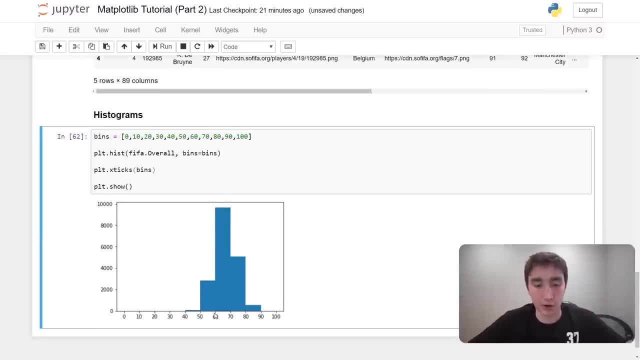 So now it's nicely labeled. Each interval corresponds exactly with what we have here, Um, but it looks like we have some unnecessary data, So it looks like There's very little players over here, So maybe I'll limit this, start at 40 and go up to a hundred. 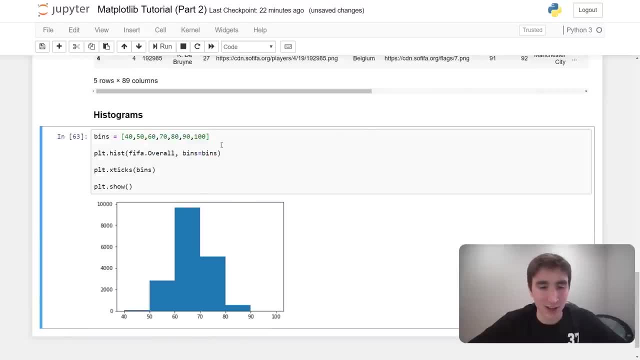 And what's kind of crazy is, you know, the players that are over a 90 are really a- uh, a rarity, Cause you can't even see that bar from the 90 to a hundred range there. So let's do a little bit, uh. 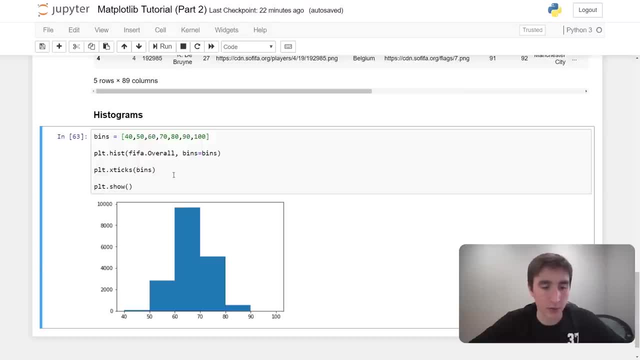 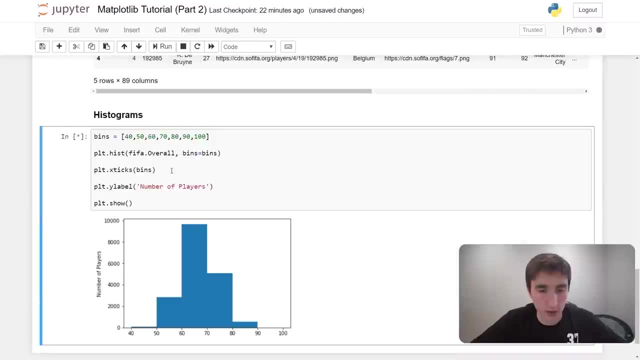 we got a title, same way as before got a Y label. So I'll do a Y label real quick: number of players And the X label would be the skill level. And then we got a title that would be like a distribution of player skills in in FIFA. 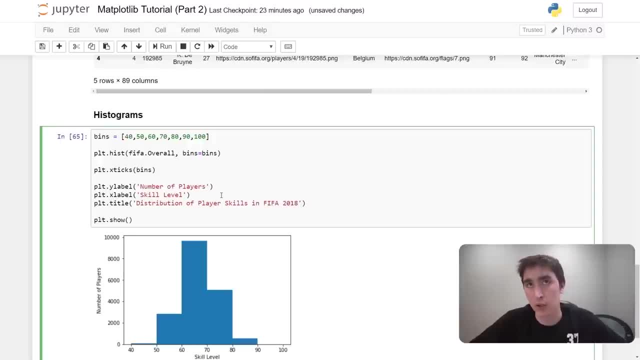 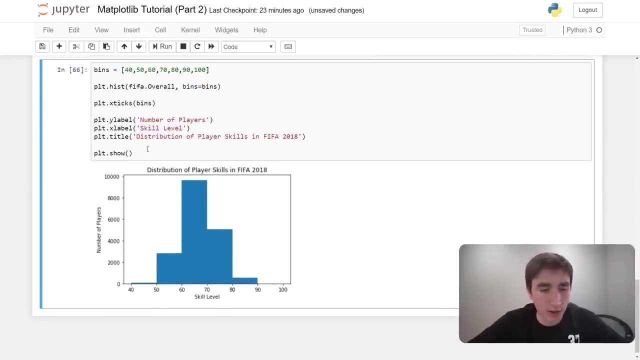 I think it's FIFA 2018 might be 2019, not positive. so that's a cool little visualization and you can get more into details, like to actually see that there are some values there you could do. you change up your y-text to be, let's say, 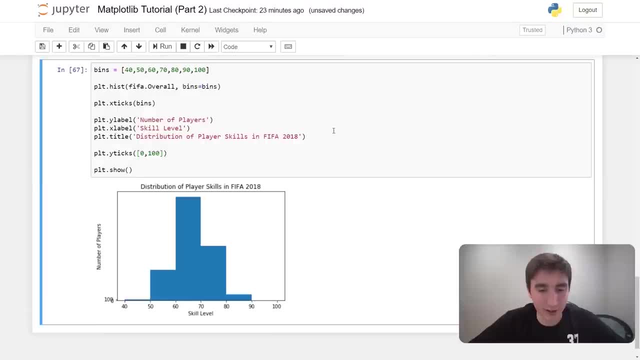 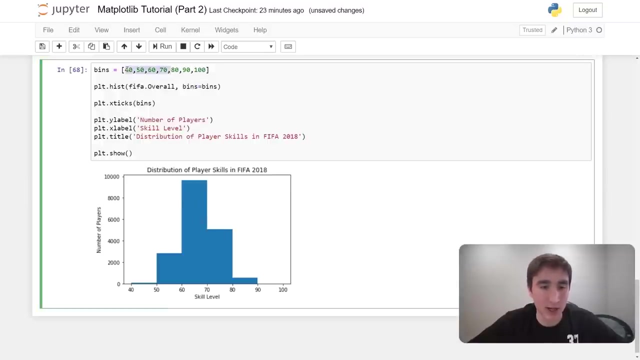 zero to 100. okay, that didn't work. yeah, I guess it's kind of tough with all of these players, but if we did move it from like 80 to 100, you see that, yeah, there are actually players that are above a 90 is just very, very few compared to the amount of players in the game. another: 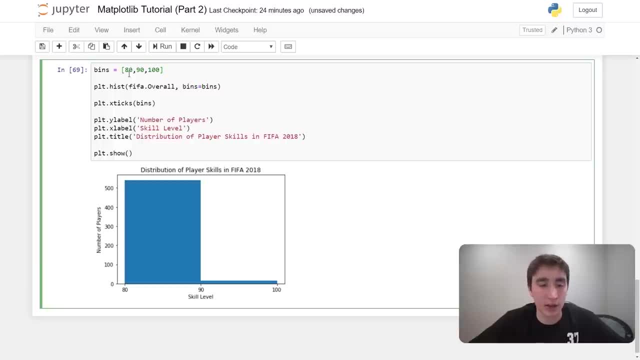 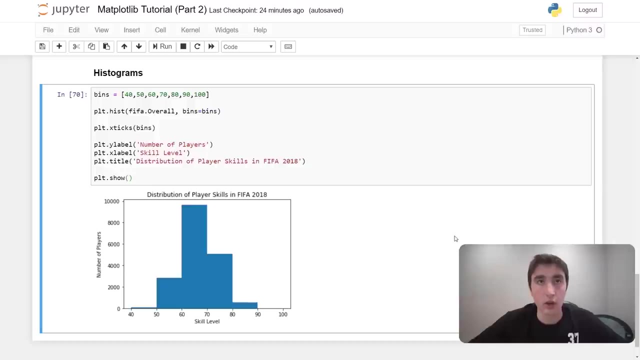 thing you could potentially do is maybe break it up, use the data and only look at the stats of players in certain teams, and then you wouldn't get all the noise. I guess in the lower skill levels that I put all the people in here. one little modification we can make to this is, let's say, we wanted to change the color. 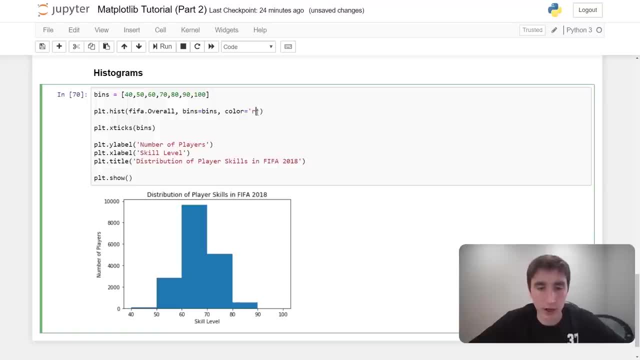 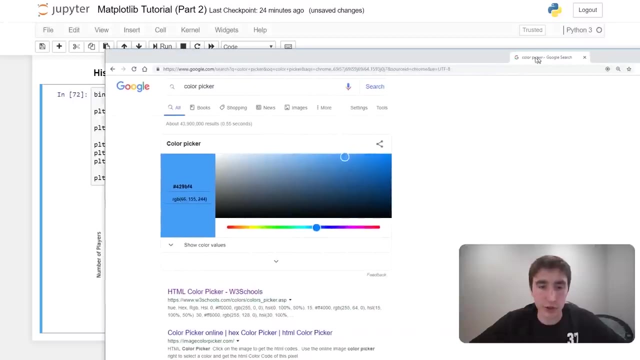 of our bar. I could set this. you know, I could set it to red easily, like that. or I can set it to a hexadecimal value very easily, and what I recommend, whenever you want a certain color, what you can do is just like: do a Google search for a color picker. as you see here, I can just 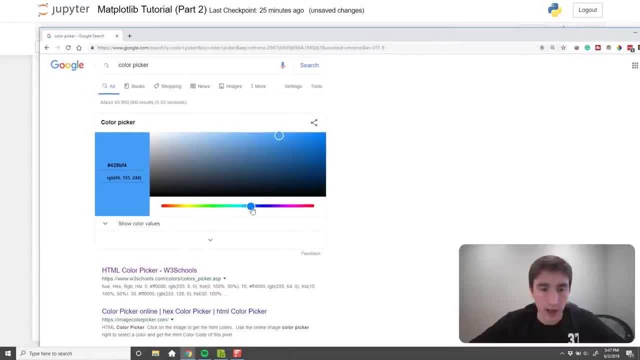 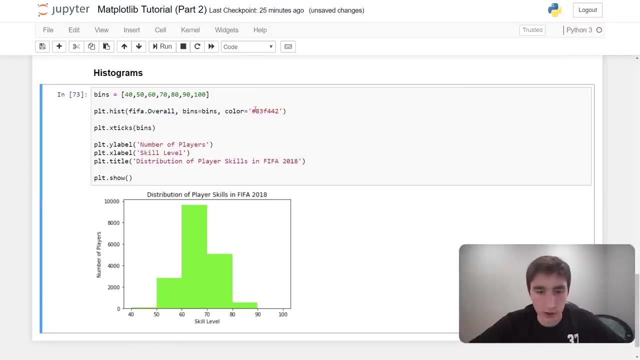 move this bar around and no matter what color I want. so let's say I want this greenish color. I copy that hex code, hide this, paste in and then whatever color I paste in the hex code, Now I get that green color. I kinda like the bluish color, so I'm gonna go with that. 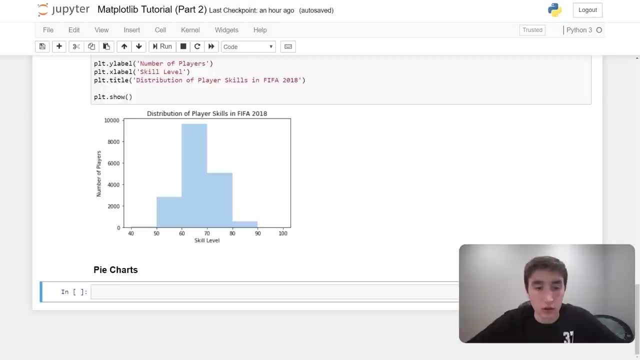 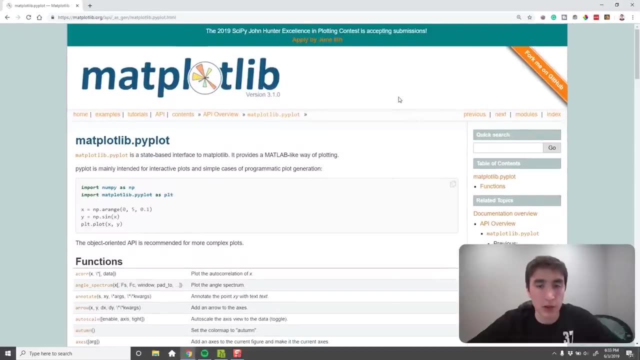 But yeah, you can play around and get any color you want with Matplotlib. All right, let's do pie charts next. And just to start off, I kinda mentioned this, the histograms, but to figure out how to do a pie chart, 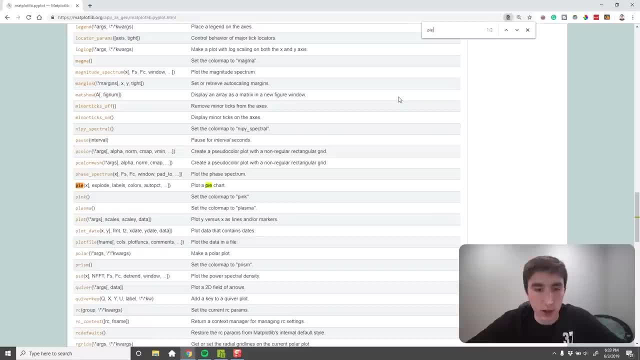 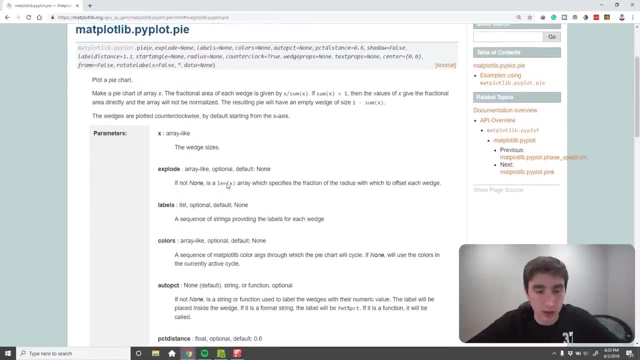 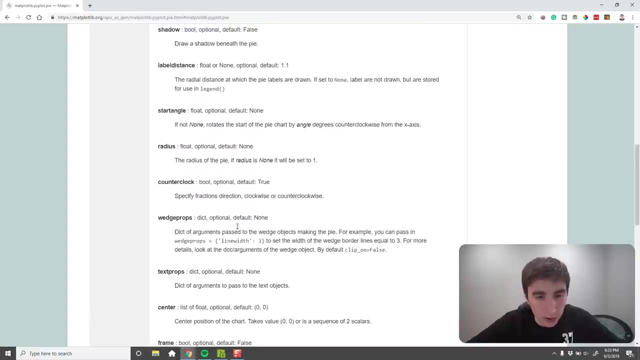 I usually just start at this documentation, look up pie plot- a pie chart is right there- And then with this page I can kinda get all the details of what I can pass in. what are the parameters that I can play around with? 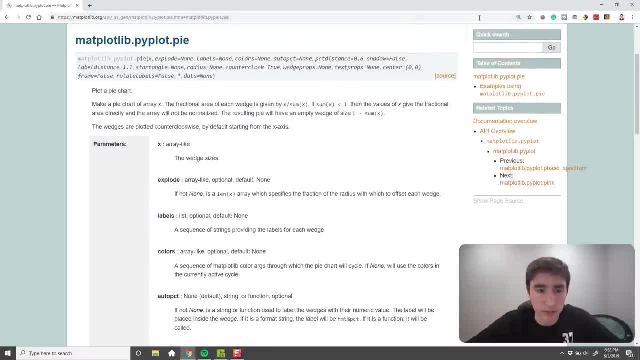 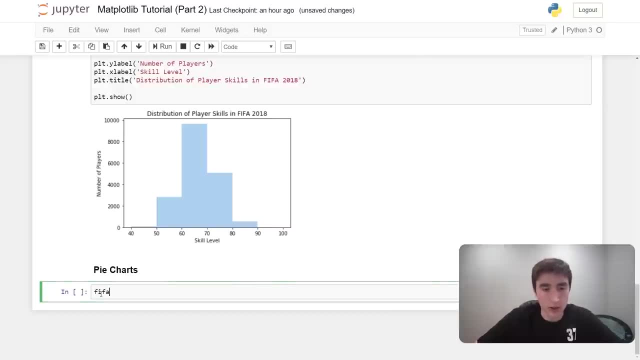 Yeah, a lot of good stuff here. Okay, so the wedge sizes is our X and that's what we're gonna input here. So what does that look like? Okay, so I'm gonna just output some of our data again And what I think we're gonna do. 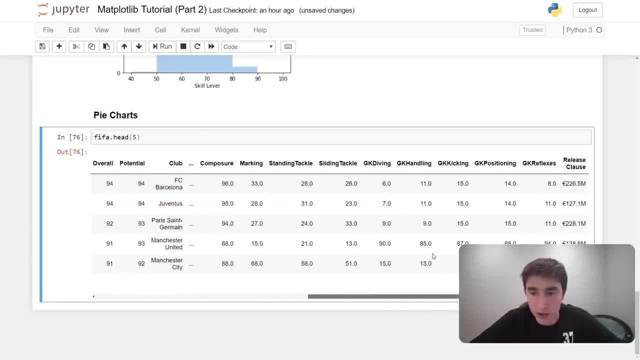 is we're gonna go ahead and do a pie chart, And what I think we're gonna do is we're gonna do a pie chart And what I think we're gonna do, for this first chart is one of the components of this. I guess we can't see it here. 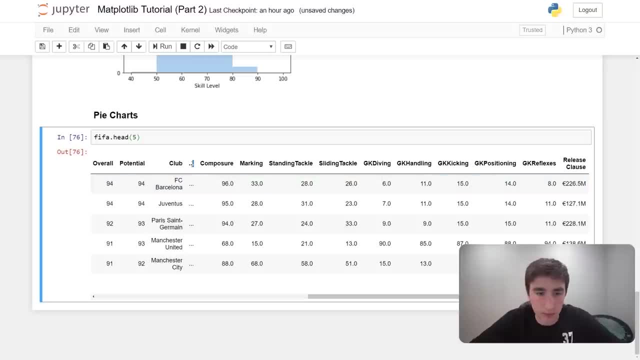 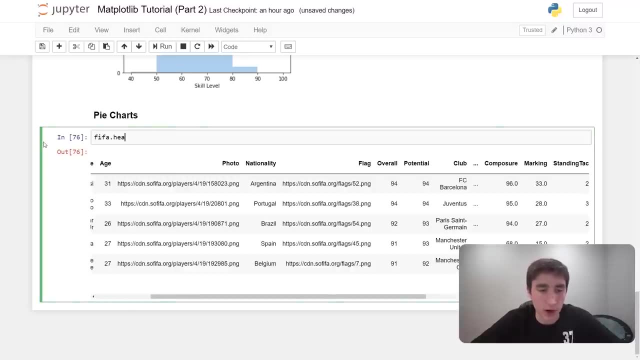 but if you opened up the full- yeah, I can't see all of it- If you opened up the full file within like Excel, you'd see that one of the parameters we can have is preferred foot. So if I look up that, you see that left or right. 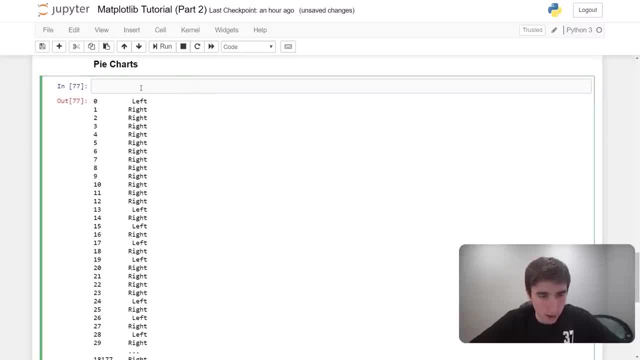 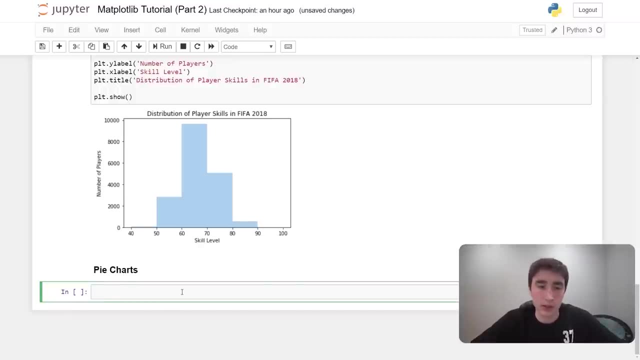 whether you play left or righty in soccer. So what I think would be interesting to do a pie chart on is the percentage of people that play with their left foot versus their right foot. So how would we do something like that? Well, we can count the number of people. 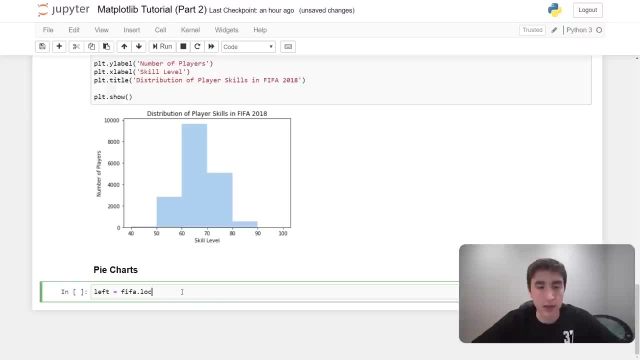 that play with their left foot by doing the following- And this plays into the stuff that I taught in the that we went through in the pandas video. but we can use the dot loc to kind of like look up the data set or kind of filter the data set by a specific condition. 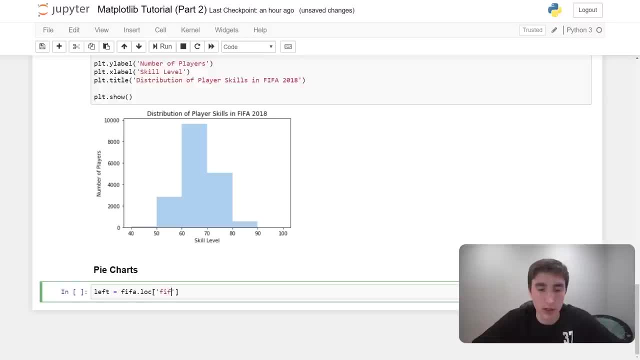 In this case for left. we want the condition to be: apologize, one sec. We want the condition to be: if the preferred foot column is equal to left, then we want only the data that this condition holds. And because we're gonna need to pass this, 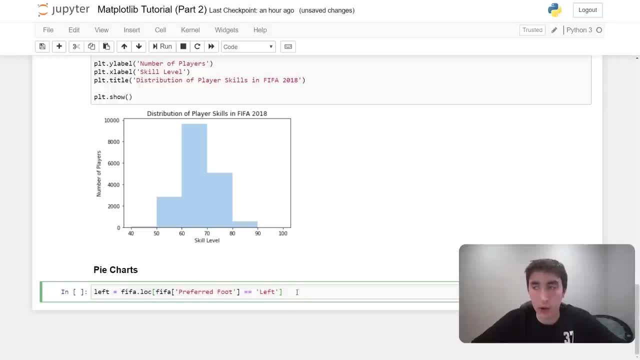 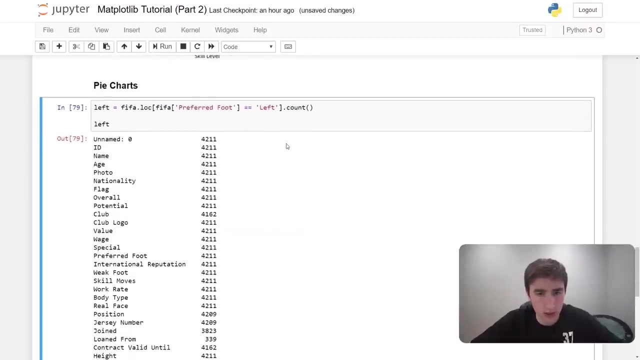 into a pie chart. what we'll wanna do is get the count of that. I believe this count gives us an array I can probably check. So let's see what is the left. Yeah, it's like an array here. So if we do count zero, we'll actually get a number. 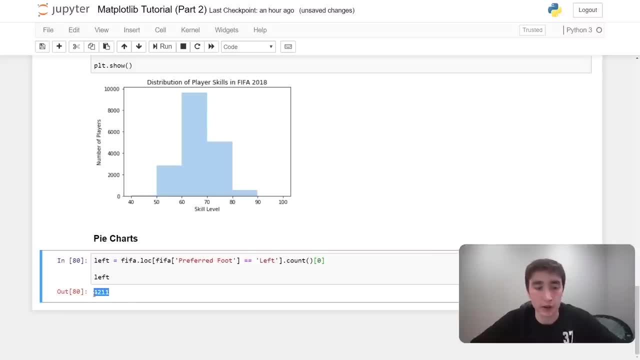 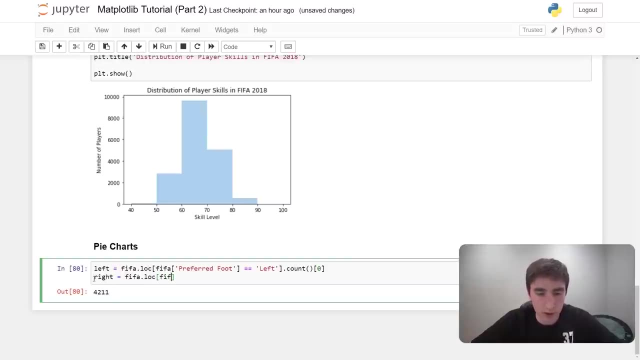 As you can see, 4,211 players prefer their left foot, And so we can do the same thing with right. It's fifaloc, fifa. preferred foot equals equals right. Get the count of that. And then, because this returns a data frame, 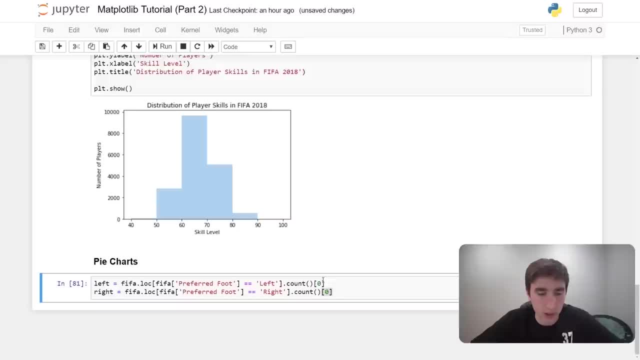 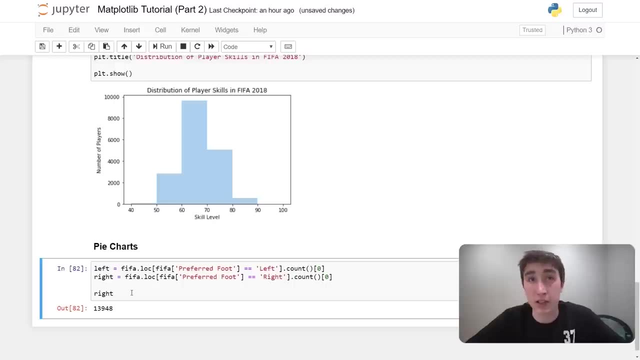 we have to take the. we'll just take the first element, which it will be a number, And let's see how much like right. Okay, so considerably more people preference their right foot than their left. That makes sense, Okay. 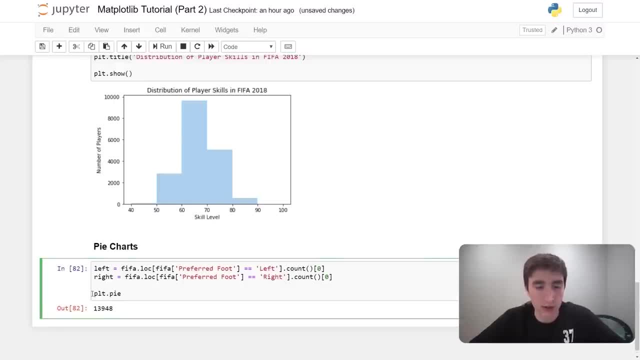 So now, how do we do the pie chart? Well, we can do plotpie. This is from the documentation And I guess I kind of jumped ahead. but you might like think maybe I can just go ahead and do fifa preferred. 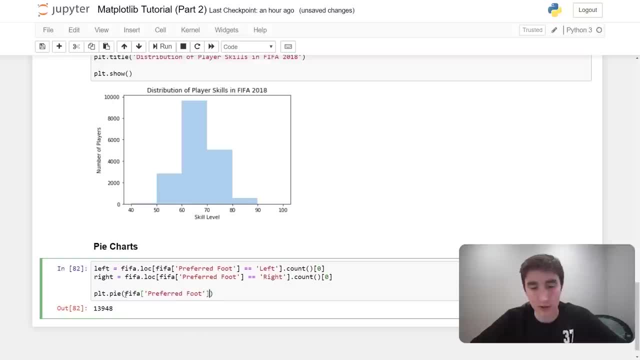 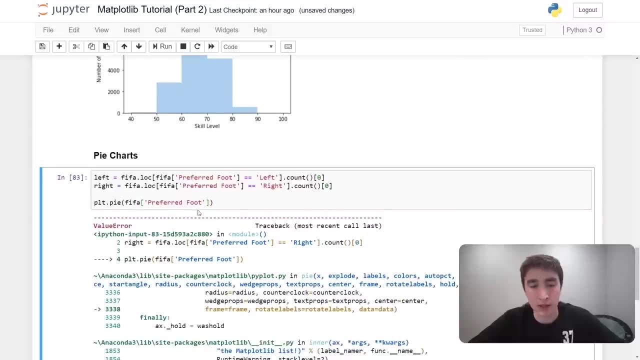 I can't even spell. Of course that won't work. Foot and like figure that it might just plot the pie chart while doing that, But it gets messed up when you don't pass it numbers. So what we need to do is passing a list. 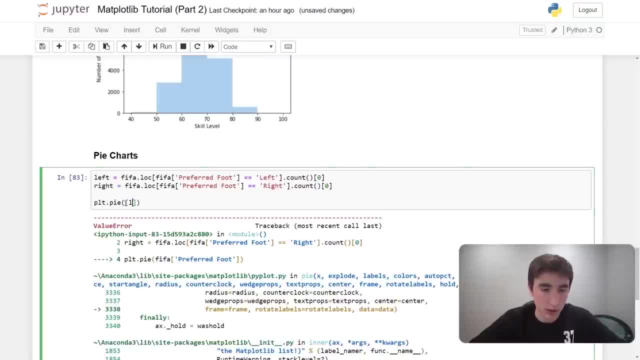 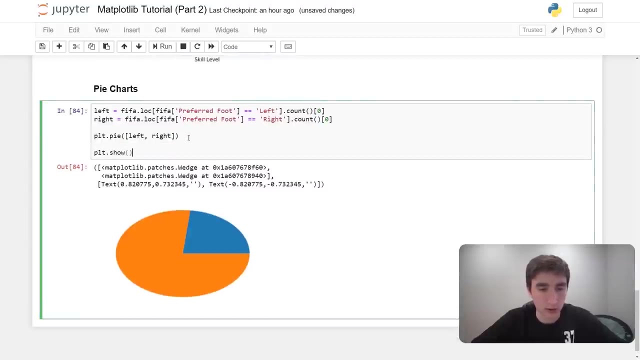 of numbers. So what we can do is left comma, right. So now we have two values and I'll make a part pie chart out of these values. Look at that Cool, And I'll do plotshow. One thing I'm noticing is these colors are really ugly. 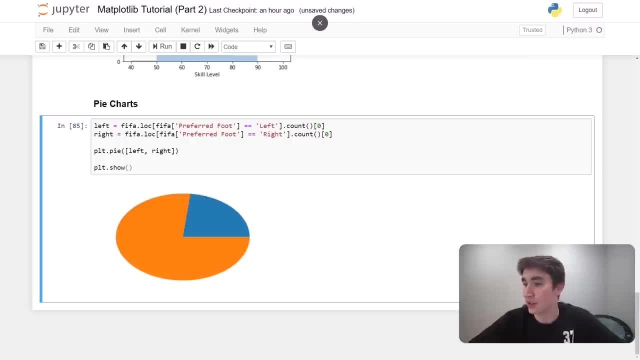 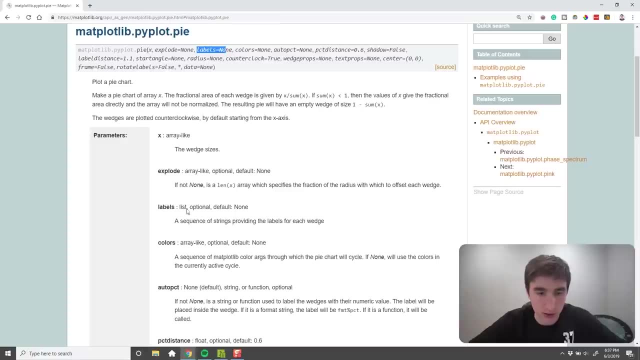 and also nothing is labeled right now. So, going back to the documentation, you can see labels is a list sequence of strings providing the labels for each wedge. We can pass in that We can also change up the colors within a list as well. 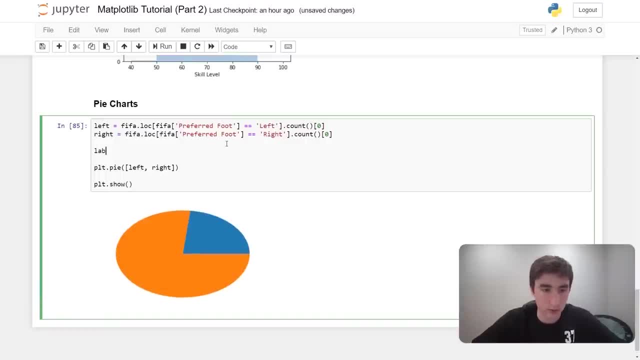 So let's do that. So labels, we'll do equals left and right And we'll pass those into our pie chart. Do labels equals labels, Cool. So now at least we have like relative percentages. I mean, we don't know the exact percentages. 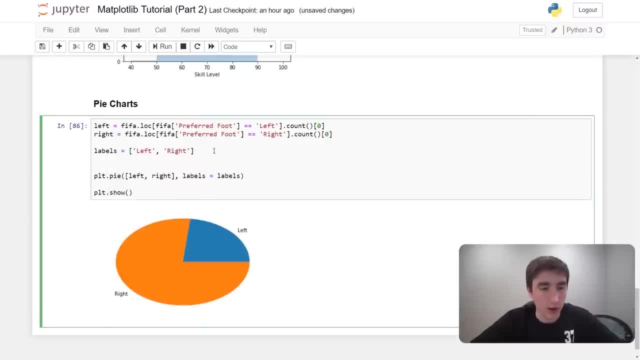 but you have an idea just based off the graph. If we added in colors, we could change this ugly orange from being there, So you could pass in two colors. Let's say, like we're gonna just use some hexadecimal values. I'm just typing in these in randomly. 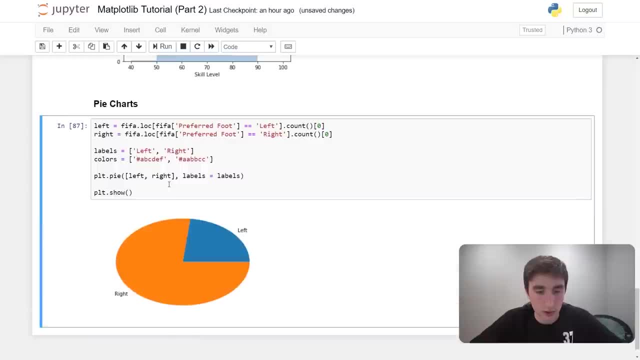 And now I have to pass in colors here. Cool, Now that looks all right. Maybe you'd want a little bit more contrast, but it doesn't really matter too too much. You can be the judge of that. If I do auto percentage. 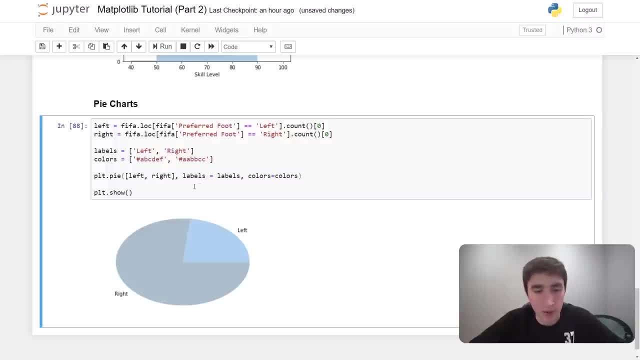 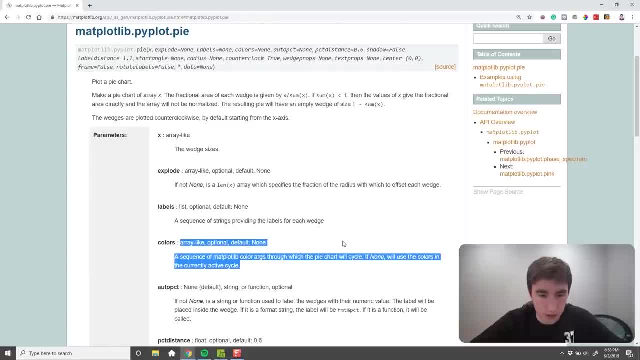 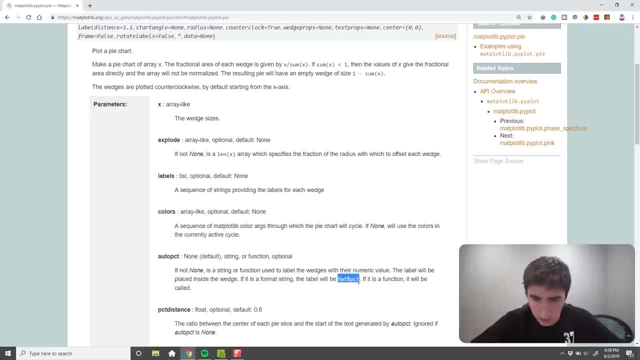 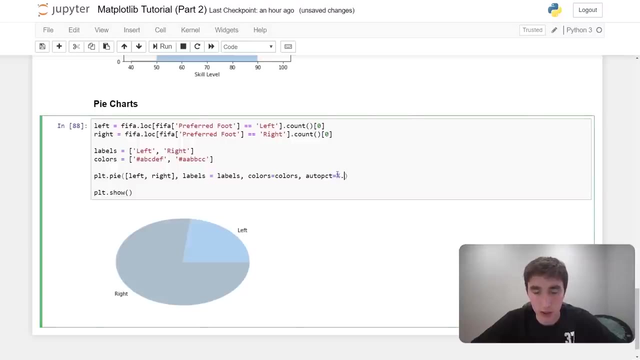 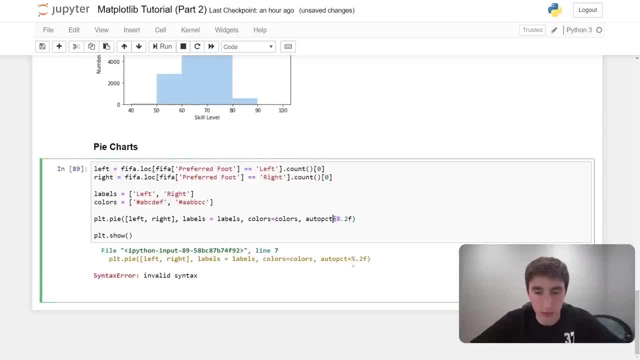 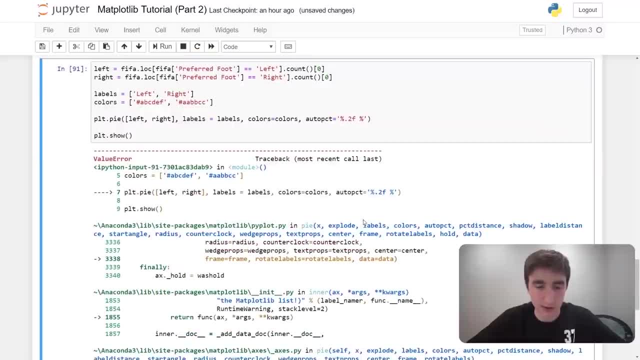 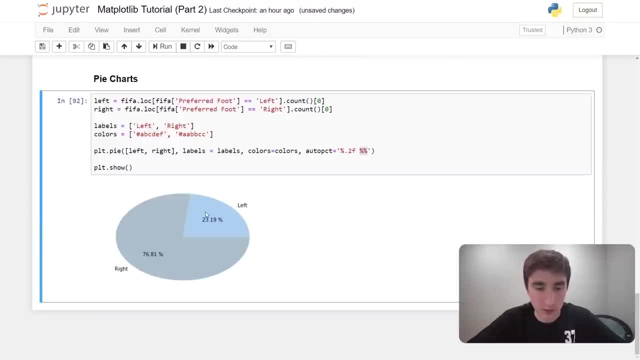 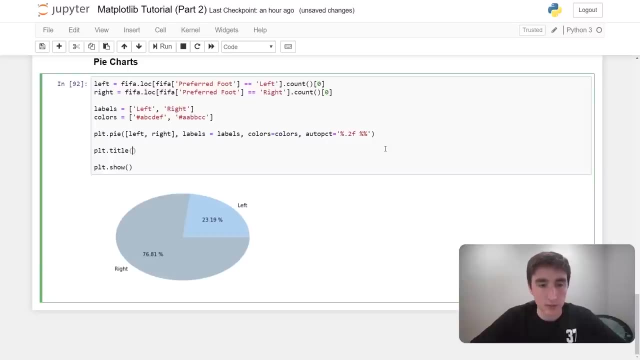 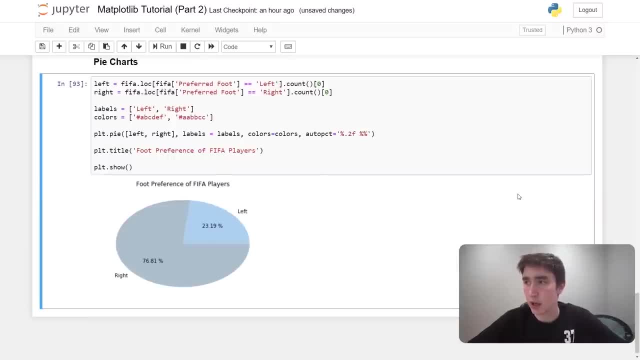 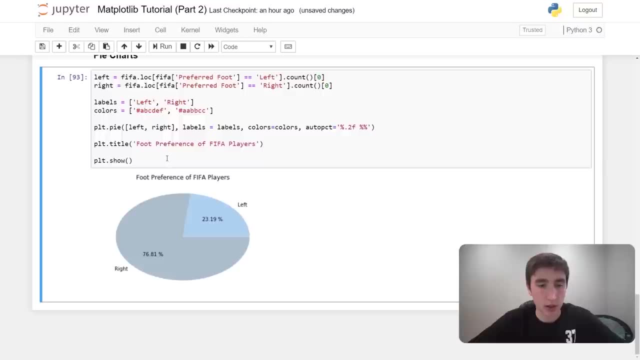 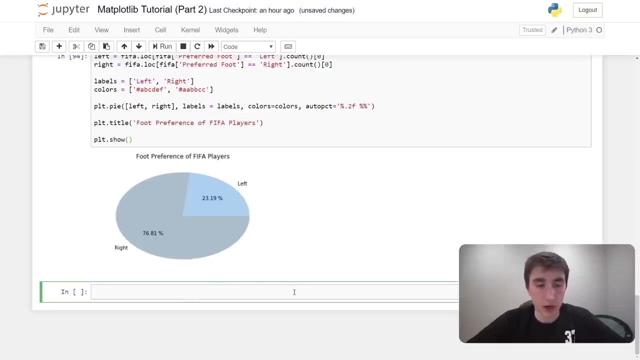 chart. I'm trying to think if there's other things I should add to this we'll. we'll get into a little bit more complicated stuff in the next pie chart that we'll build. so this is a pretty simple pie chart. let's make another pie chart. all right, pie chart number two. so in this one what we're gonna do is look: 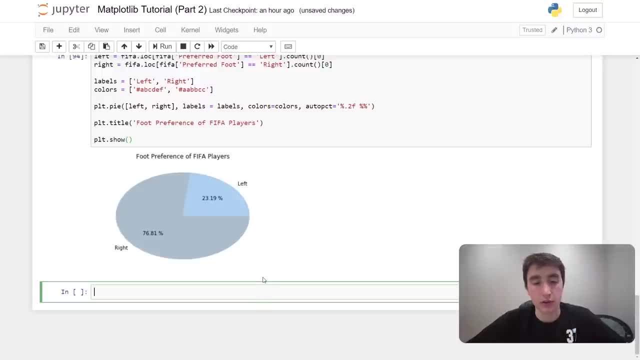 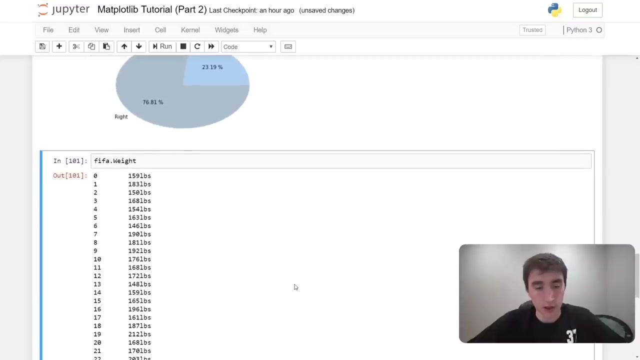 at the breakdown of the weights of the FIFA players and we'll plot it as a pie chart. so I mean, okay, let's look at what the weights look like. so I'm gonna print out weight here, okay. so we have a list of all these weights we can see. is that there? 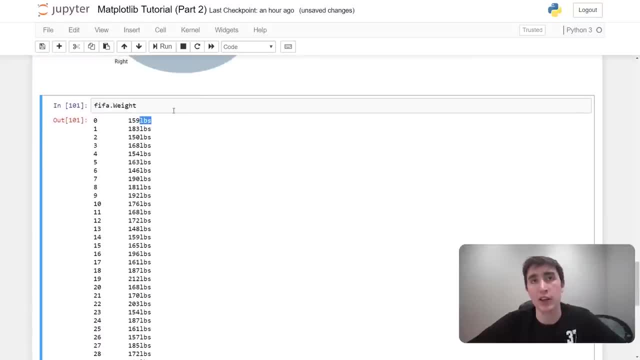 and note that they're in pounds. they're not in kilograms, as many of you guys might expect- and pounds. but you could initial step you could do to this pie chart would be to convert all these values to kilograms. that'd be a fun little exercise. but okay, we have all these pounds. and one thing I immediately 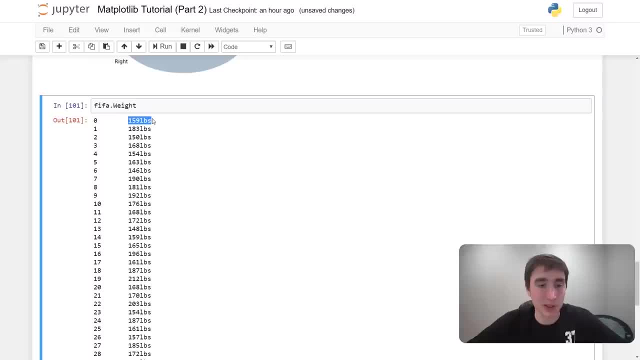 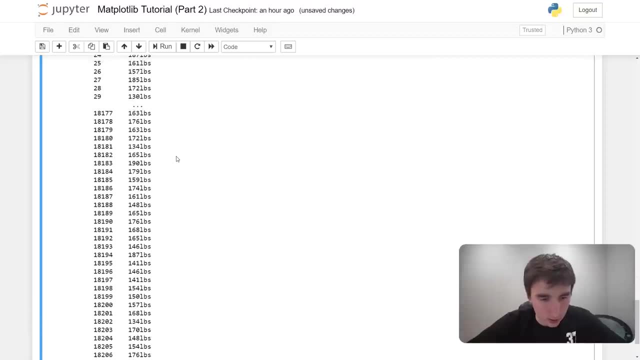 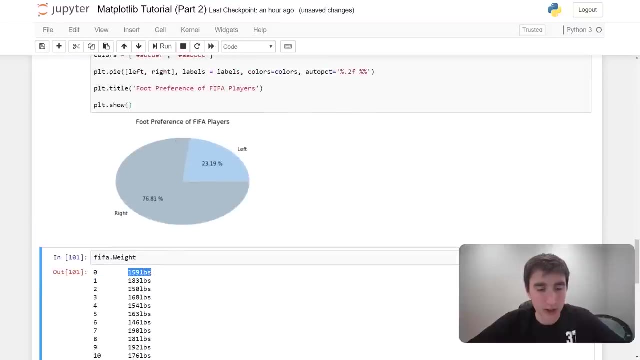 notice is: if we're trying to count ranges of these pounds, it's gonna be off with this pounds string attached. is there anything else I notice here? no, it's mostly just that, but okay. so basically what I want to do is reset the weight category to not include these pounds and just be the number. so this is. 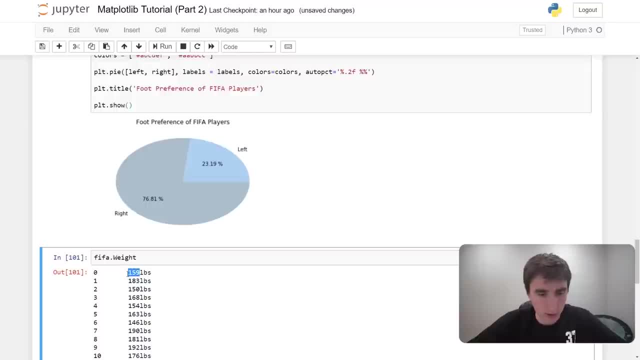 going to be a string right now and we just want this converted to an integer, so let's try to do that. okay, we're going to reset the weight column and what we're going to want to do is strip off, so X here we're going to do X for X in FIFA dot weight, so X in this case is going to be a string, so we can do. 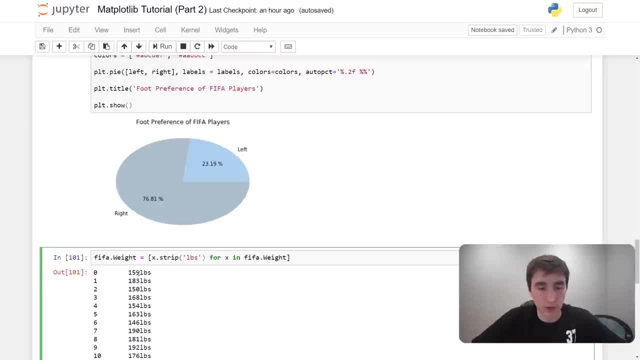 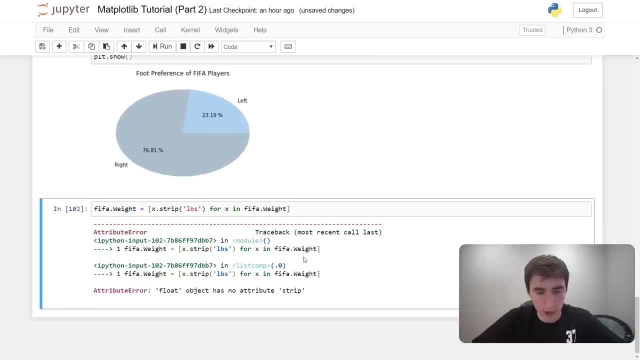 strip LBS. so that will give us just this part of the string for action FIFA. wait, let's see if that works. uh, float object has no actually strip. interesting, I mix. I was expecting that all these would be strings start to start with, but because they're not, what we can add is an if statement within our 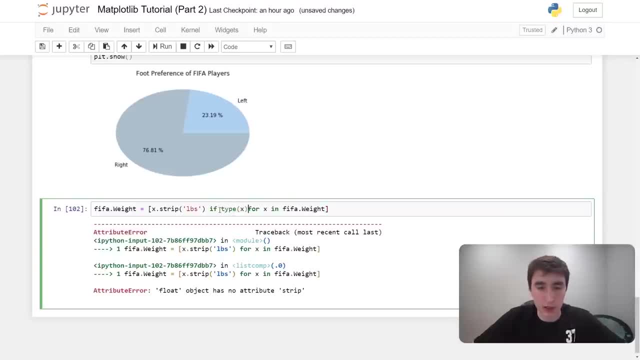 list comprehension. I'm going to just say if type X equals, equals string- I'm guessing maybe there's a couple empty values or something, so we're just kind of ignore those- and then else X. so if type X equals, equals string, we're going to do this, else just leave it as is. that's what we're saying here. let's see. 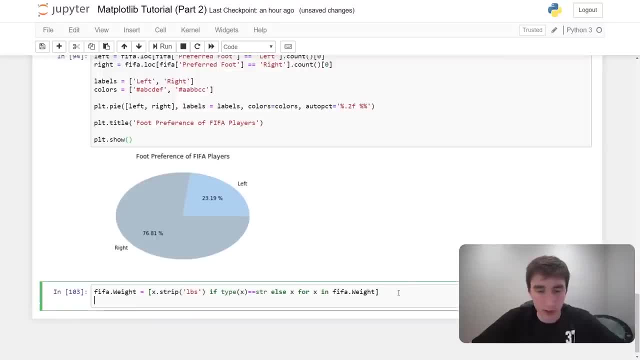 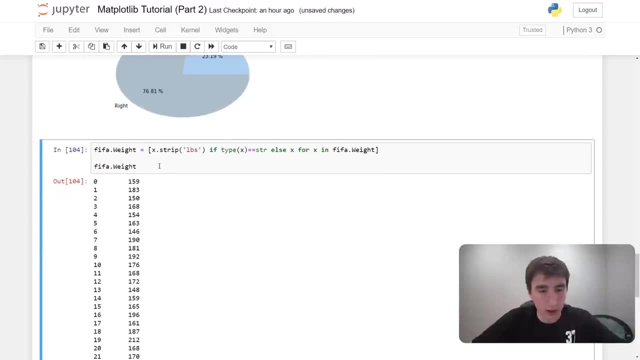 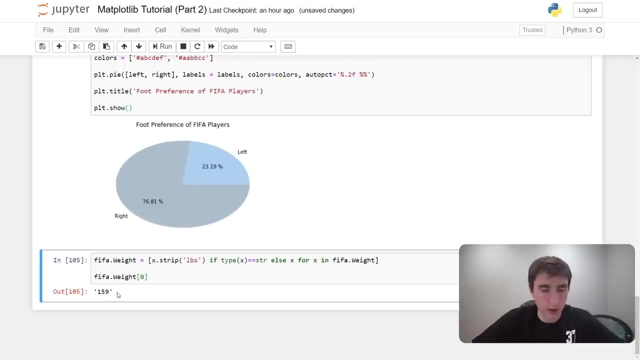 if this works, now we print out FIFA dot. wait, cool, cool. and I'm going to take the first value real quick and notice it's still a string. so what we're actually going to want to do to this line is surround it with the in block, which will convert it to an end. now, if I look at 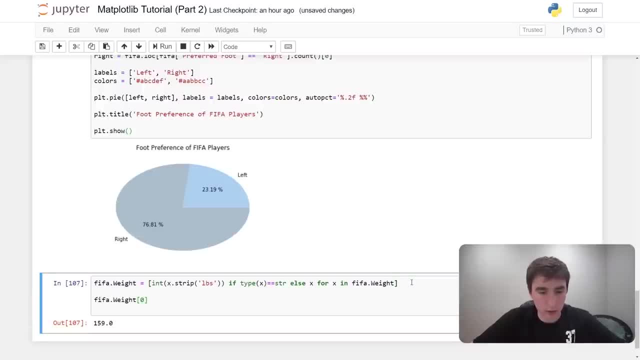 this FIFA dot wait zero. we get it as a integer value- I don't know why it's giving a decimal here, but should be an actual value. and then if I look at the first value, I'm going to take the first value and you notice, because the point zero, we know that it probably is being read as a 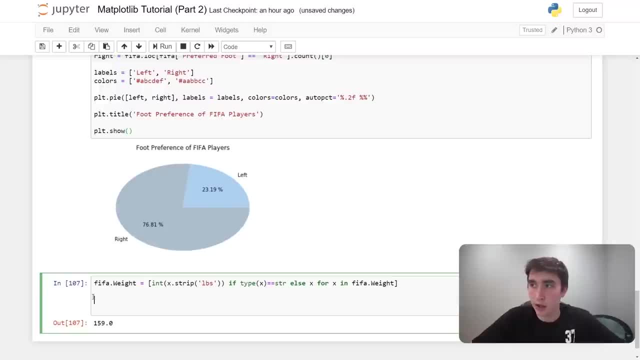 value. okay. so now we have these values set right. so let's start counting things. so we're going to start with light players and we'll say: light players have a weight under. this is kind of arbitrary, but we're going to say that they have a weight under 125 pounds and then we're going to count that, just like we did in. 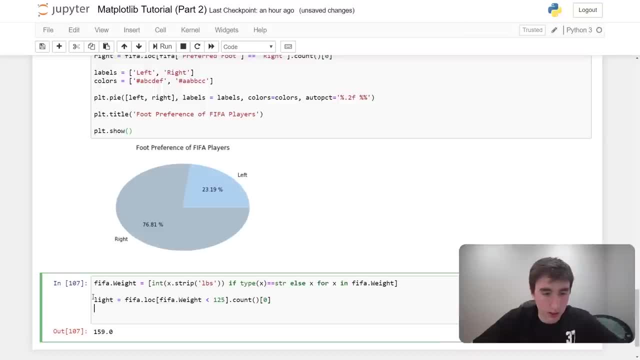 the last example, then the next condition we'll do is, I guess, medium light players that will be above 125, greater than or equal to 125. then we need an and condition, the and condition and the way we're gonna format this with our pandas. notation is like that and this is probably review a bit. 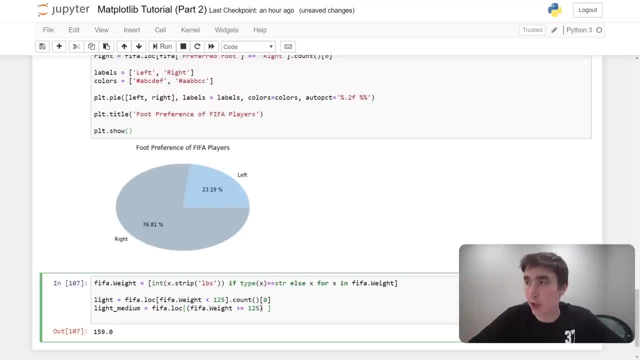 if you did watch, watch through the pandas video that I did. and FIFA dot. wait, zero weight is less than 150. let's say so now. we're getting only the rows that have both of these conditions. true, we're gonna count that zero. keep doing this. I'll probably speed this up when I edit the video. I'm gonna just get three more. 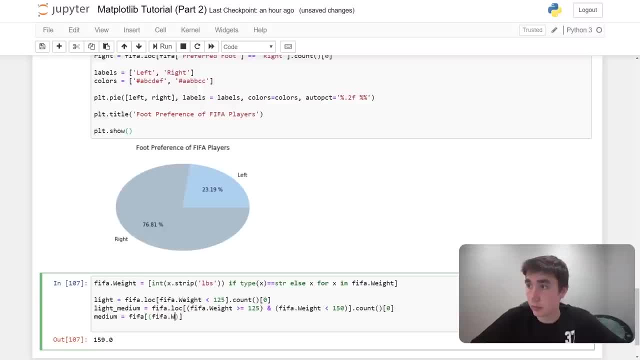 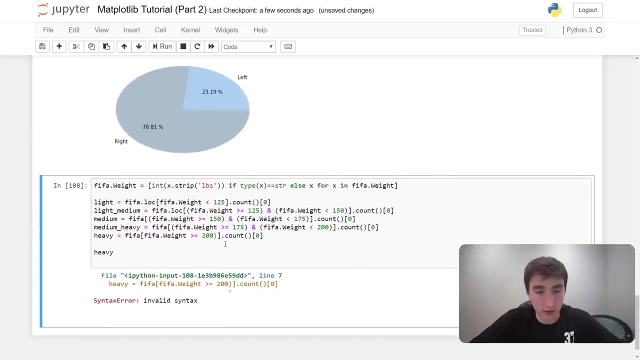 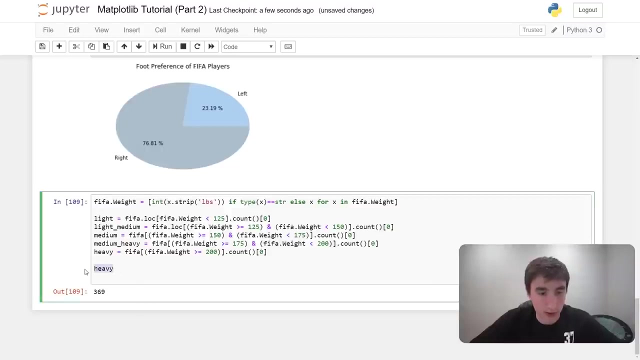 categories. all right, cool. so we have five different weight categories and I can like print these out. I don't know invalid syntax. what did I do? oh, didn't end up. 369. heavy people, medium heavy. let's see if this is a valid number: 4,000. so yeah, it makes. 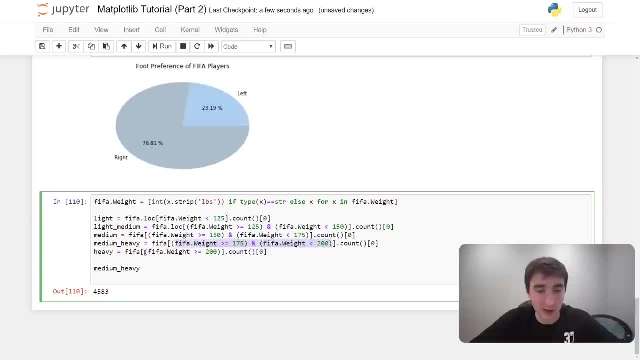 sense that that's a valid number. so let's see if this is a valid number. so there's more between 170 and 200. then there are people over 200 in the league. it's kind of tough to be a soccer player over 200 pounds, okay. so let's now plot. 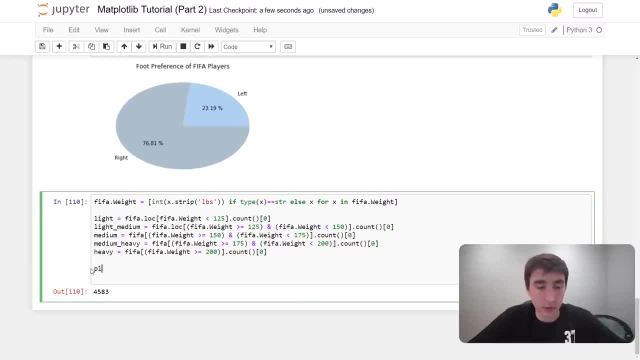 this. so what we want to plot will be our weights, and I'll make this an array: light, light, medium, medium, medium, heavy and heavy right, and our labels can't type today, all right, so plot dot pie. waits, let's see what this looks like. cool, it looks pretty good. 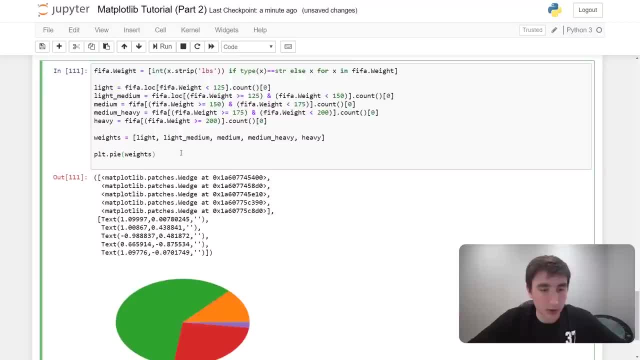 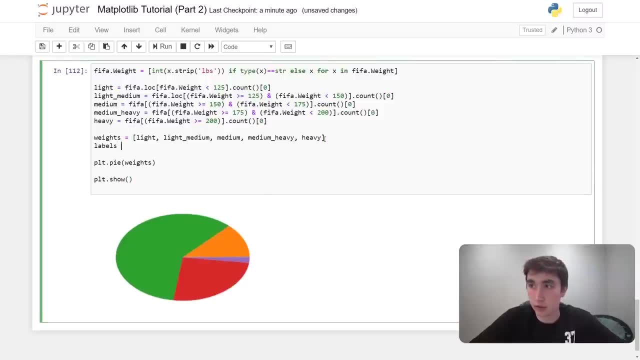 but it has no labels right now and I'm gonna do a plot dot show, so we need to add some labels. so under 125 is the first one, 125 to 150 is the second, 150 to 175 is the third and 175 to 200 is the fourth and finally, over 200 is the last. 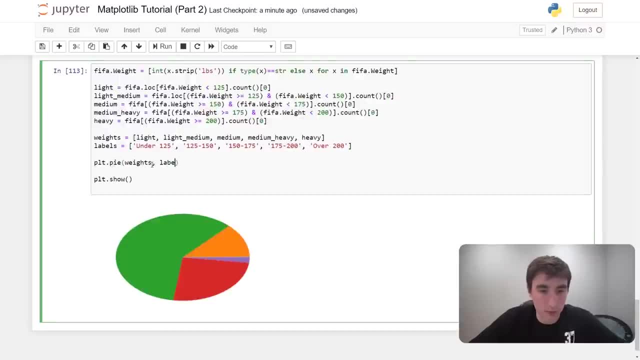 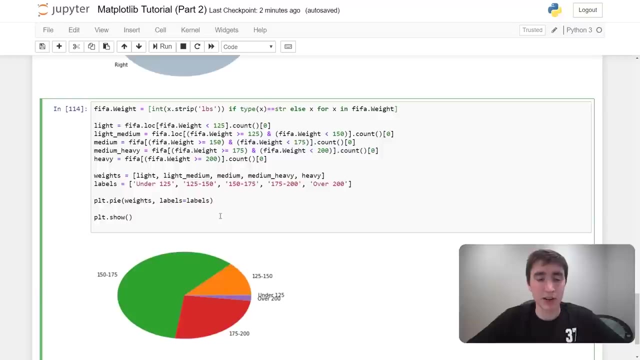 And we'll pass these in with our pipe chart. Okay, cool, So now we have all these labels. One thing I don't like- and this is a good little thing to know- is: you can? I don't like the default color scheme and instead of passing 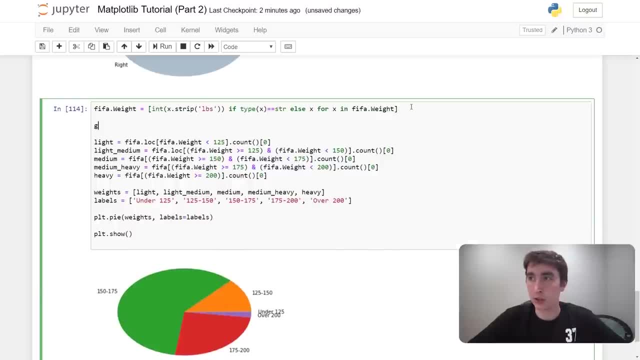 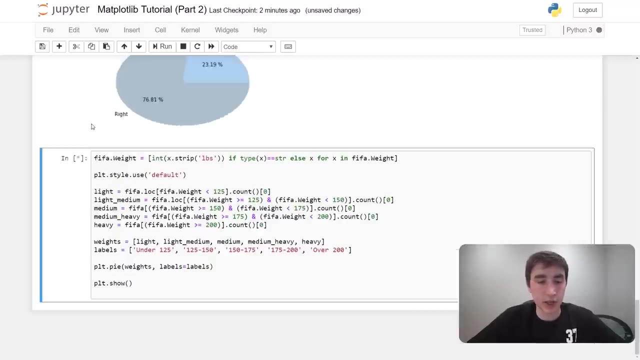 in all five of my own colors. one thing you can actually do is- I don't know what I just typed in. I didn't mean to do that, I'm getting ahead of myself- is? there's a plotstyle and so, instead of the default, which is currently set as you can see, it stays the 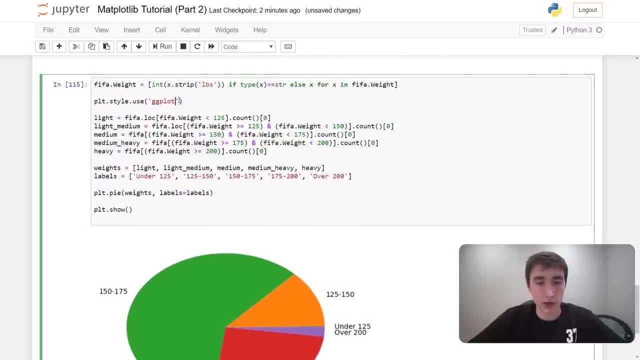 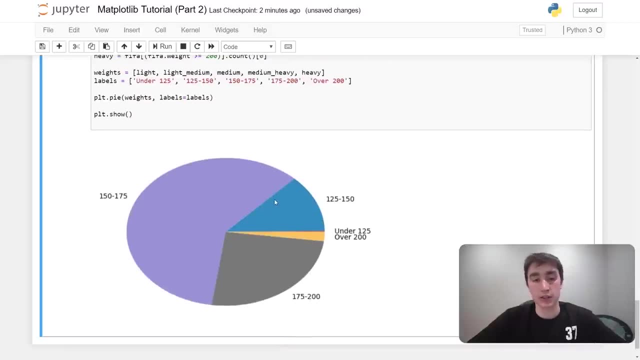 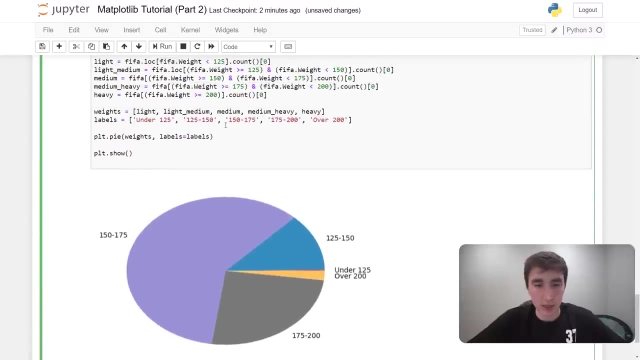 same. when I do that, we're going to use the style of ggplot, and I'll link a list of these different styles in the description. So I personally like this color scheme a lot more when I change the style of our plot. Okay, so that's pretty good. We can also add the auto percentage, as we did. 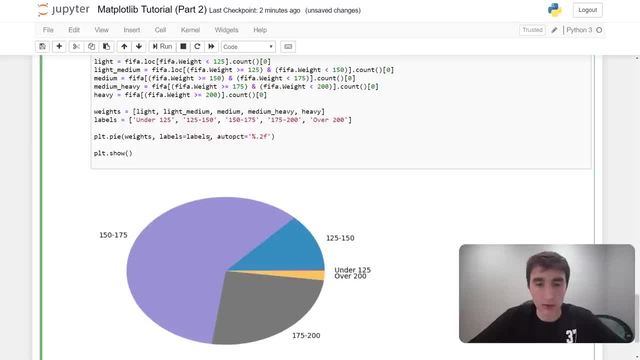 with the last example. So percentage 0.2f, percentage percentage: cool, But things are a little bit ugly in this case, that things are squished together. So how can we resolve this problem? And really, if you go into 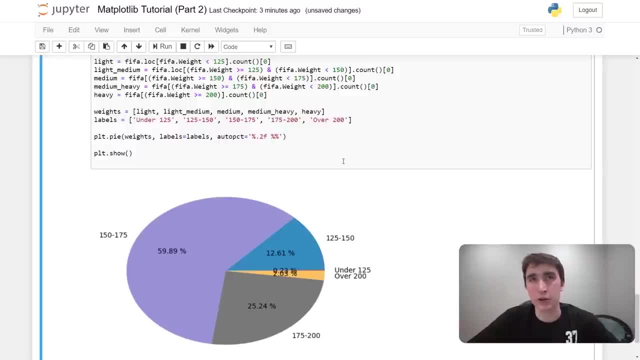 the documentation you'll see there's a lot of these weird names and you might not know what everyone means. But if you kind of look up, like if you did a Google search like pie chart, Python numbers getting in the way of each other, you probably find some different solutions. So one: 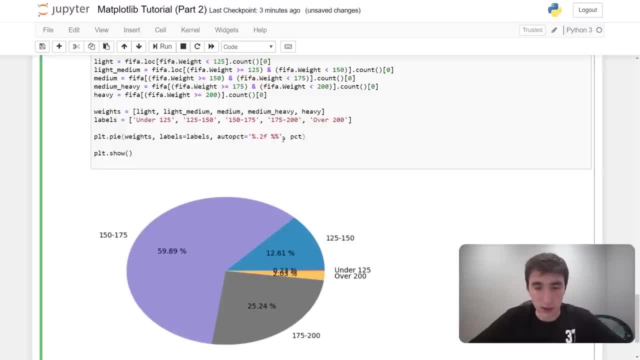 solution we could go ahead and try would be setting the percentage distance. So the percentage distance is the percentage distance from the center of the graph. So if I did percentage equals percentage distance equals zero, you'd see everything's right there. So instead of that, 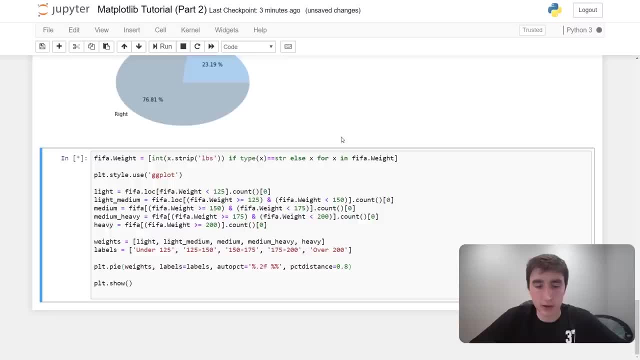 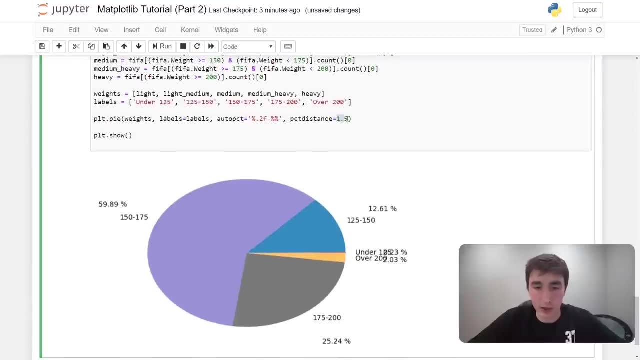 we'll do like 0.8.. So this comes zero to. one is within the chart And you could even, if you wanted to, like 1.5, and that would be values outside the chart, But 0.8 was a good value. 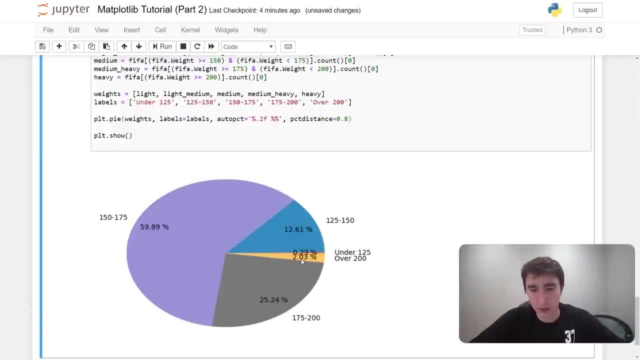 that I thought, Okay, so this maybe makes it a little bit better. These numbers right here that I'm highlighting aren't as squished, but they're still not great. So the other thing we can actually do is use this explode property. And what explode does? it breaks the graph apart a bit, And so 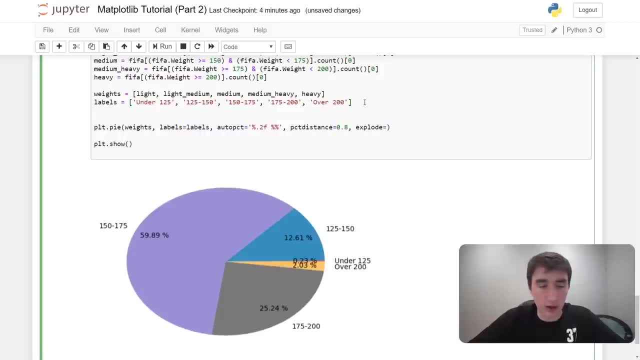 let's see what that does. So we need a list that's as big as our. yeah, this could be a list. it can be a tuple. I'm going to set it as a tuple. That's what I did when I was playing around with this. It doesn't, shouldn't matter. Zero. 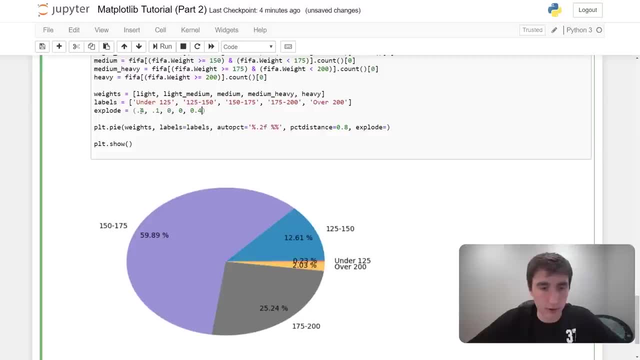 0.4.. I'm going to- these are the values I want to get to, but we'll start with doing them all- 0.1.. And I'll reason to why I got to the values that I got to. Okay, so explode equals explode, So this. 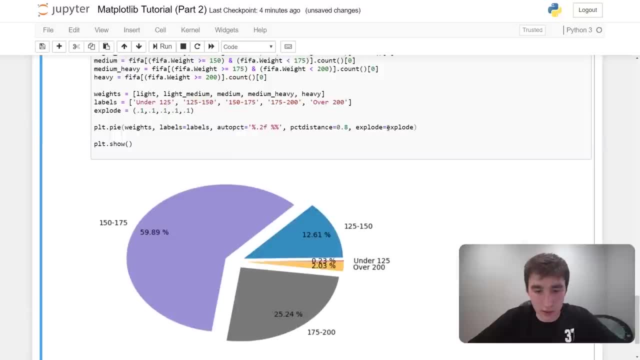 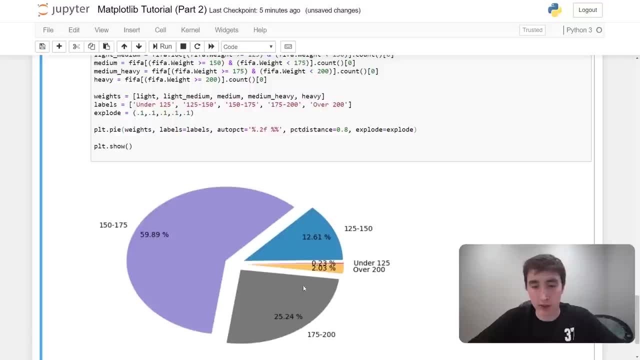 exploded. We really just need these values that are very close together to explode a bit. So what we can do to that is all right. so we want under 125 and over 200 to be exploded a bit more. As you can see, those correspond to our labels here. We don't really need 150 to 175 to explode at all. 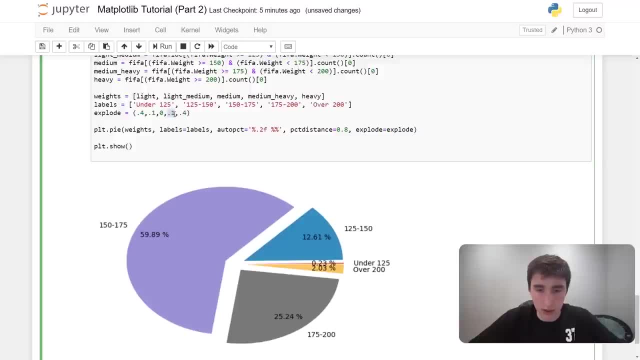 because that's pretty set. We don't really need 175 to 200 explode. So what does this look like now? And we'll have this explode a little bit? This is this 12.61%. Cool, And I think that this looks decently good. now You can more easily see the different. 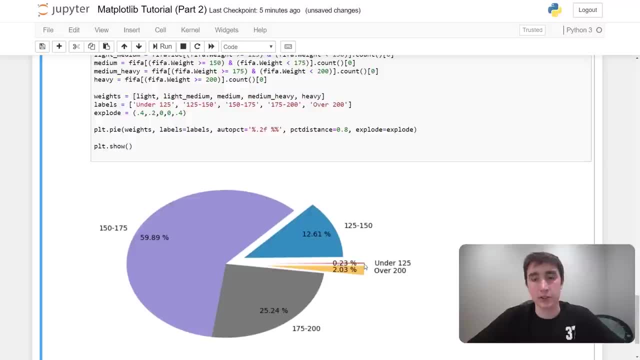 slivers, And I guess it's tough because this sliver is so small- the under 125, but I think that you can more easily read this than you could. So we're going to do that, So we're going to do that, So we're going to do that. 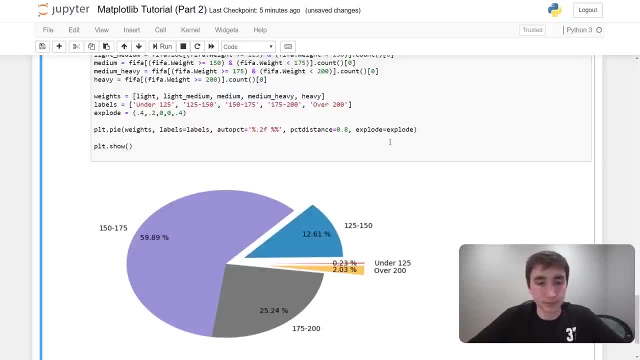 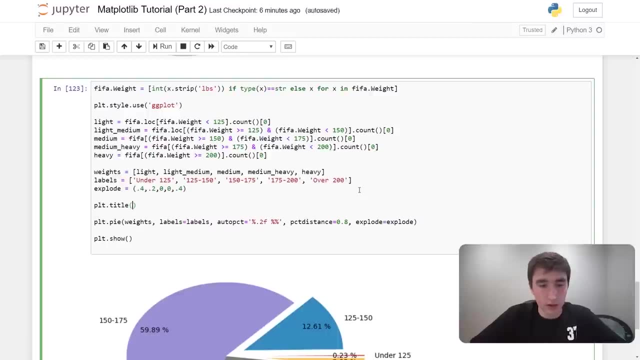 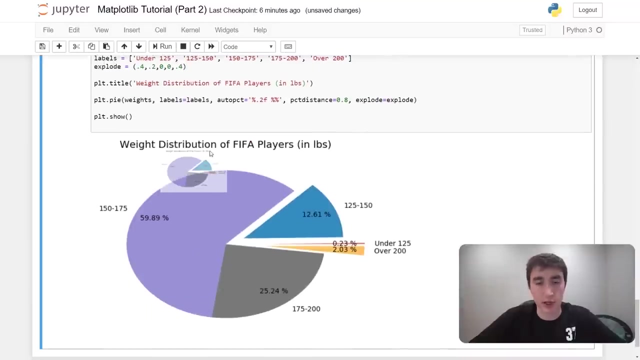 So then we, and, as in the other examples, we can also add a title, So weight distribution of FIFA players, And we would want to say: this is in pounds, Cool, And also, as you notice, because I changed the style, the header actually changed too. So that's one thing. 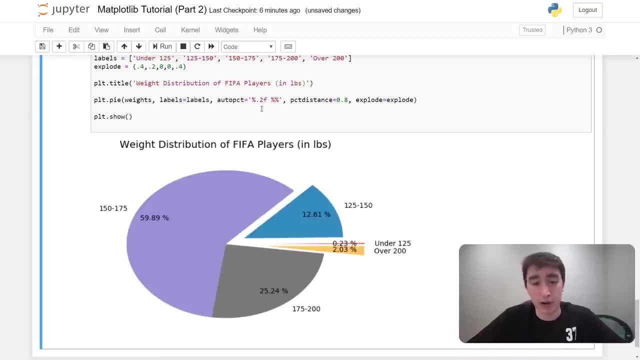 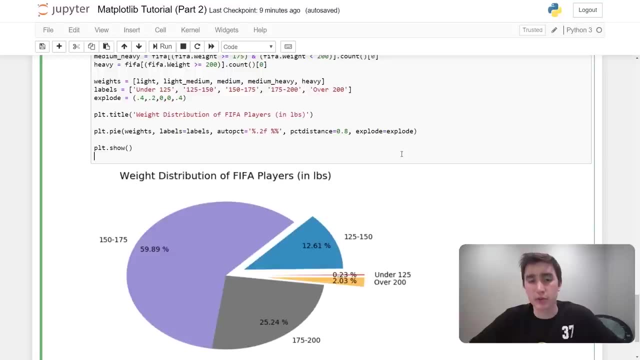 to be a little bit careful with styles, but sometimes they can be very helpful. all right, because this video is getting kind of long, we're going to end it with one more graph, but if there's other types of graphs that i didn't cover in this video or my previous video that you want to see, let me know in the comments. so we're going. 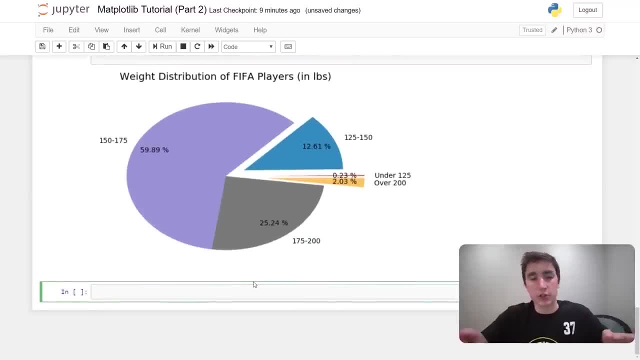 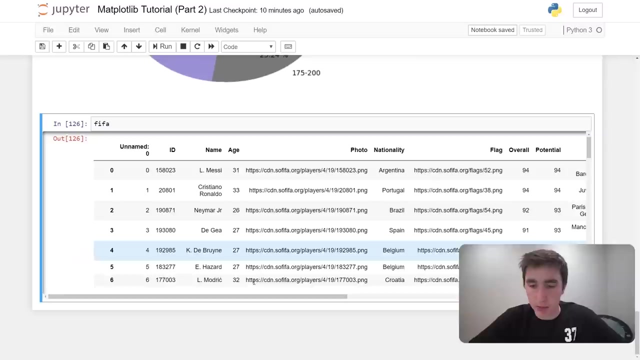 to do a box and whiskers chart and really the question we're trying to ask here is how can we compare teams like the, how good two different teams are in our set? so, looking back at our fifa chart, let's print that out so you can see that all these players have a club. 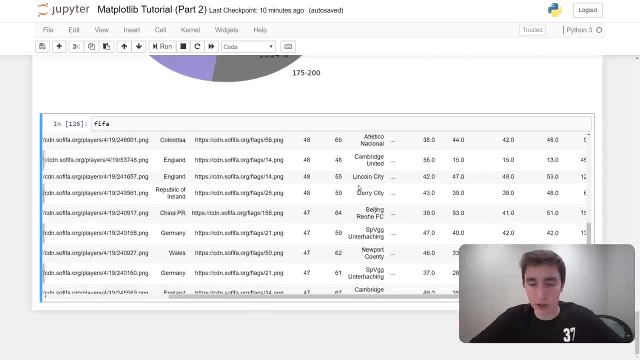 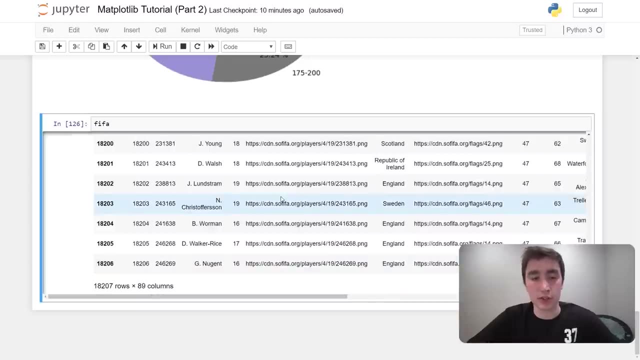 so we're trying to compare the relative strengths of different clubs, and so the i thought that a good way to do that would be this: to use this box and whiskers chart, which shows um shows your highest player or it shows your highest score, if you have a box and 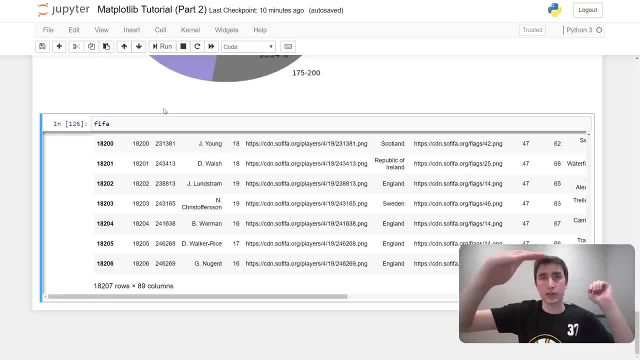 whiskers chart. it will show like the max, it'll show the mean and then it'll show a box around where the middle fifty percent of scores or values were. i think that's a good way to compare a team where you can kind of see, okay, where's the best player at, where's their worst player at, if everyone got injured. 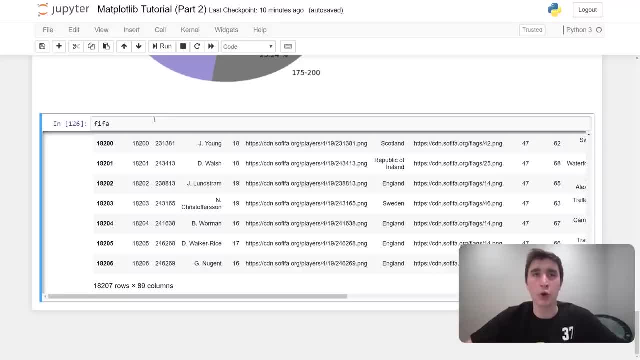 and then the, the middle box is kind of like the core of the team, like how good are they? so i think it's a good way to potentially compare to different teams. maybe you can disagree with me, maybe nào different way you would recommend, but that's what we're going to do in this example. so to start, 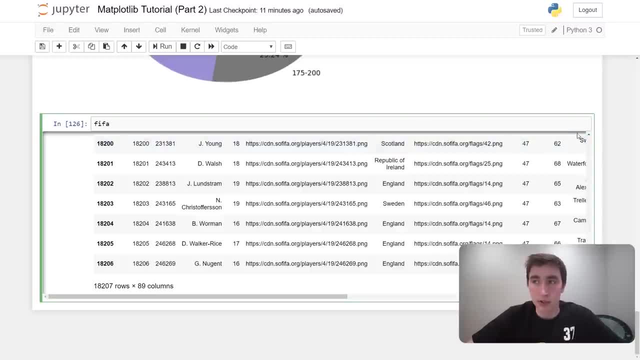 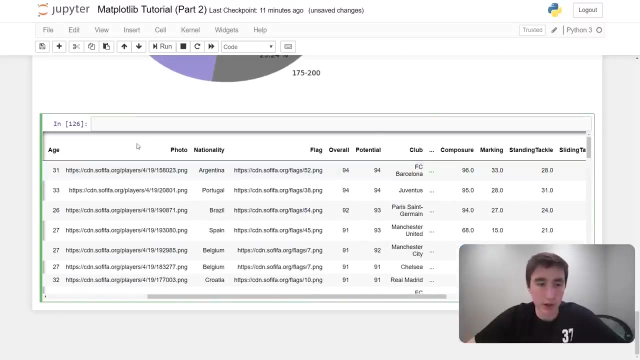 let's uh, take a couple teams and count their um, their overall scores, for that club. so we'll start with what's a good team to start with. go up top. we'll start with fc barcelona, so we're going to do barcelona equals fifaloc, so we're going to filter out all the rows that have people from barcelona. 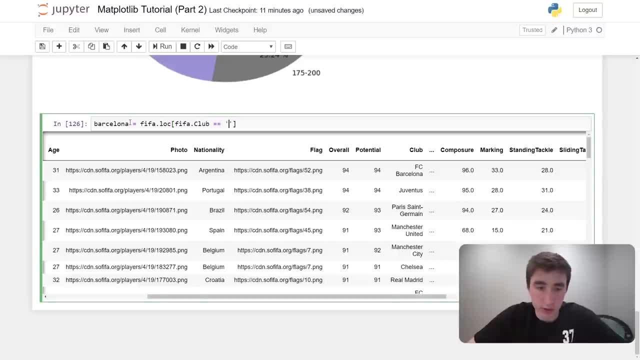 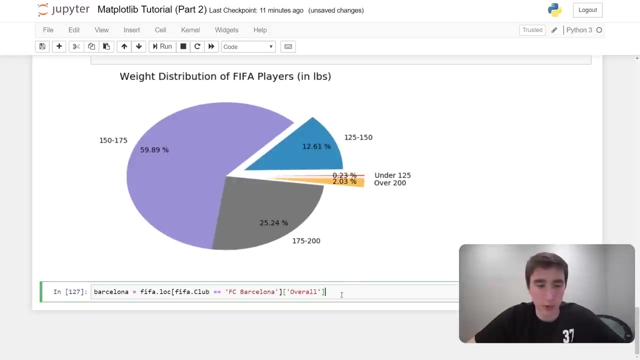 so we can do: fifaclub equals equals fc barcelona- yeah, cool, and let's see. and then we want, when we do our averaging, we're going to want to take their overall score, so we can just filter by that too. so now, if we print out barcelona, 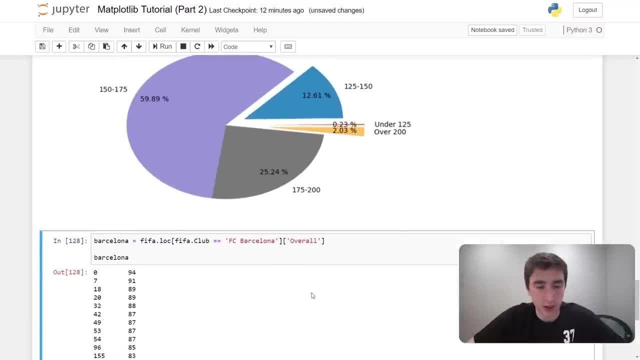 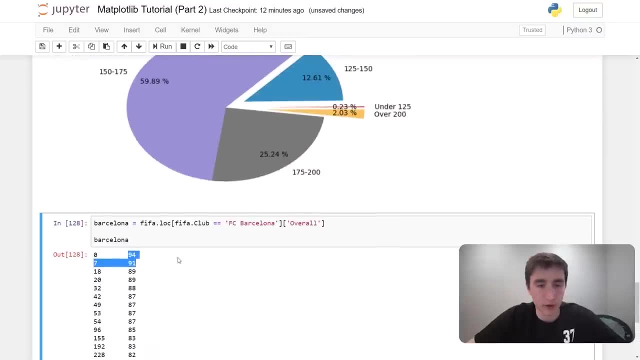 because we're comparing the overall scores. i think that's the most useful metric. you see, we just have a list of all the players on barcelona, their relative, their overall performance in fifa- cool, and we could do that with another team. let's say we do, uh, real madrid. 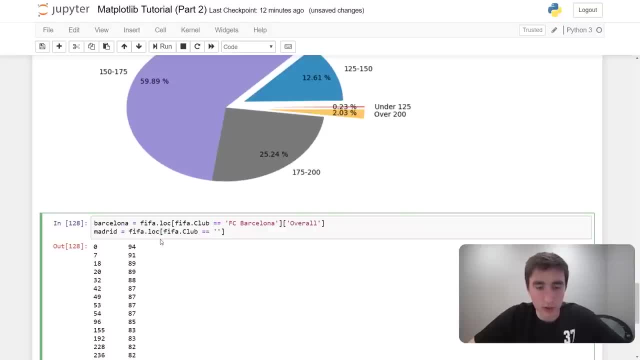 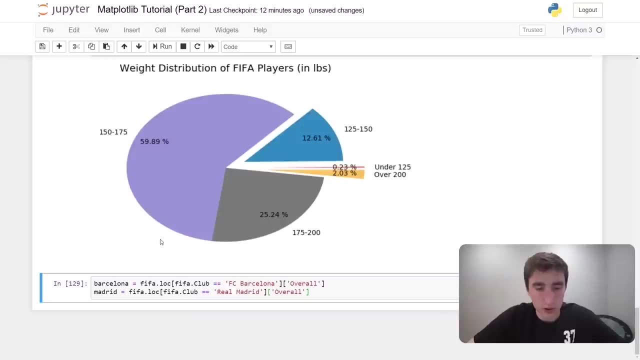 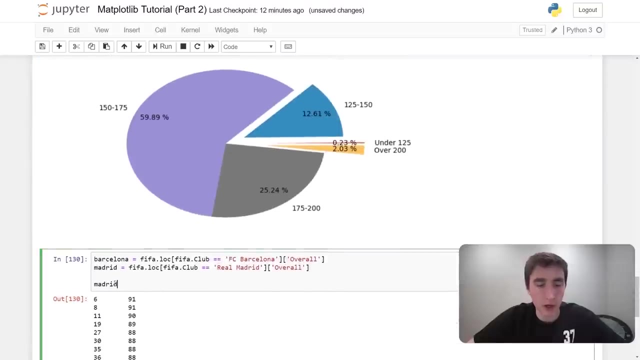 fifa club equals equals real madrid, and we want to take their overall values as well. cool, so this is two different values. we can see madrid here and all those values. okay, so now let's plot a box and whiskers chart for that. so to do that, we do plot dot box plot. we pass in barcelona and we'll pass in madrid. so these are the. 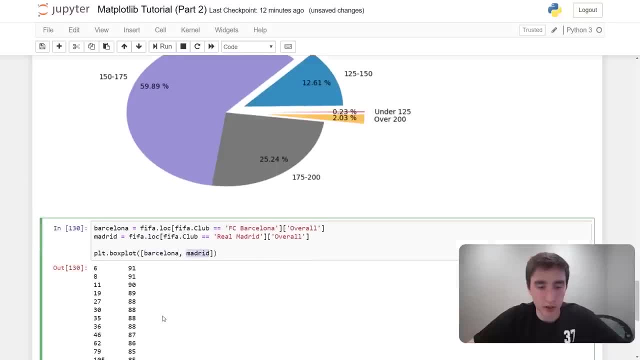 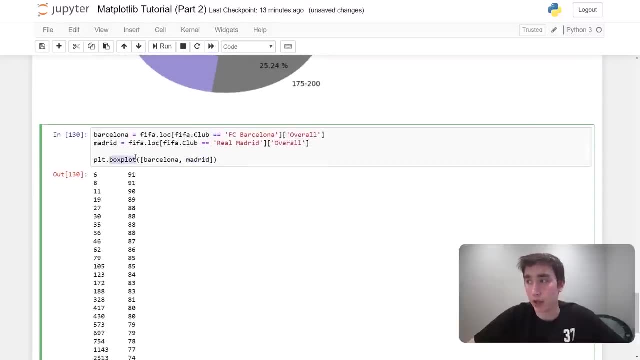 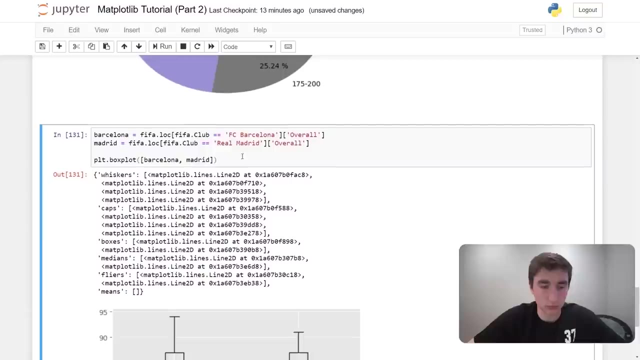 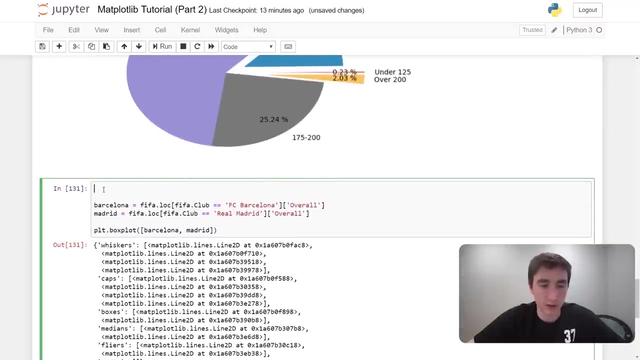 all the values for barcelona and all the values for madrid and corresponds to what we see here. so it will know this function will know that it needs to make a box plot off of that. so what does that look like? okay, one thing i noticed too: this is also a residual effect of changing the style in one cell. 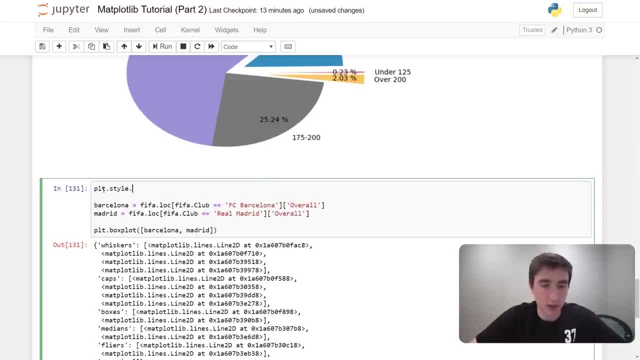 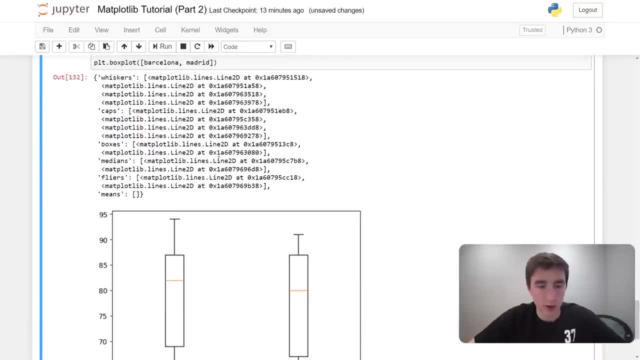 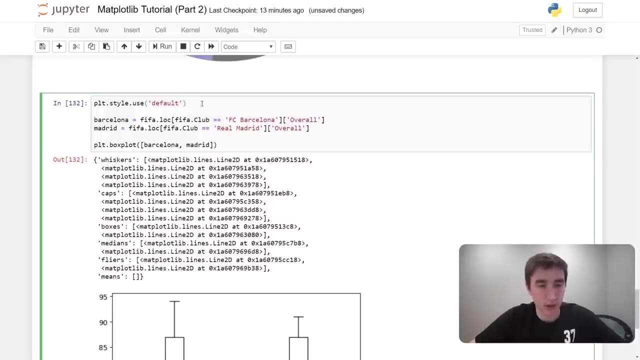 style is still changed. i'm going to change the style here back to our default style. so default style looks like: this graph doesn't really tell us too much right now, but we'll get it to look a little better in a second. um, and i want to do plot dot show. so all this. 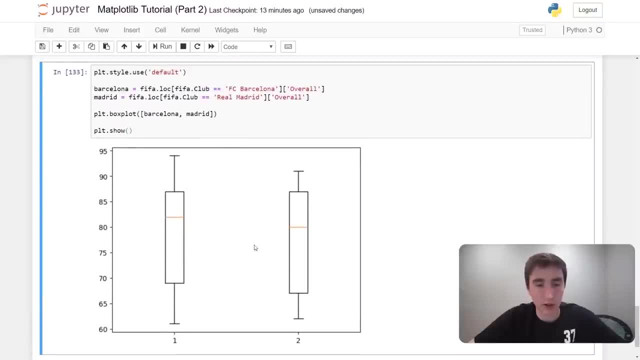 stuff is not there, okay, cool. so this is a comparison of the two teams. relatively, you can see they're pretty dang. even i'd say barcelona has a slight advantage here in this box is a little bit higher than real madrid's, but, and also their best player is ranked better than. 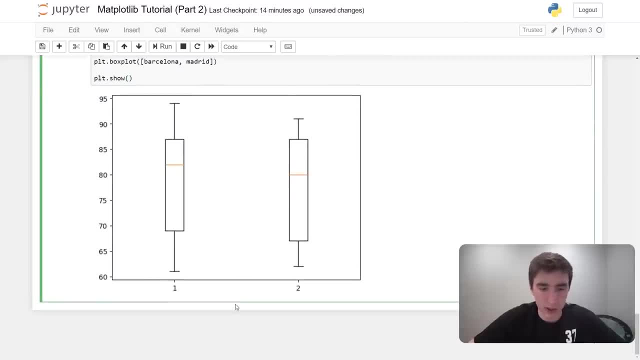 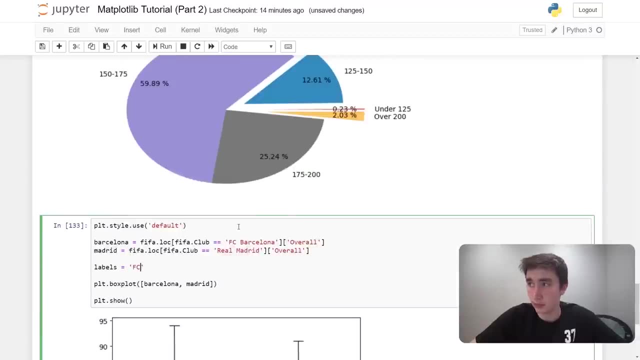 real madrid's best player, but it's kind of annoying when it just says one and two down here. so let's add our labels. so it's a list: fc barcelona and real madrid. so the first thing we're going to do is we're going to put in our box plot. it has a labels. 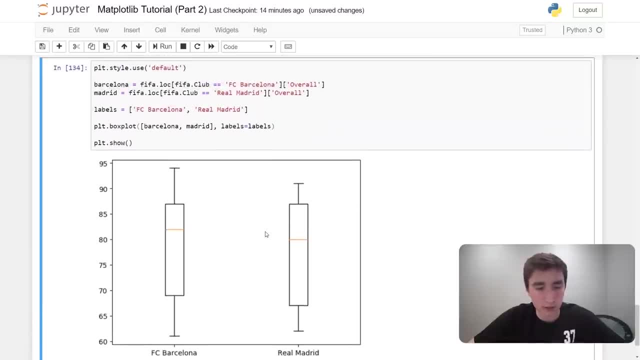 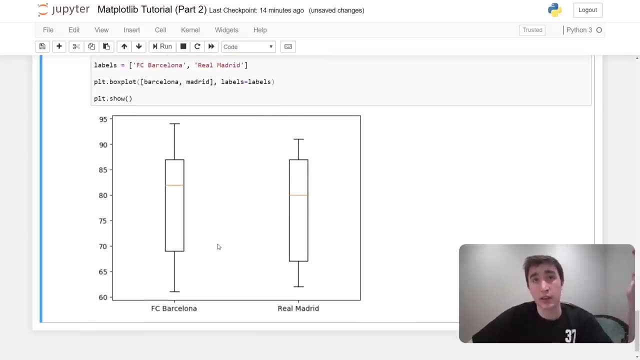 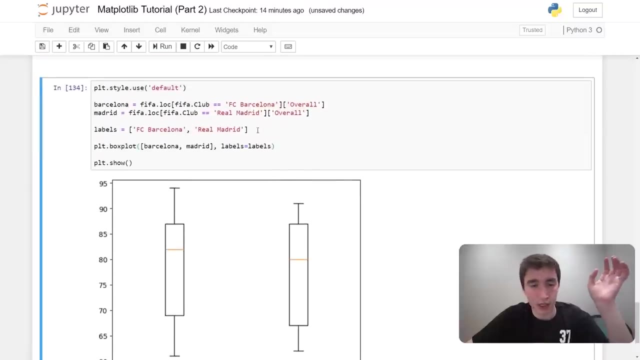 property and you can double check the documentation to see this. labels- labels, cool. so now we have our two different box plots, and so these two teams- with this comparison, i would just say that they look pretty similarly matched, like they could go head to head probably be a pretty good game. 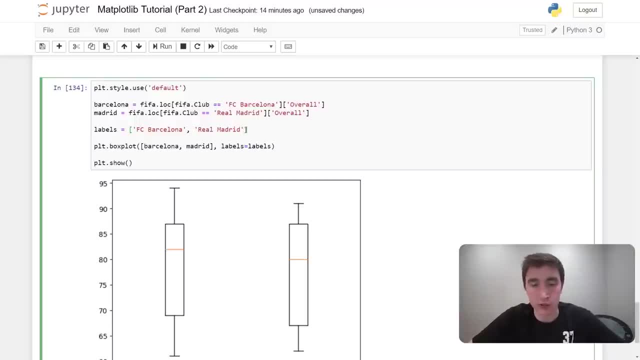 where you really see kind of the coolness of visualizing this data, you take a team that's not as strong. so my local team here in boston is the new england revolution. they're an mls soccer organization so i also pass in some scores for them and their short. 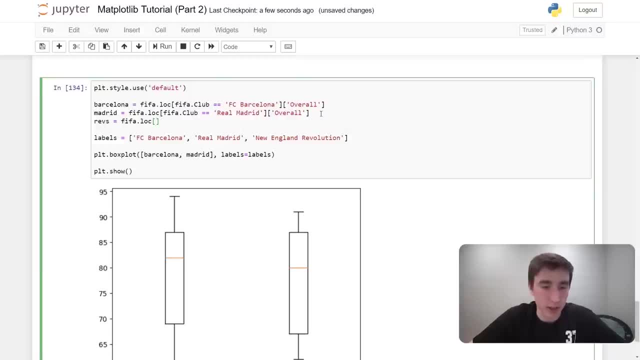 tinned name is the revs, so i'm going to just call them that instead of typing out the whole new england revolution, revolution every time and uh, yeah, what am i trying to say? new england revolution and we want to take their overall. and you could look at all the different teams in the data sheet. 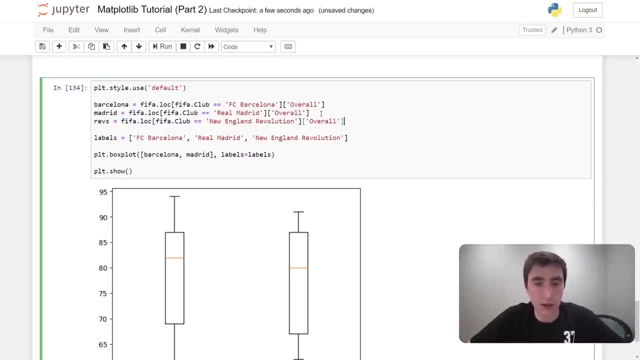 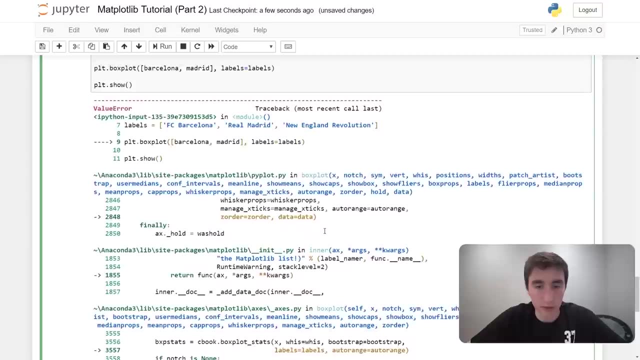 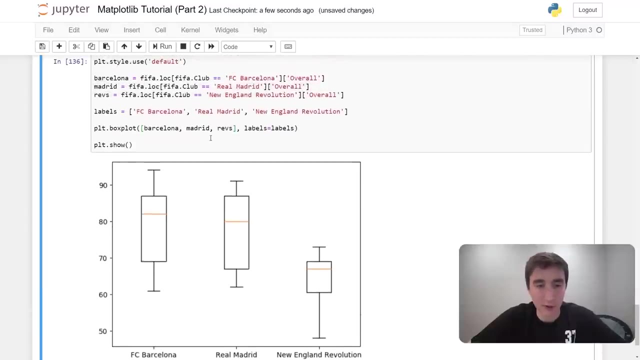 and get like a certain team that you wanted to look at. pretty easy, you just have to be careful that you type in everything properly, and apparently i did something wrong. oh okay, yeah, we also want to pass in the revs here, cool, so now we have three teams and you can see that. 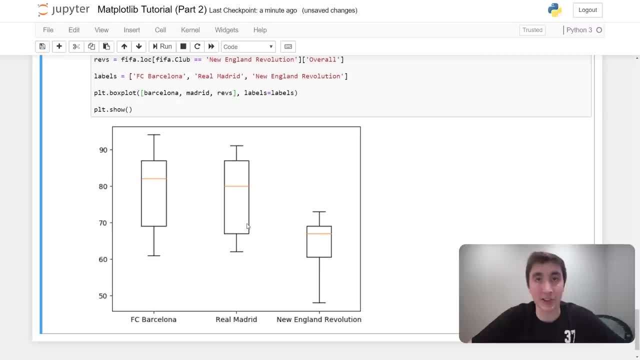 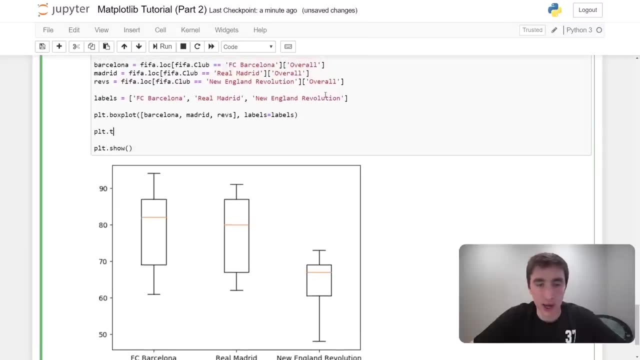 the new england revolution is significantly worse than real madrid or barcelona, which is what we are wanting to show. um, let's add a title here and we'll add some style to this chart as well. professional soccer team comparison- and because i'm from the states, i call it soccer. yeah, you probably call it. 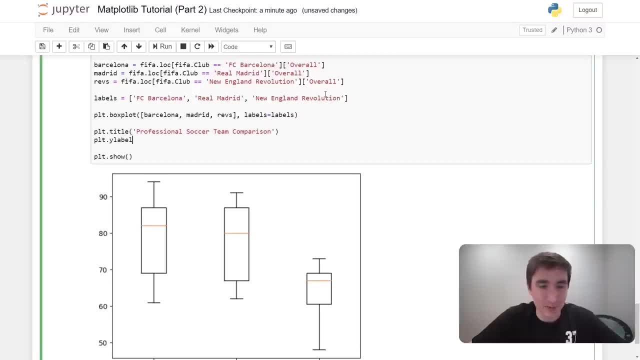 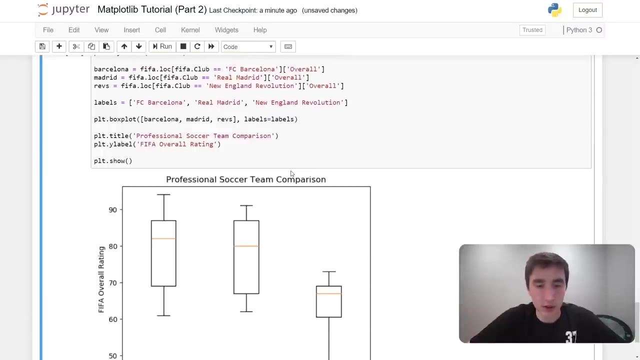 football, but that is besides the point. fifa overall rating, overall reading, is our y-axis and we have our teams down here in the x-axis. that looks pretty good to me, okay. what we could also change up potentially would be: um, our tick mark, um, uh, okay. or we could change the figure size. maybe it would look better if it stretched out a. 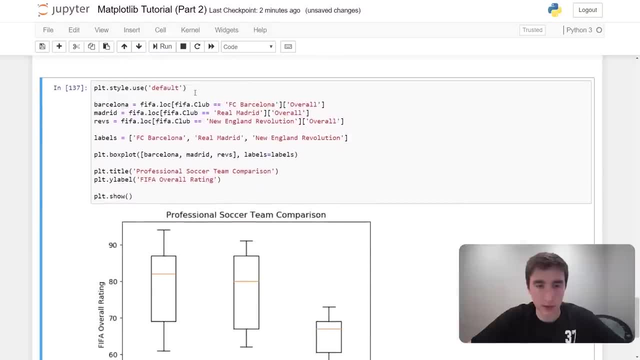 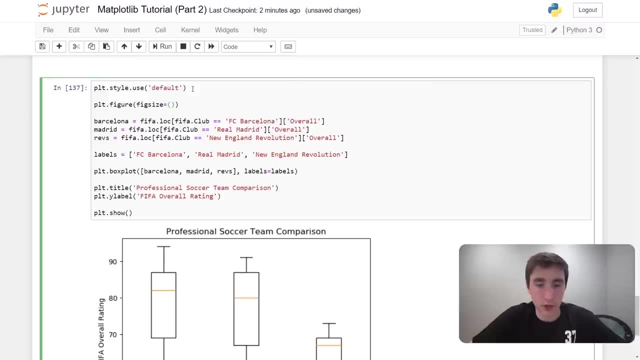 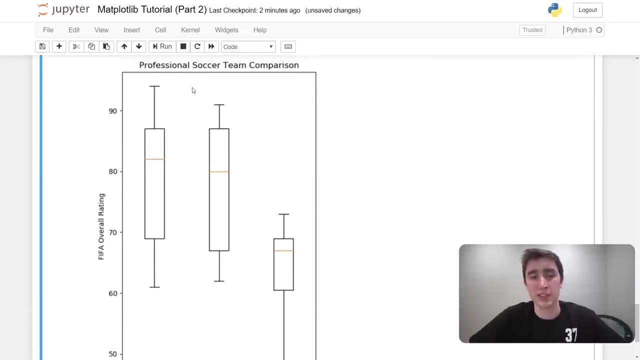 bit more along the y-axis. so we'll change our figure size a bit. so plot dot figure fig size equals. we'll have the y dimension be greater than the x and as you can see now it looks like this and this gives us a little bit more detail in. 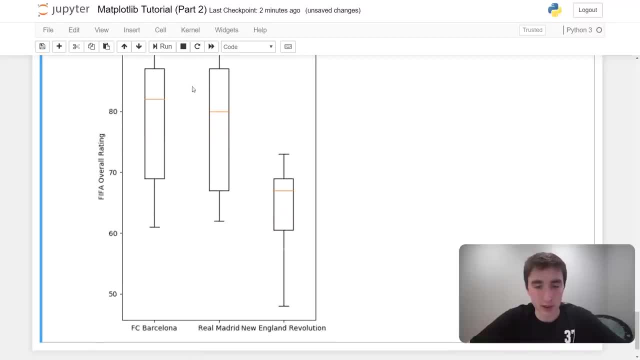 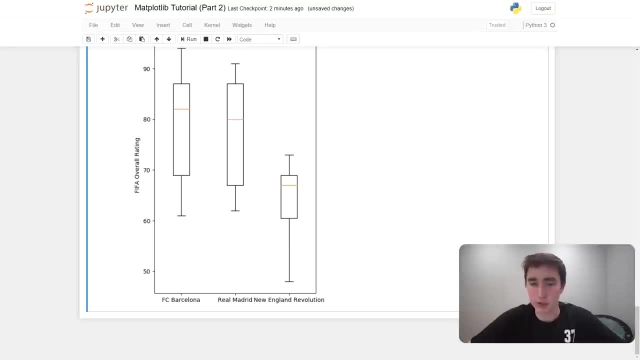 the actual scores among the two teams. but yeah, you can still see the new england revolution is not as good and also this name is kind of running into each other, so i'm going to shorten new england revolution to any revolution, to just kind of make it a little neater, cool, all right. so 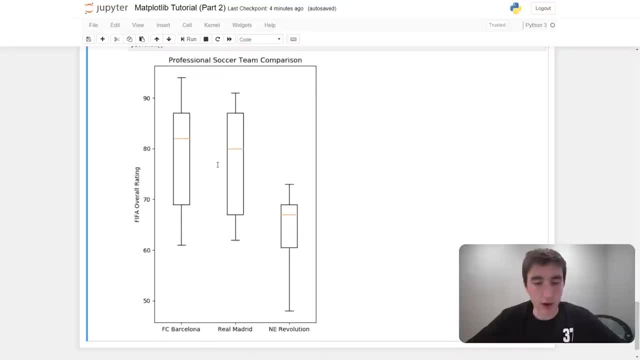 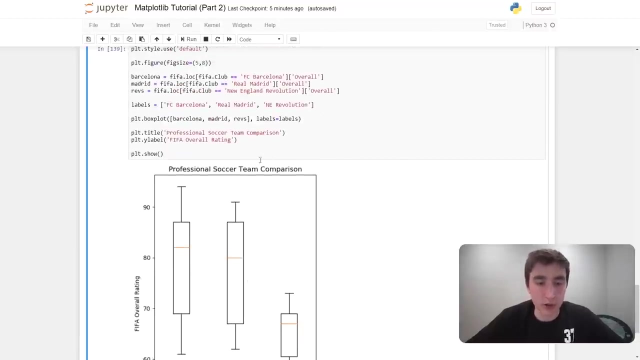 the final thing we're going to do is add a little bit of style to this graph so it looks a little bit better, and you also, if you wanted to, yeah, feel free to add more teams to this and like, really see the differences between soccer teams and fifa. but we will add some color around the perimeters of. 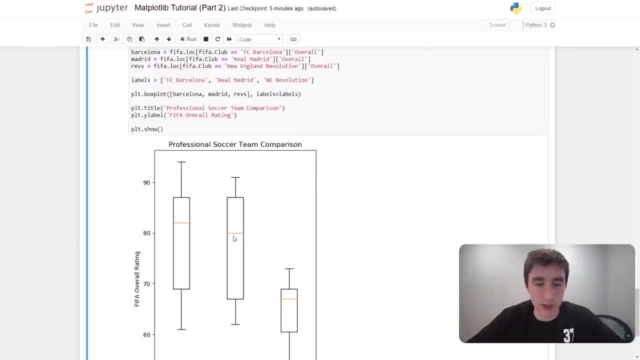 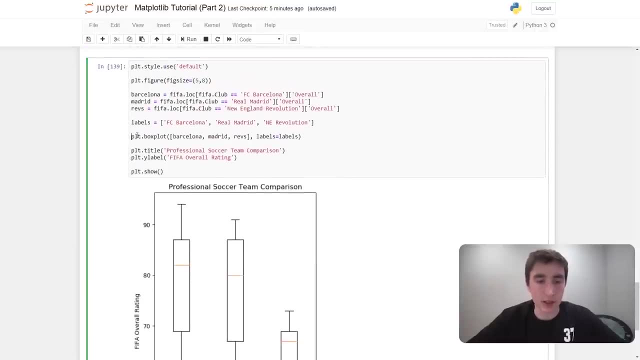 these boxes, maybe make this line a little thicker. that represents this, represents the medium, the orange line, okay, so what i found to be the best way to do this is: i'm going to save boxes as the result of this plot and then, basically, what we can do is this will store the three different values. 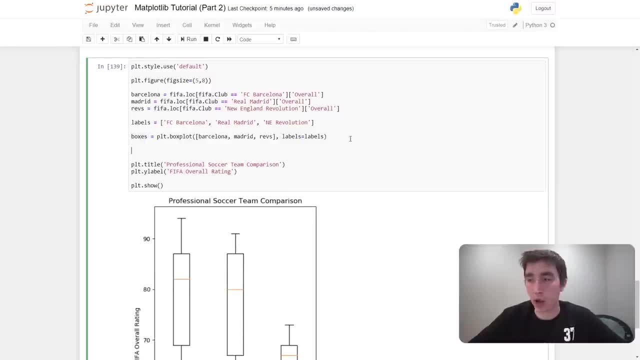 we plotted here, so it'll help us style each individual box a little easier. so for box in boxes, boxes- so you're getting the box parameter from what was saved here. we want to set the color and this also kind of shows you that there's different ways to do. 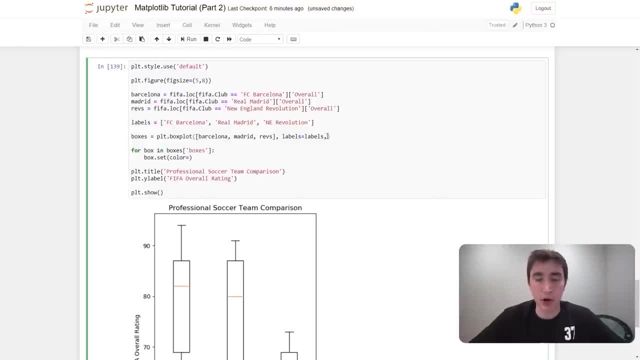 these things like i could have passed color in here. the problem with passing color within here is it would make everything the same color. so if you wanted to like, go ahead and change a specific box, like, and have a list of colors. it's easier, or i guess maybe color is not the best. 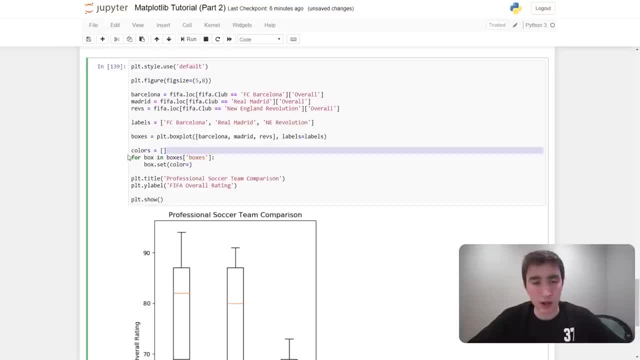 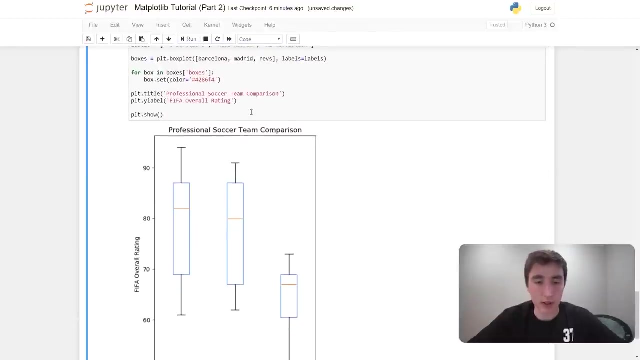 example, because colors probably would allow you to pass an array, but for certain properties it's hard to set just one value at a time, so i'm going to go ahead and set the color here. so now you see that we have a different color around our box and they're similar to boxes here. 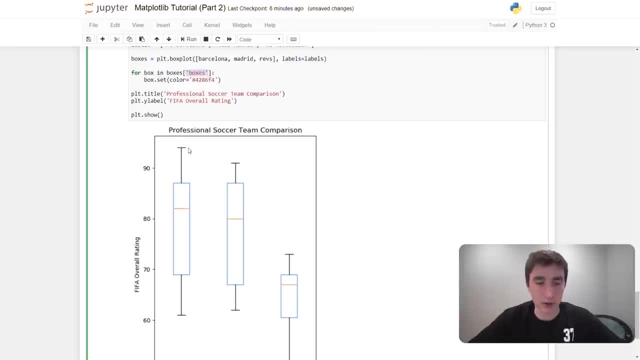 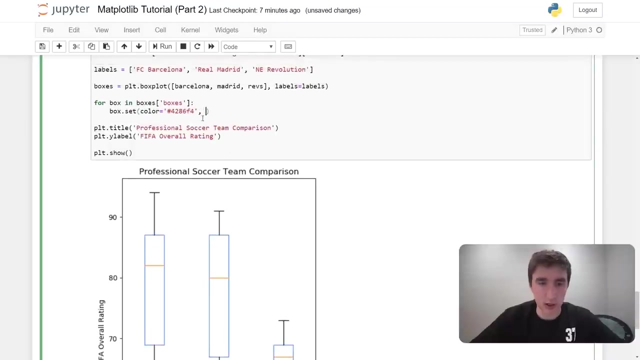 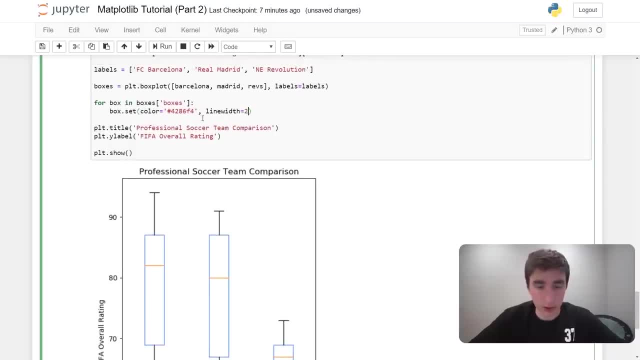 here and then we can do: line width equals two and all these parameters i'm finding from the, from the documentation. okay, cool, so set edge color, basically, and let's say we wanted to change the fill color, so change fill color, and you could, as i said before, like you could, iterate through these and 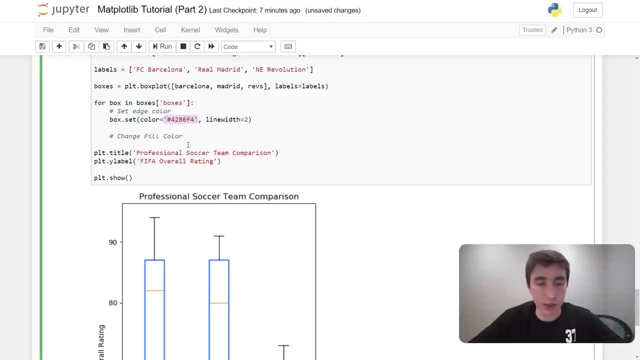 through a list and, like each time, set a different color for each of these change, fill the color. we could do something like set face color. we could all do this in one line as well, but kind of just showing different ways you can go about things. face color is another property. this 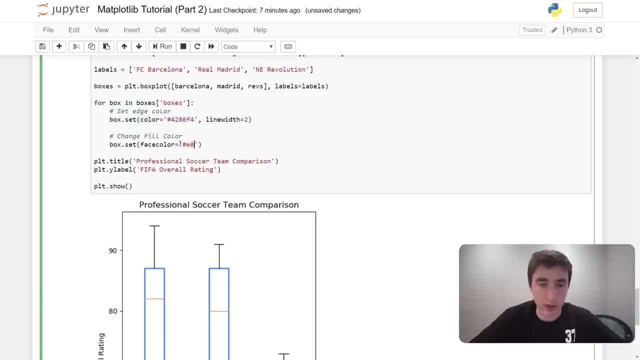 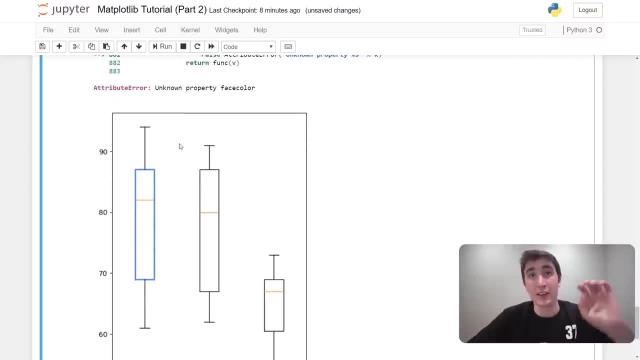 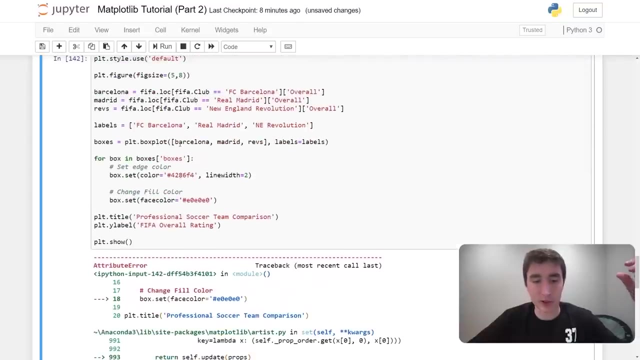 actually changes the inside of the box. so what happens when i do e0, e0, e0- this is a grayish color, unknown property face color. this was something that i found super annoying when i was trying to do this. um, so if you're trying to set the face color of our box and whisker chart doesn't recognize, 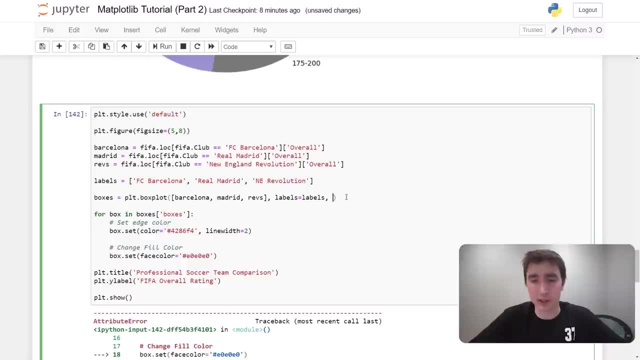 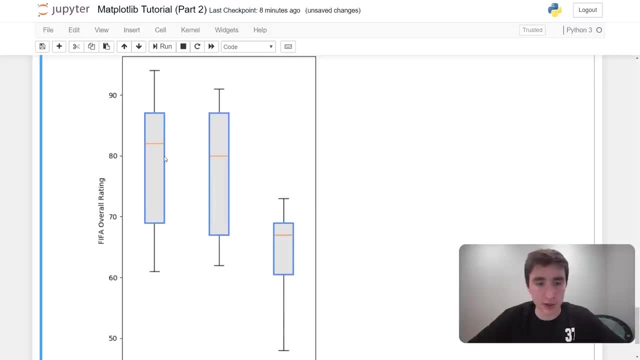 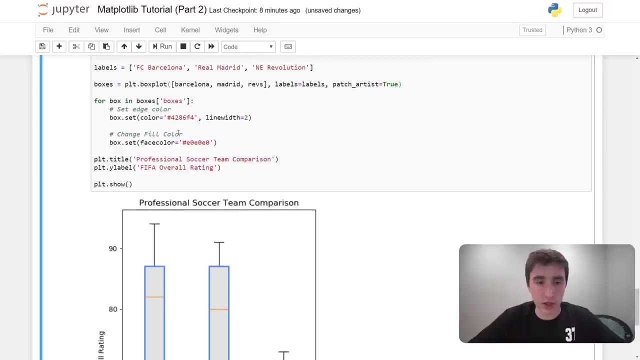 you can't like recognize this property face color, for whatever reason, by default, so you actually have to set this patch artist property to true to allow you to change the face color. so now we have these graphs, i think that looks a bit better. um, we could also change up the median line so you could do it within this format or another. 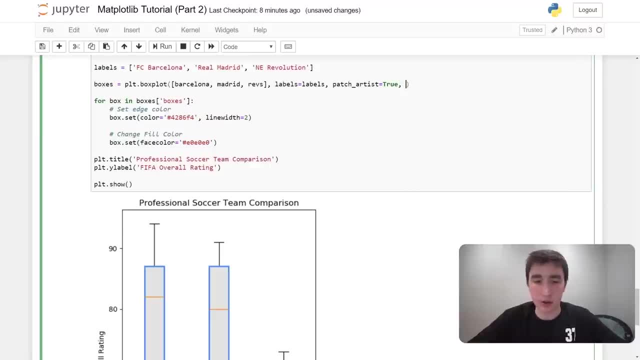 way we can do. it is, one of the properties of boxplot is median props, so you could also pass in like a dictionary of median props, and so we could pass in a line with here too. so let's say, we wanted this line to have the same thickness as um the outline. pass that in and there we go. 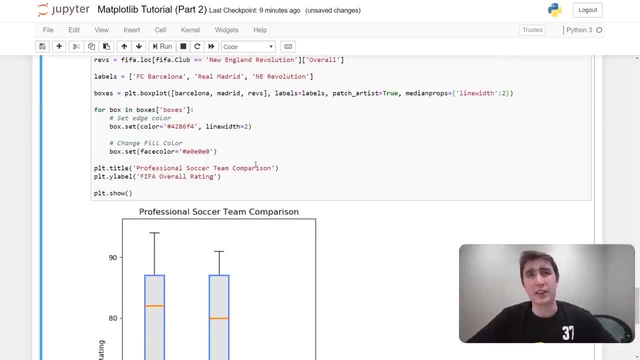 a lot of the styling stuff. it's really a matter of uh, google searching really like you can look at the documentation, find some things from the documentation, but what i find is sometimes quicker is to say: oh, how do i change the outline color in a box and whiskers chart?